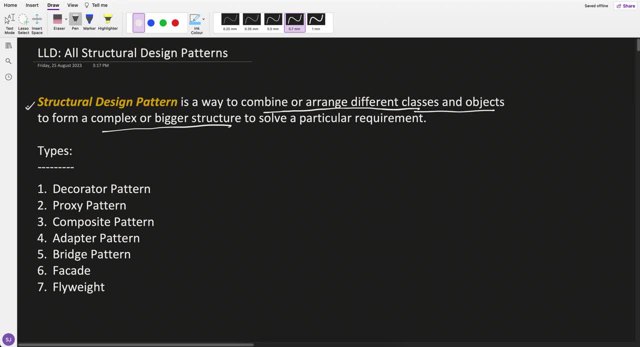 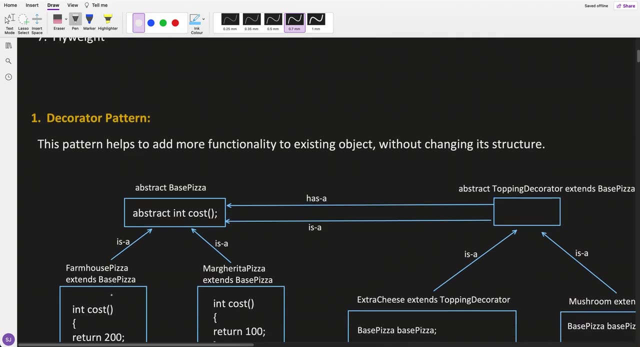 Okay, Okay, So that is what is known as structural design pattern. So there are seven different types of structural pattern: Decorator, proxy, composite, adapter, bridge, facade and flyweight. So let's check each one of them. First is decorator pattern. 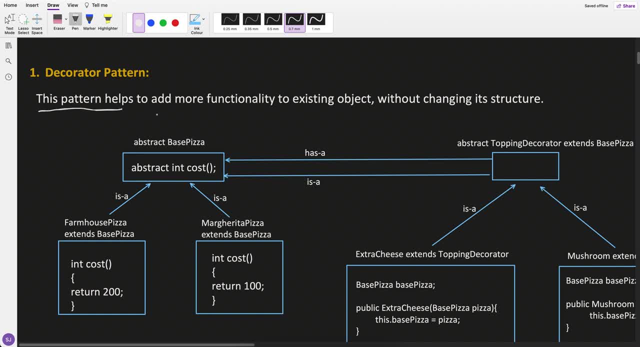 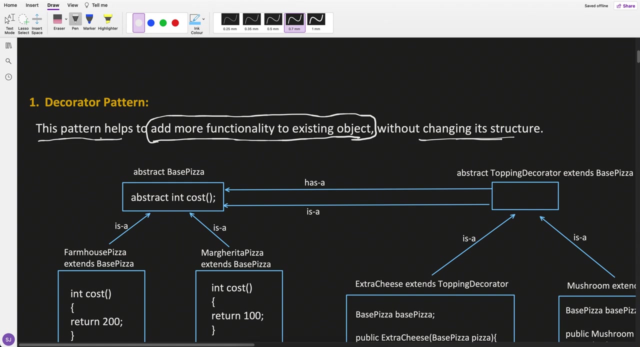 So this pattern helps to add more functionality to existing object without changing its structure. Okay, So just concentrate more on this: to add more functionality to existing object Without changing its structure. Okay, So I have defined, I have explained this decorator pattern with an example of pizza, if you remember. 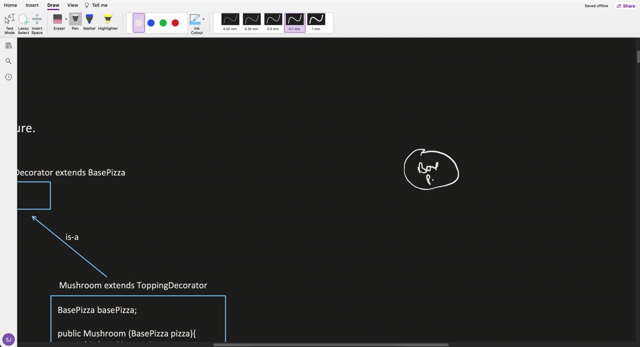 Right. So let's say we have base pizza Like base pizza. let's say it's veg delight, Okay, Now you can garnish it with extra cheese, Right? So what it is saying that add more functionality to existing object. So I am adding more features to an existing object. 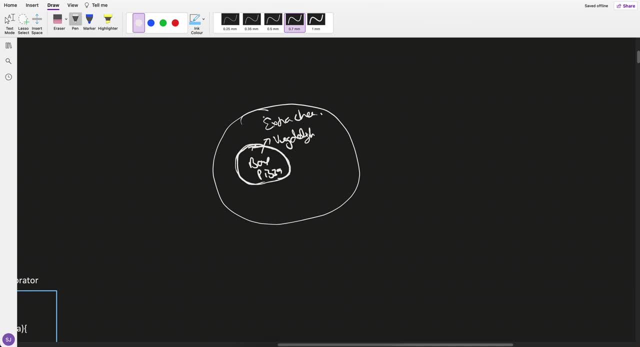 So base pizza is my existing object. I am adding more features, Extra cheese, Add mushroom. Now I can add more cheese. Now I can add more mushroom, More mushroom or some other veggies, Right? So I keep on adding extra features on the very base object itself. 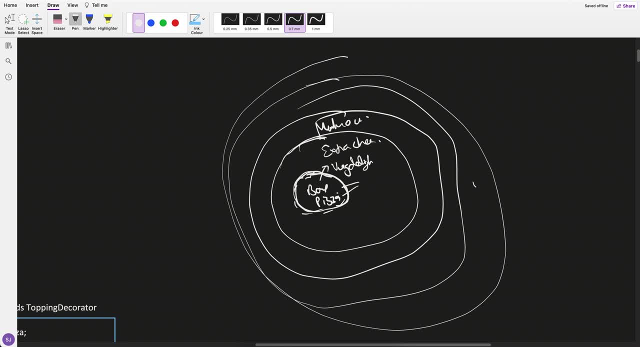 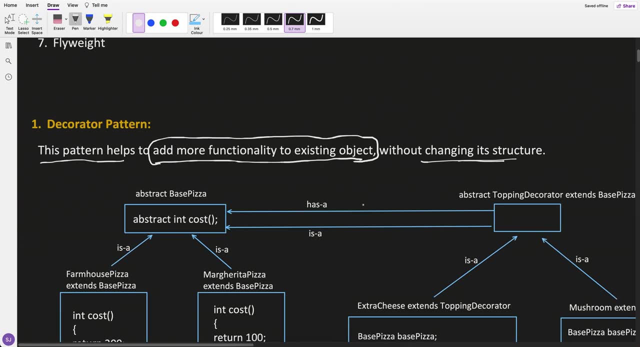 Okay. So if you see that I am not even changing the base pizza, which is of my base object, But I keep on adding more, more layers of the feature. That's what decorator pattern says that Add more functionality to existing object without changing its structure. 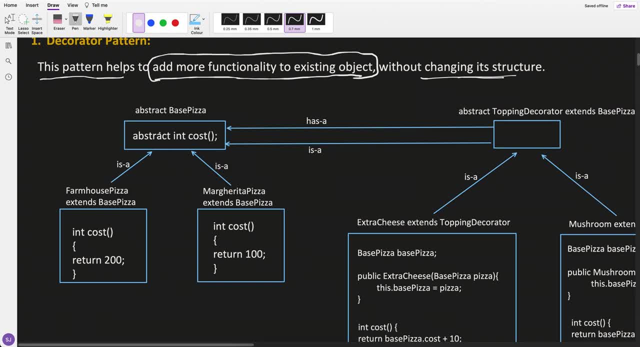 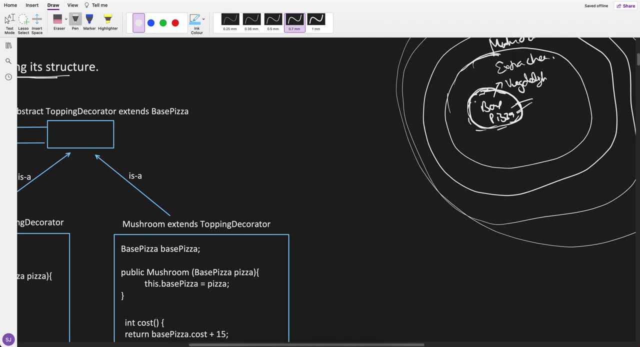 So how we gonna do that? Just see this example. So here I have created an abstract base pizza, Right? So there in the, this is my base pizza. So I have created this, an abstract class, So there can be different type of base pizza. 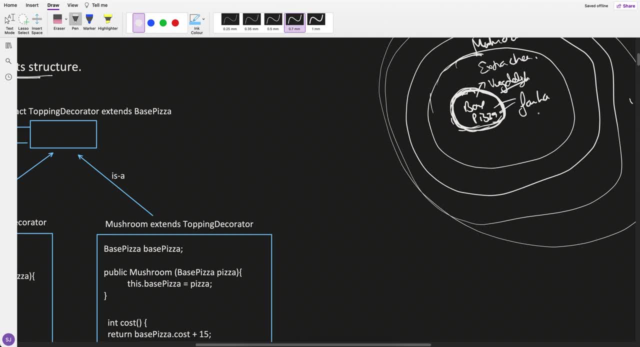 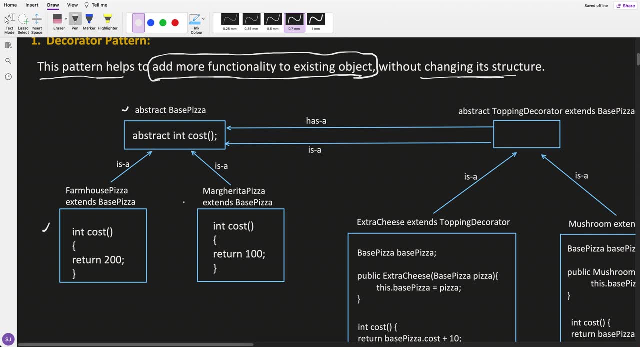 So veg delight is one, Let's say, farmhouse Margarita. So there are different type of base pizza, So I have taken created two classes, Two concrete classes of this base pizza. One is farmhouse, Which extend this base pizza, And one is margarita pizza. 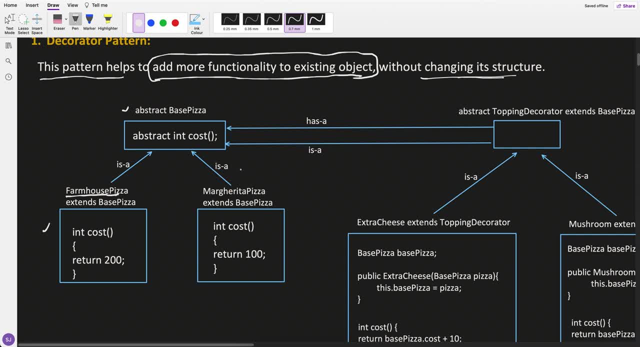 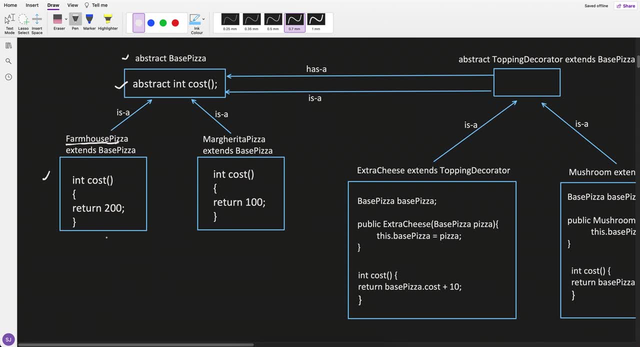 Which extend this base pizza. So it's a isza. Okay, So it has one abstract method Cost And this farmhouse is implementing that abstract method And it is, let's say it is, of 200 rupees. Margarita is 100 rupees. 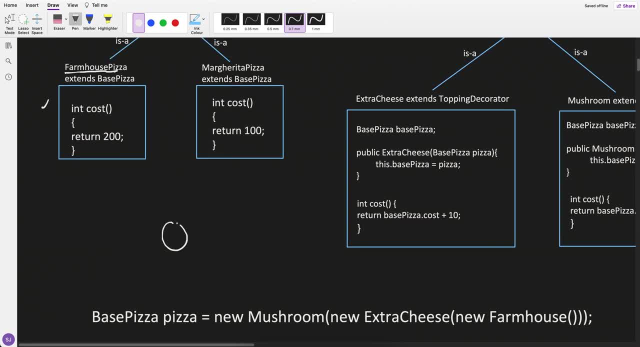 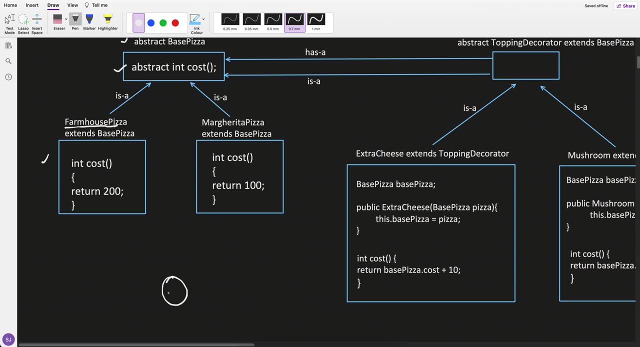 So this is very, very base object. Okay, Now I want to add additional feature, Right? So once I have created, let's say, Farmhouse, Now I want to add additional feature to it, Like add more extra cheese Or add mushroom. 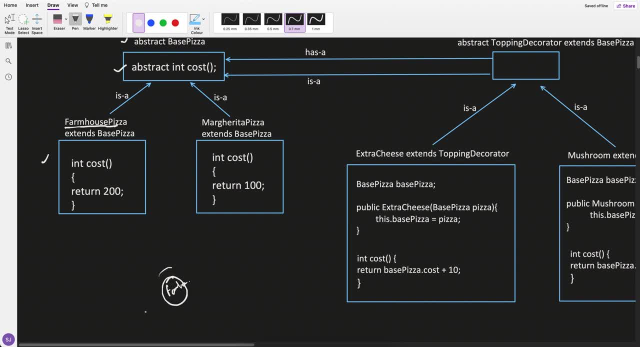 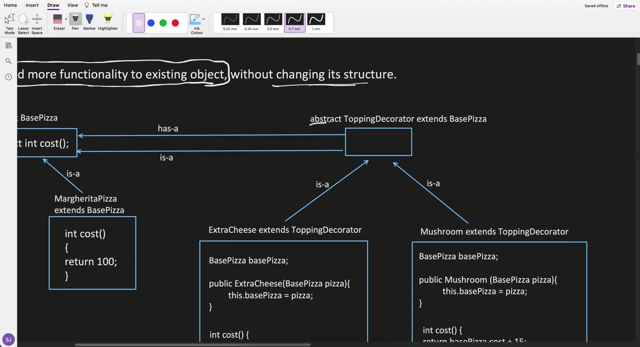 Or there can be multiple combinations, Right, So that's where the decorator pattern is used. So what I have done is I have created an abstract class With the name topping decorator, Right. And if you see this, Notice one point. 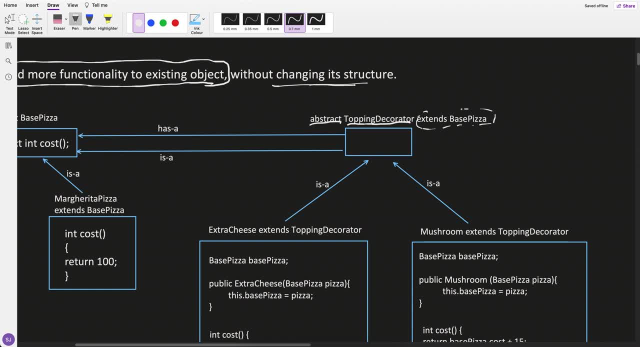 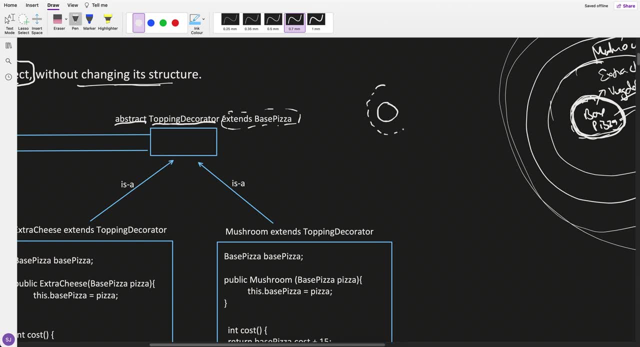 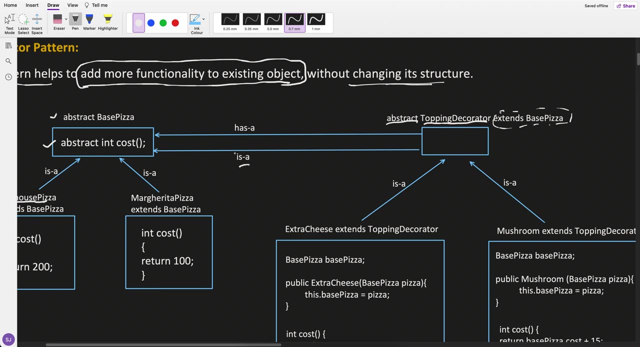 It is also extra cheese Which is extending the base pizza. Okay, So, whatever the base pizza is And whatever the topping decorator you are creating On top of it, So that itself is a pizza, So that also is a, That's also is a pizza. 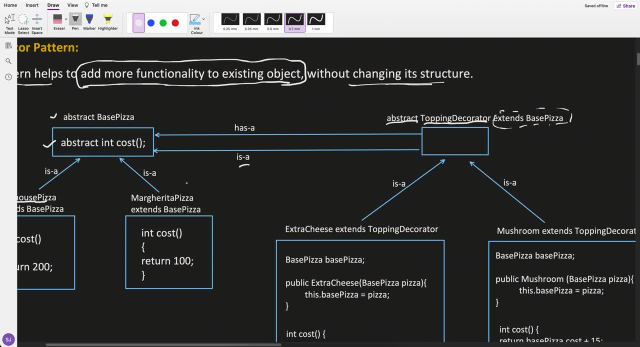 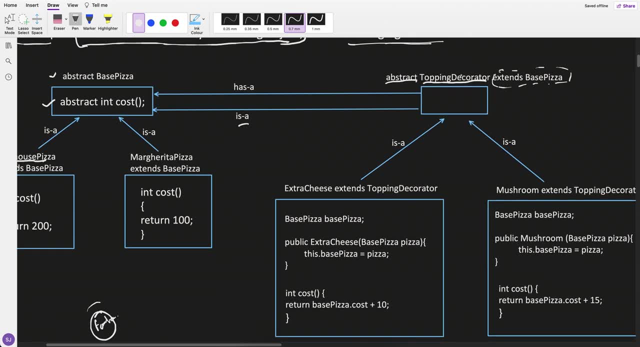 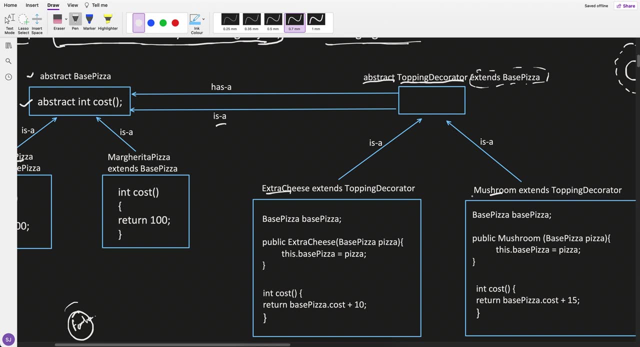 So, whatever the topping decorator you gonna do, It is also is a pizza itself. Okay, And I have, So it has two childs. I have created two type of topping decorator: One is extra cheese And one is mushroom. Right, So they are extending the topping decorator. 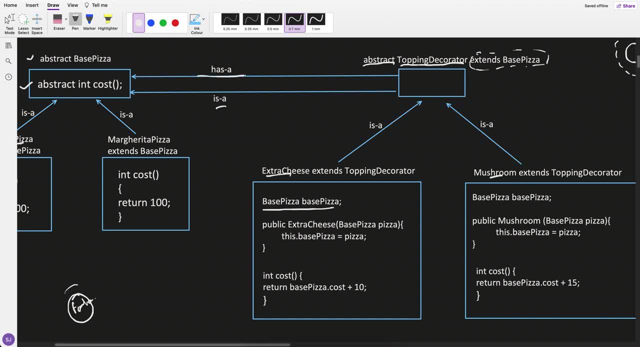 And inside this I have the base pizza, So that's why I kept has a. It has, So it has both. the relation Is a And has a, So this topping decorator is a base pizza And this also has a reference to the base pizza. 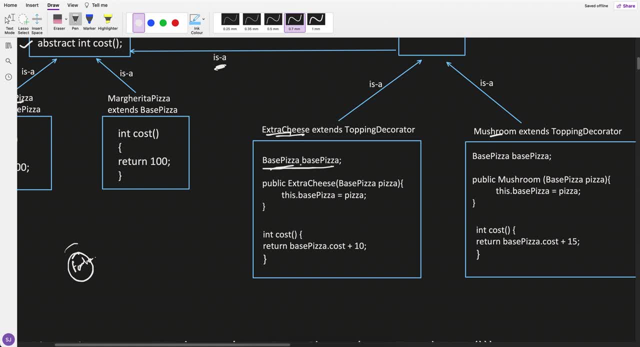 So now in the extra cheese, What I am doing is I have a base pizza reference Right And I use the constructor to initialise the base pizza Right, So it can be either margarita, or either it can be farmhouse. Whatever it would be. 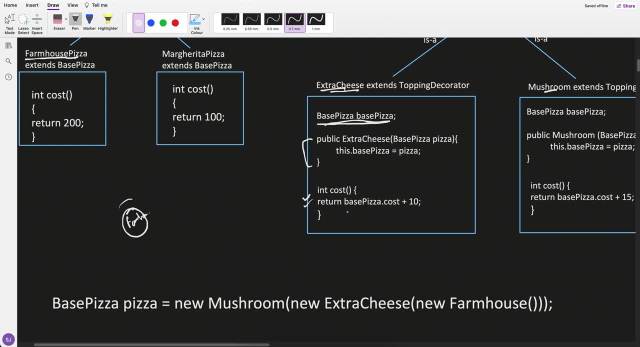 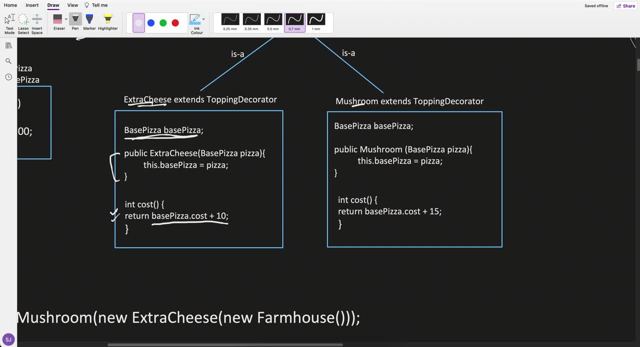 And how cost I am adding it. Whatever the base pizza cost is, I am adding ten rupees to it. Extra cheese For mushroom: The same thing. I am adding fifteen rupees. So now let's take this example. Now understand this. 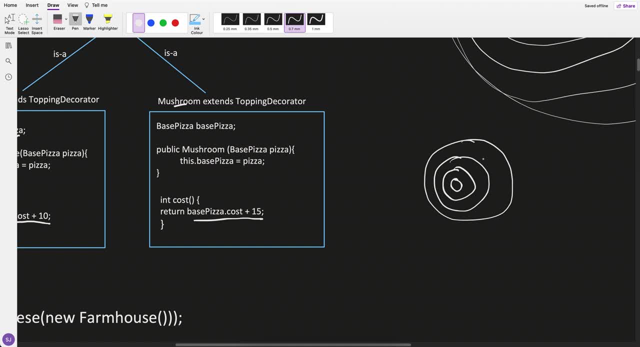 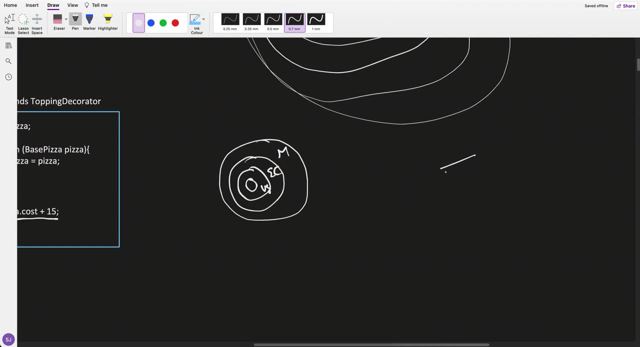 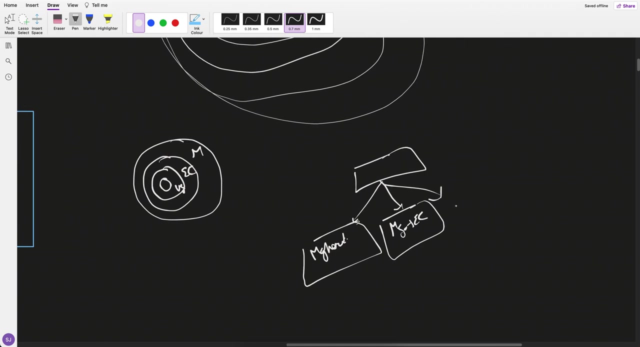 this multiple layers. now, let's say you have mushroom, you have extra cheese, you have veggies. so now, if you don't have this decorator pattern, what? how you will gonna create it. let's say you have. you will create only, let's say, margarita. you can have one class like margarita plus extra cheese. you can have one class like 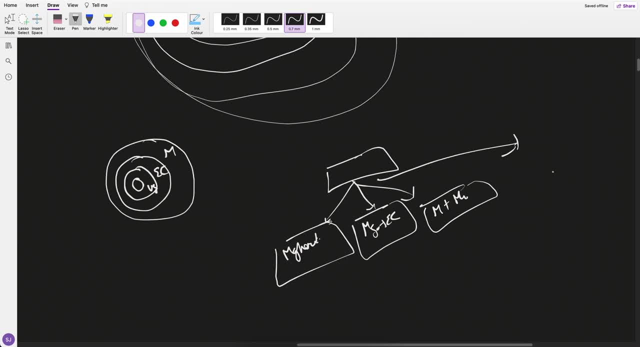 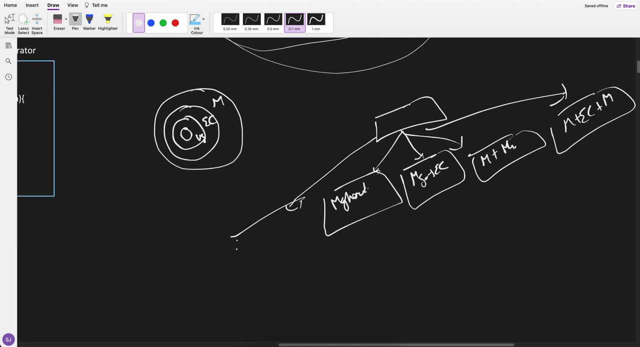 margarita plus mushroom. you can have one class like my: Margarita plus extra cheese plus mushroom. some somebody want two times extra cheese, double cheese, right, margarita plus extra cheese plus extra cheese plus mushroom. now I have Farmhouse. so now I have the same different classes for farm house, also farmhouse of extra. 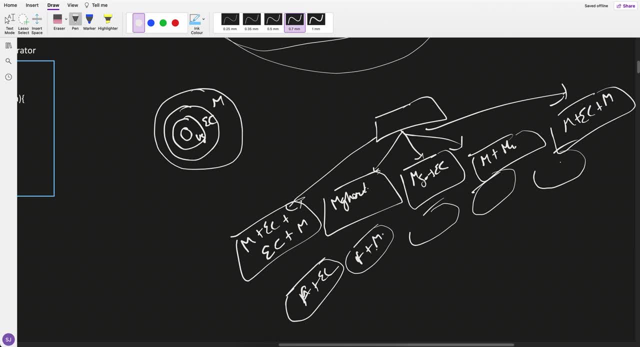 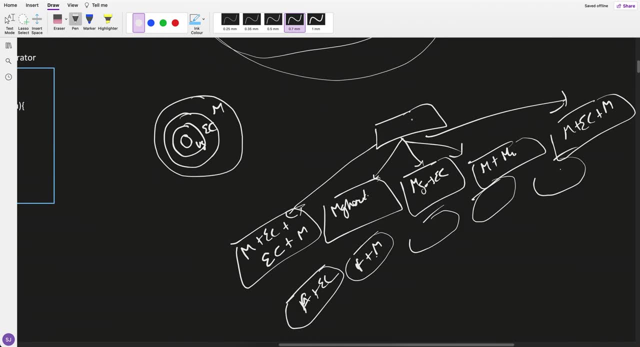 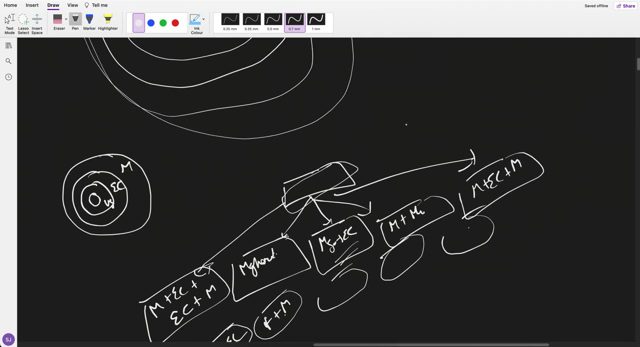 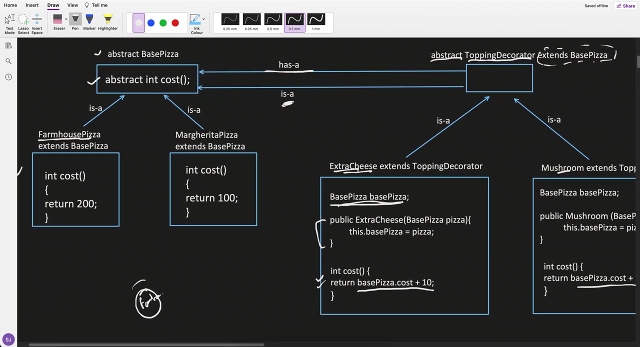 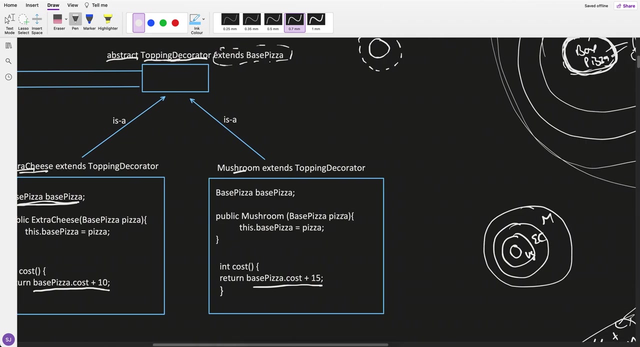 cheese farmhouse mushroom. now, if you see that you, If there are, let's say, 10 toppings, then you will. if you go with this approach, if you create a class for each combination, you will get into another problem which is called as class explosion. To save this class explosion- that's where the decorator pattern- what we have done helps it. so it separates your base pizza and separates the topping decorator. if any more topping decorator exist, add it here. mushroom with extra cheese, veggies or whatever. 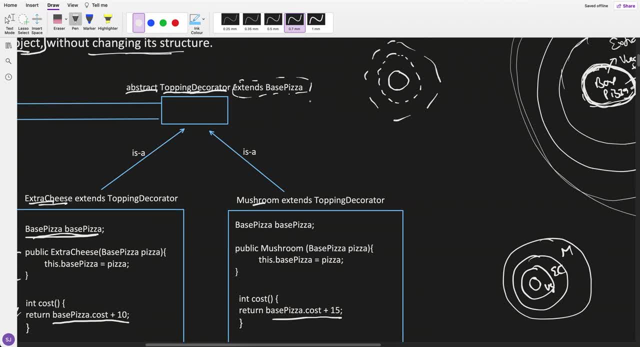 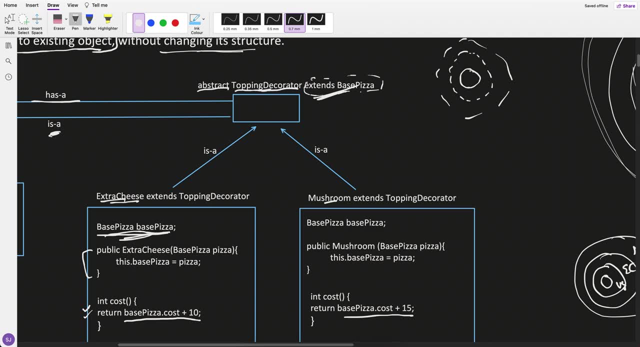 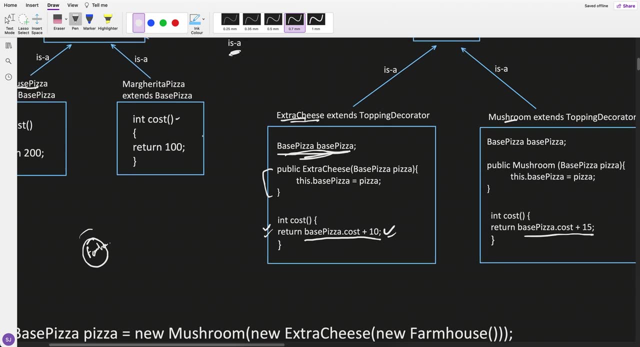 So this topping decorator itself is a pizza. that's why itself is a pizza and it also has a reference. ok, So whatever the base Pizza you will create, it will append to it. so I am just taking a feature of cost. so whatever the cost it has, it append to it. 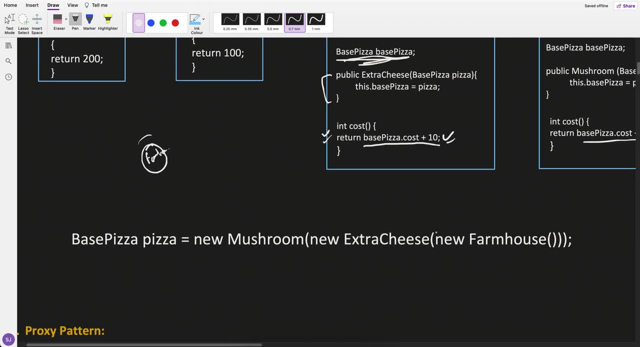 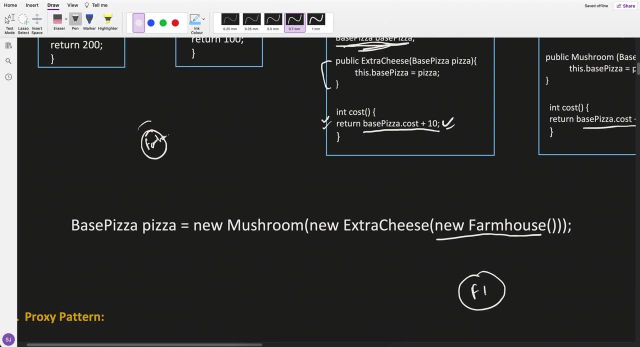 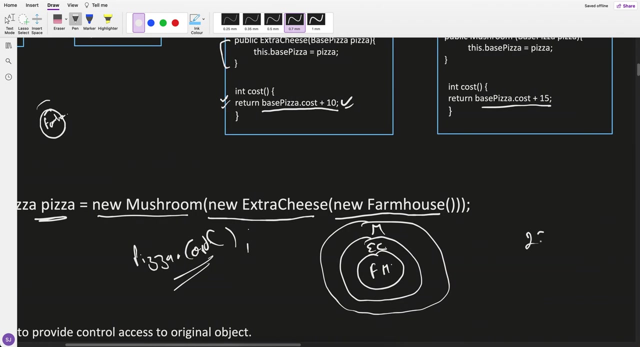 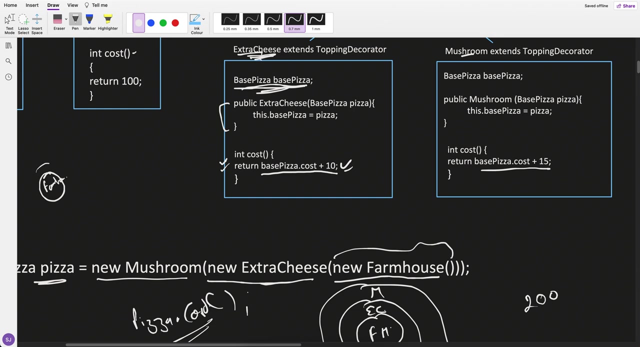 So now let's see how I am creating. so here I am first creating a farmhouse. I am first creating a farmhouse pizza, so this is my farmhouse pizza. then I am layering it with extra cheese, so I have added extra cheese, Ok, Ok. Then I have layered it with mushroom, so I have a mushroom here, ok. so now this is my pizza. if I do pizza dot cost, right, so it would be. farmhouse was for 200, right? so extra cheese in the extra cheese in its constructor. I have sent the farmhouse object: base pizza was the farmhouse. 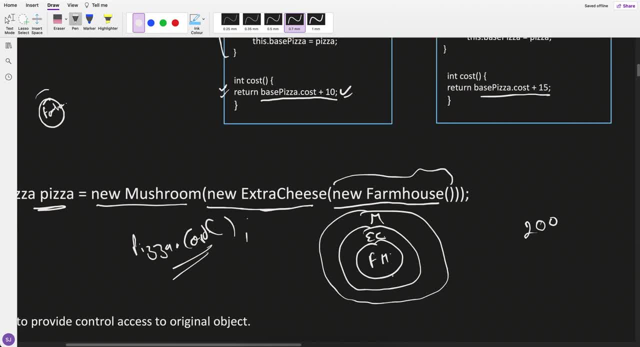 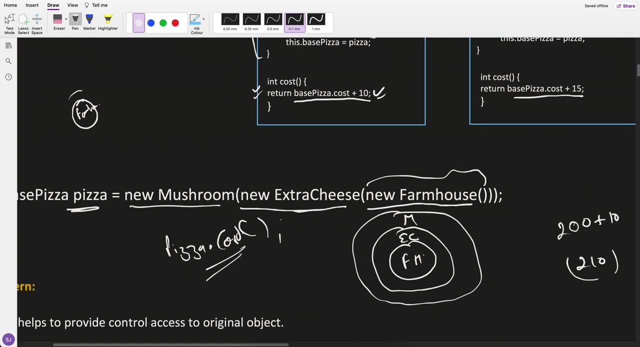 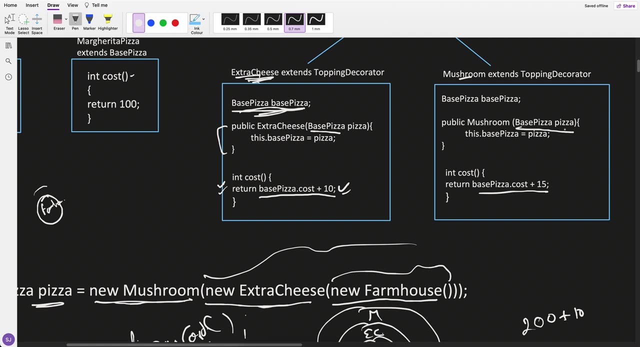 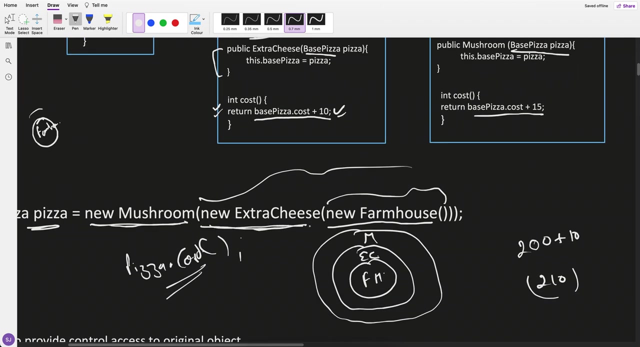 So base pizza dot cost. so farmhouse was 200 plus 10, so 210 and this 210 rupees I passed to the mushroom. so in the mushroom constructor I passed this base pizza right, so itself topping decorator it's a pizza extends base pizza right, so this itself is considered as a base pizza. so its cost so 210 plus 15.. 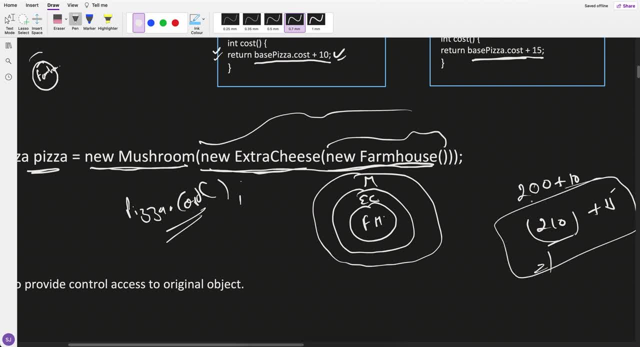 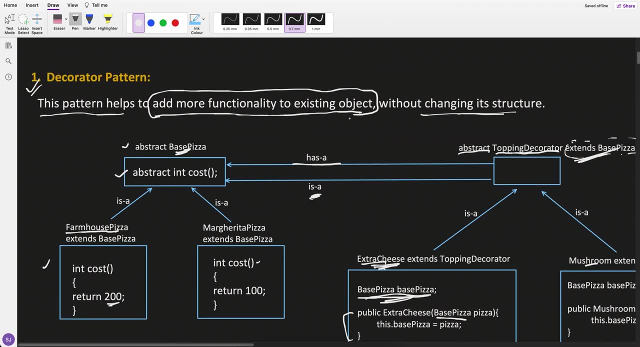 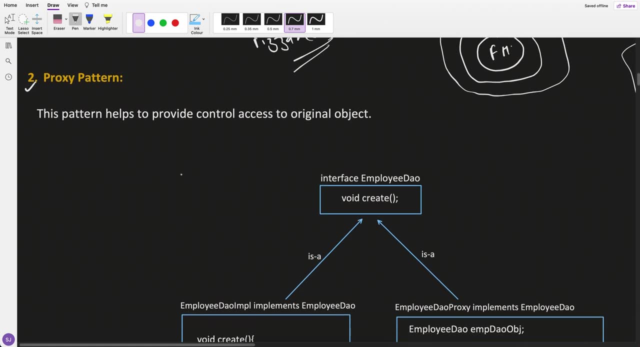 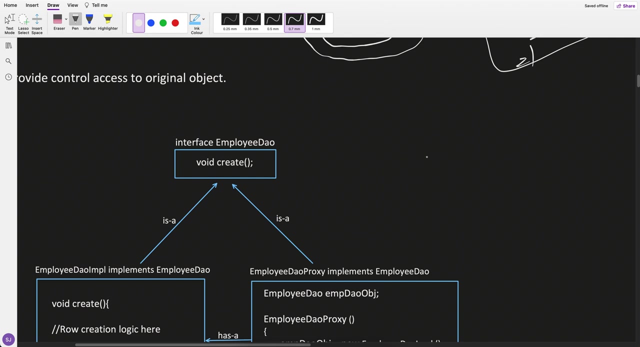 Ok, Ok. so this is your ultimately pizza cost, Got it? so this is your decorator pattern where you add more functionality to an existing object without changing its structure. Now let's see the second one, proxy pattern. so proxy pattern is very, very- you can say that- intuitive, is like somebody is in mid between your client and the resource. 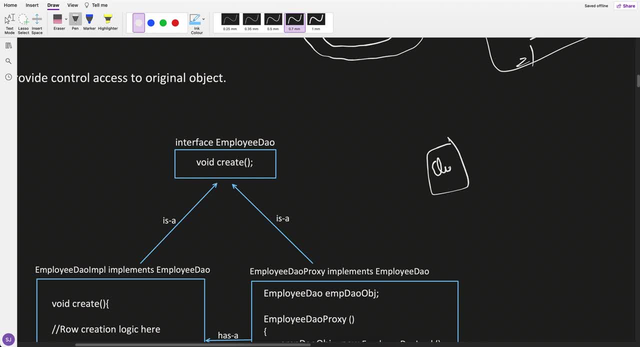 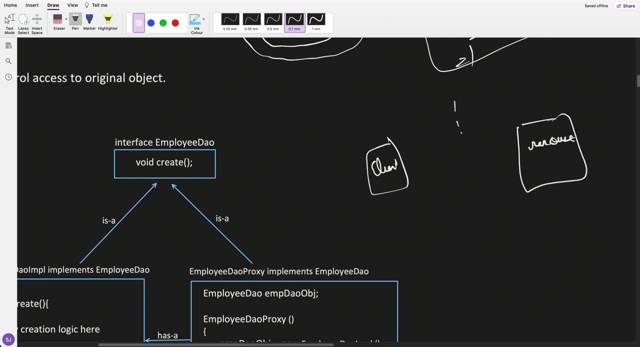 Which you wanted to access, right? So this is you and this is your, the ultimate resource which you wanted to access. so there is one proxy in mid, Ok, So it. whatever the request goes, it goes through proxy and proxy will send to the resource. whatever the request comes from the source, it goes here and goes this: 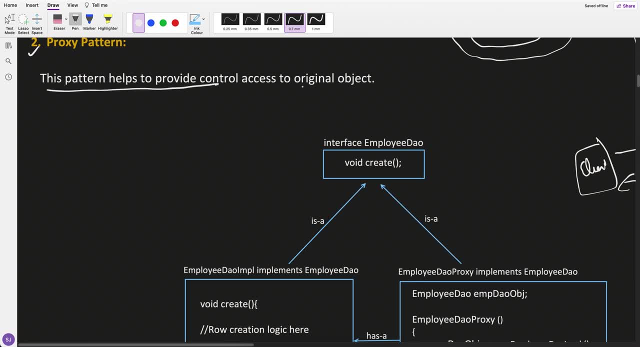 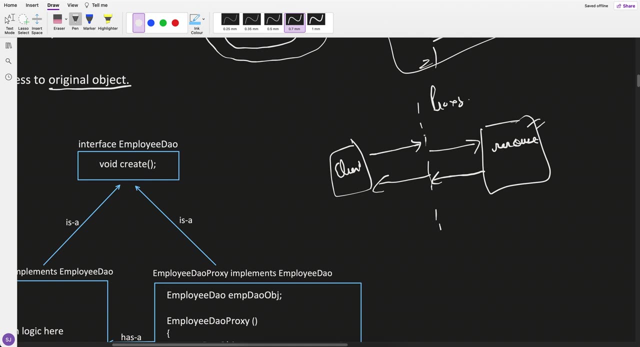 So here this pattern helps to provide control access to the origin object. so it provides some control access to original object. so it can take like who can access the resource, who cannot access the resource. or before accessing the resource, if I have to do perform tasks like logging right or some other any task, certain validation it can do right. so 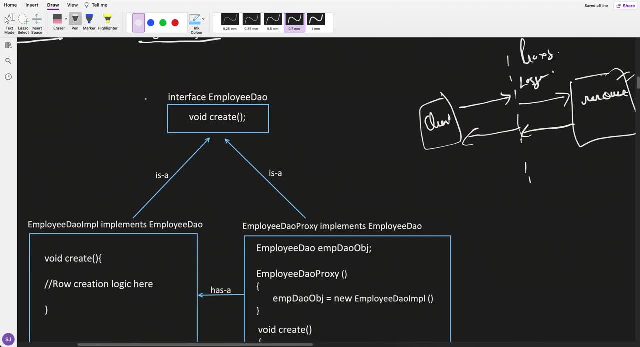 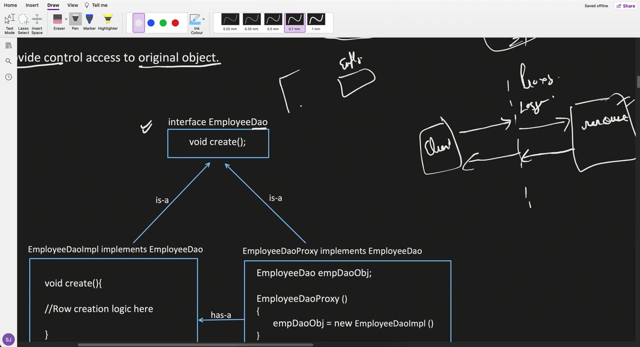 let's understand with a very, very simple example. I have created an interface- employee DAO, right? you know right now what is dow. dow is data access object which is used to access the DB. so let's say you have employee table in Java you create one dow class, which employee dow, which. 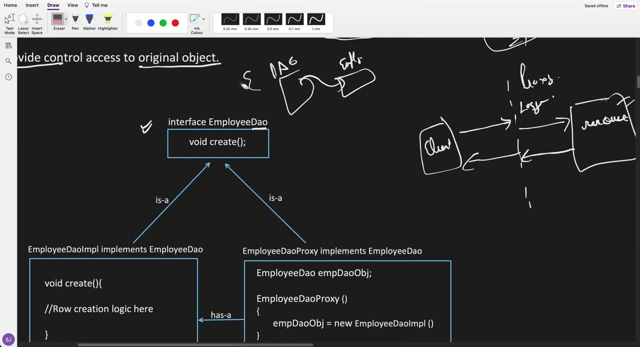 access this table right. just basic information like what is dow classes are. so now let's say I have created an interface called employee Dow and I have exposed one method- create okay. so now let's say I have created an interface called employee Dow and I have exposed one method- create okay. so 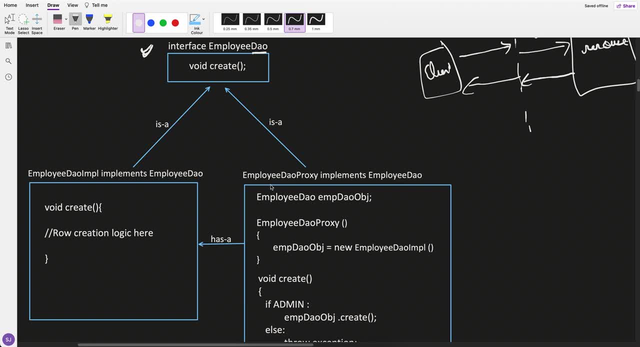 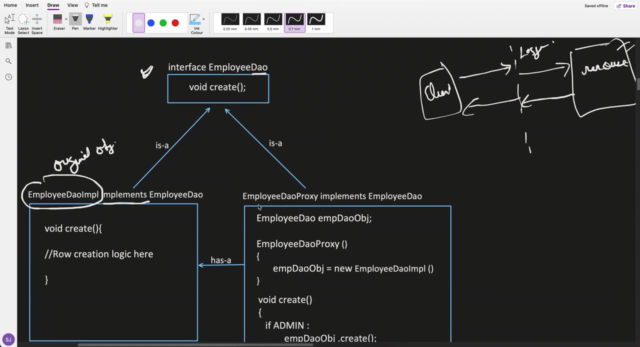 now, I have two child classes of this interface to implementation of this one implementation is employee Dow IMPL, which is your original, which is your original object, and I have also created a proxy. you have two child classes of this interface to implementation of this one implementation is: 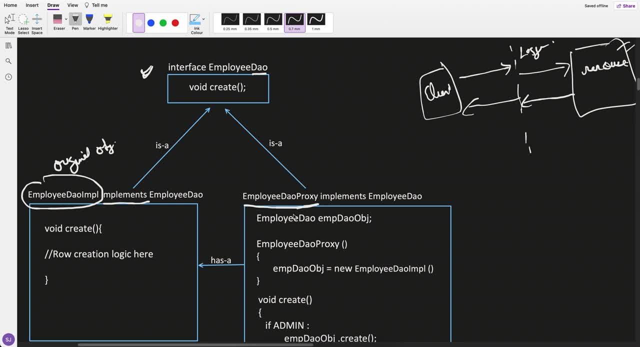 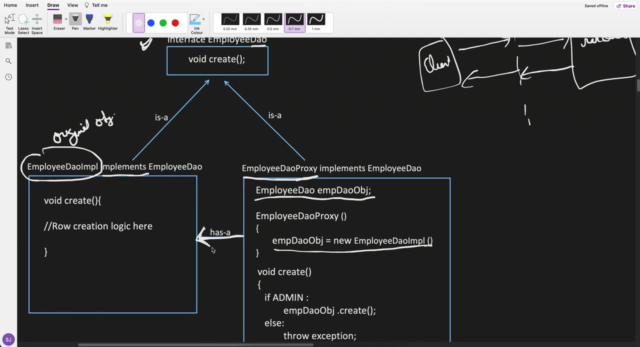 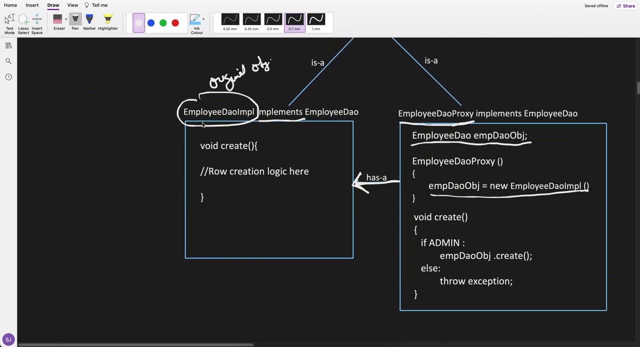 right. so I have also created a proxy, and this proxy has the original object. this proxy has theo original object. this proxy has the original object. so I have created an object or IMPL this one. okay, and now, whenever anybody greater wanted to call this employee Dow, IMPL, create method. it has to. 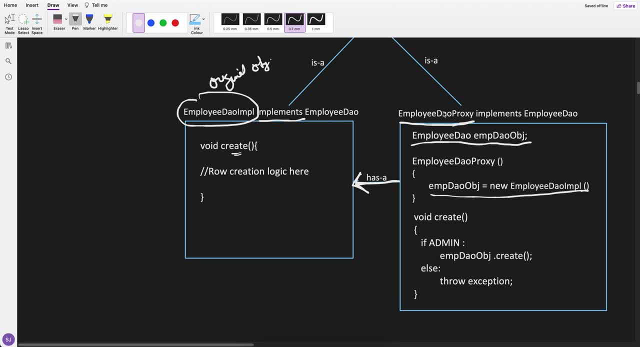 call. it is like this: custom go grab and iht délef. whatever is my node? node is this: one IMPL we just Premise, picks up a channel. if you want to typically, then you want to customize it. it has to first pass through from this proxy right. so i am creating an object, implied dow. 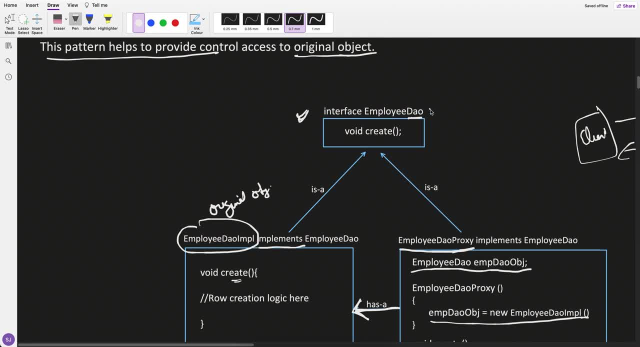 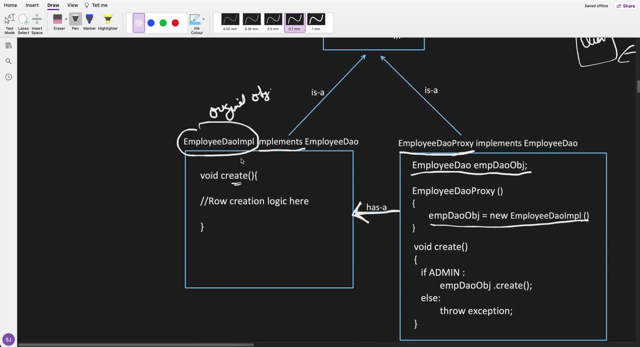 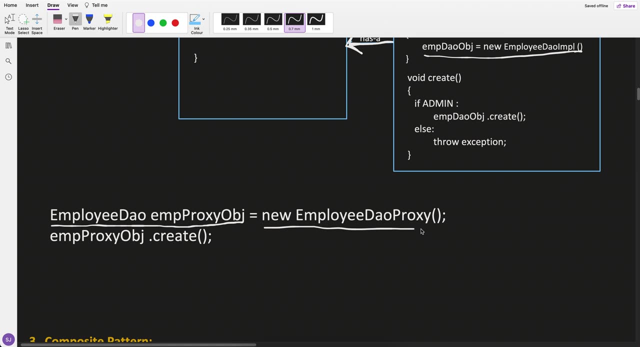 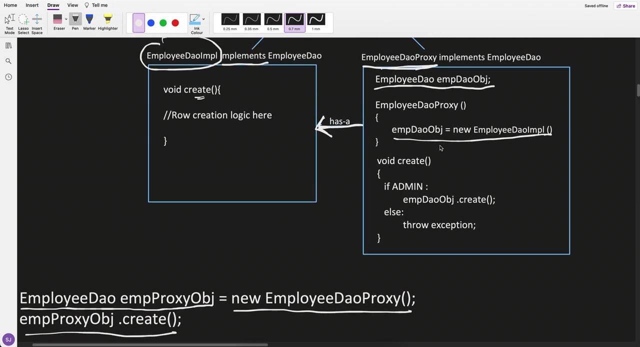 i have created an object, so this is an interface, right, it can be, so it this reference. interface reference can hold a reference of this objects, right? so i am creating an object of the proxy, new proxy, so i am creating an object of a proxy and calling the create method, so calling this. 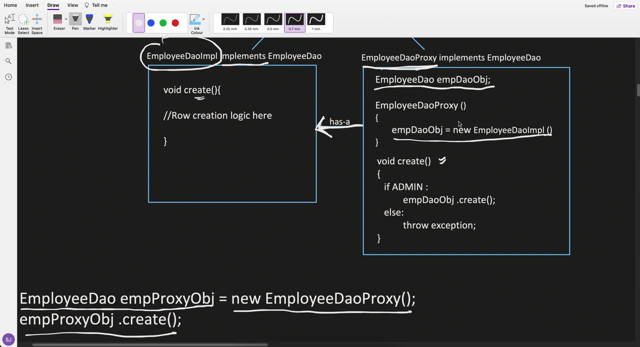 create method. now, when you invoke this proxy object, what will happen is it has the reference of this original object and when we call the create method, so what it do is it do certain validation. so i just, for example, i have added: if the request is from admin, if it's an admin call, then invoke the original. 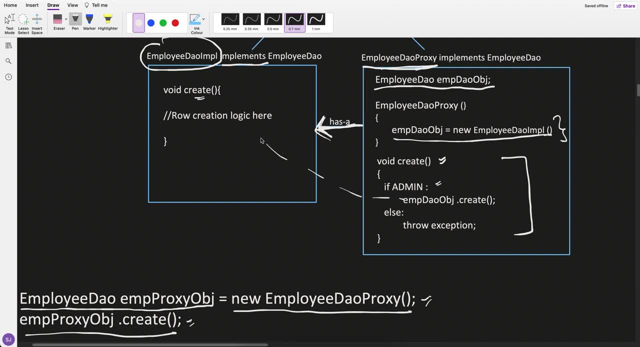 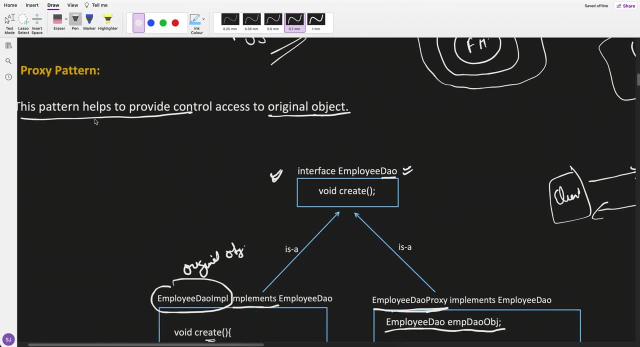 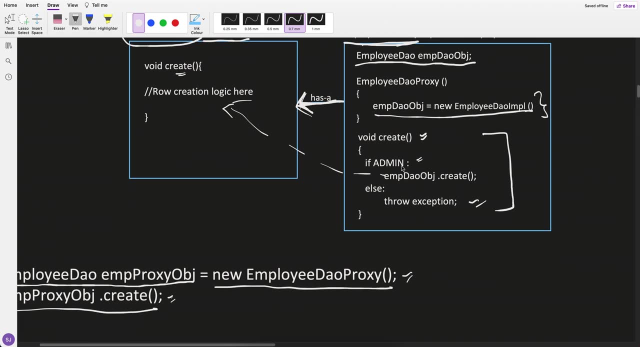 object. so now it is invoking the original object. this method, if this call is not from an admin, throw an exception. so what does it say? is that this pattern helps to provide control access to original object. so now i am controlling here if the call is from admin. 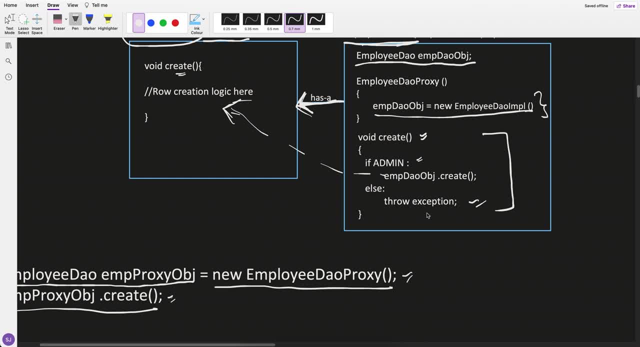 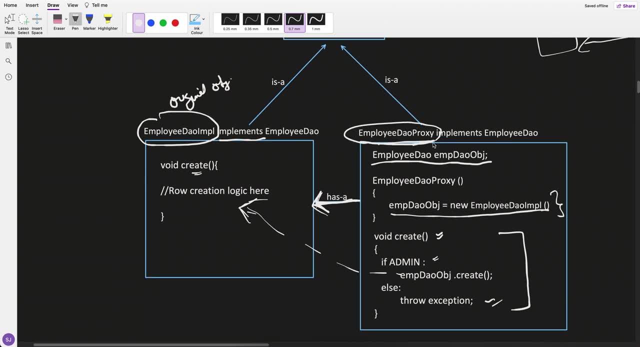 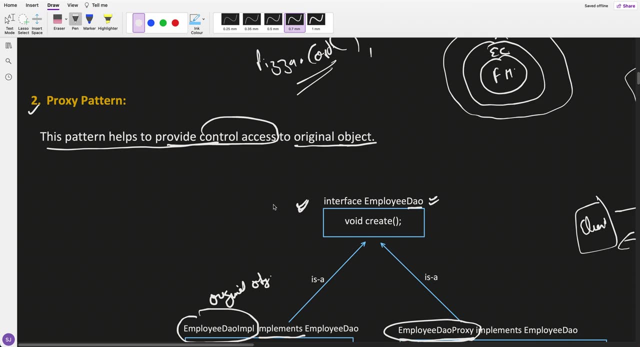 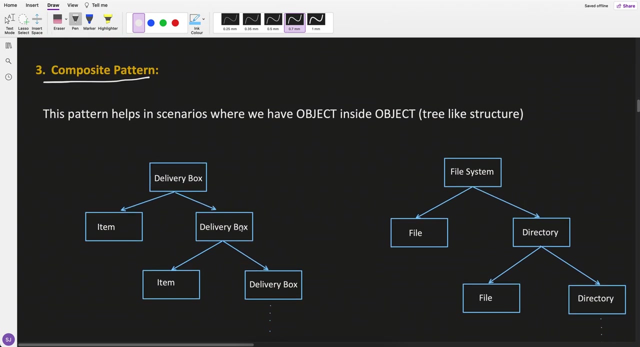 then only call this, otherwise throw exception. you got it. what does it mean? very, very simple. so here, the only thing is we create a proxy also, and this proxy has this one, and it is a part of the same interface. ok. the third one is composite pattern. what does composite pattern is this: 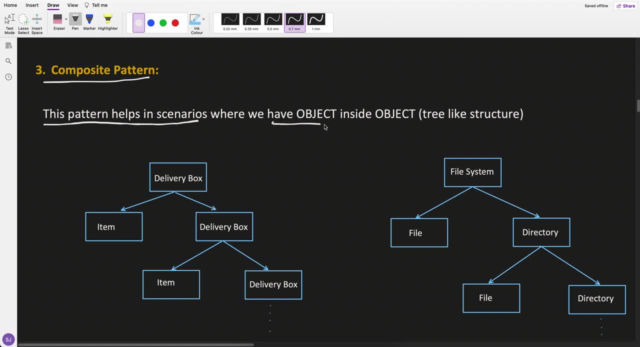 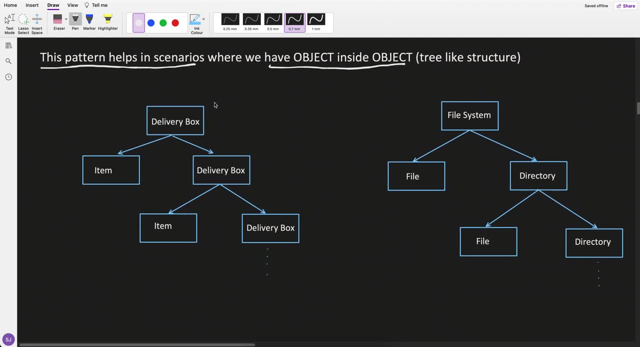 pattern helps in the scenario where we have object inside object, tree like structure, right? so just take this example: object inside object. so let's say delivery box inside delivery box, you can either have the item or generally i call this as the leaf before, so in the tree. 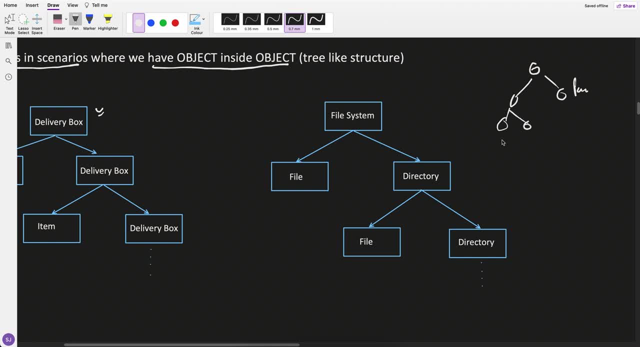 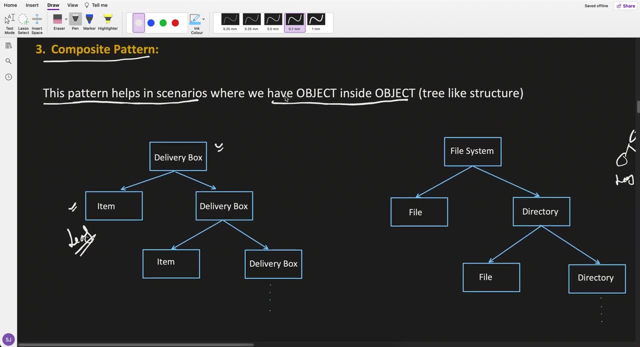 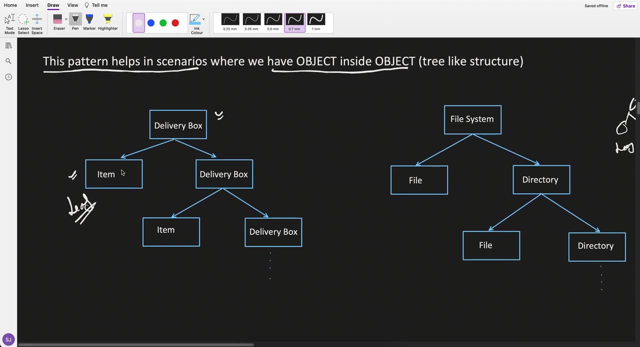 one you have is parent node and other you have is a leaf node. leaf node means they are the end nodes. so that's where, in the composite also, where we have to solve a scenario where we have object inside object tree, like structure. so delivery box can either have item and once. 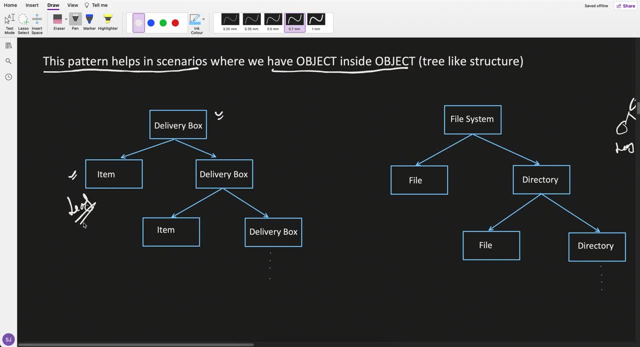 you got the item, you can't have another delivery box, right? so it's generally known as leaf and delivery box can also have another delivery box. so the same thing now, a recursion delivery box can either have an item or it can have a delivery box. similarly, it can have either. 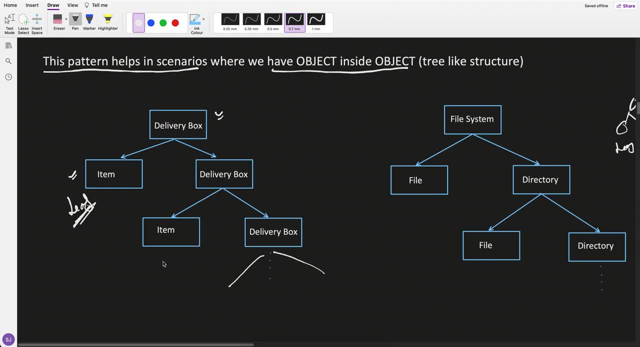 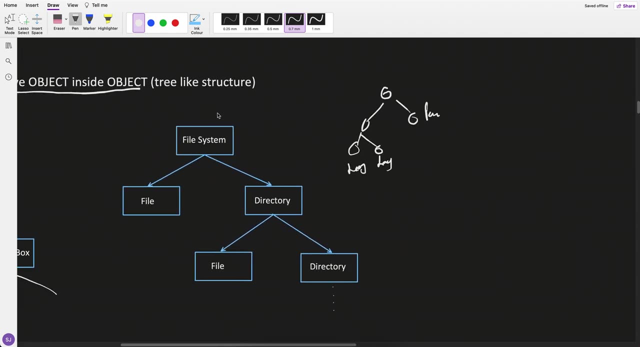 item or can be a delivery box. ok, so these items are generally a leaf nodes- you can say that- and this delivery box are nothing but a composite objects, right object inside object. another example is file system. let's say i have a file system. inside this file system, either you can have a file which 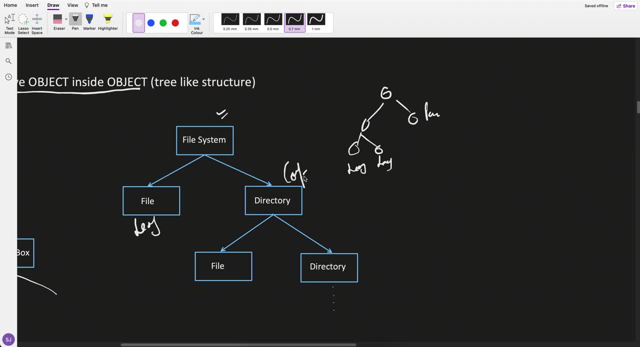 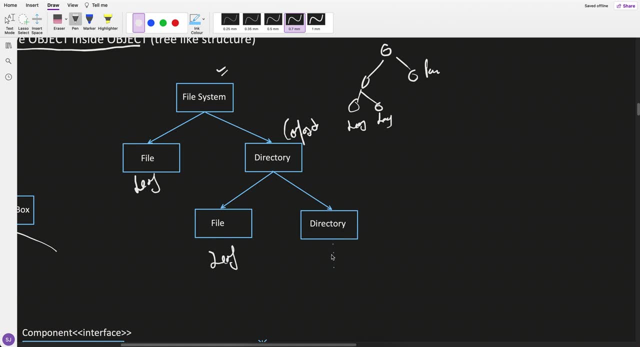 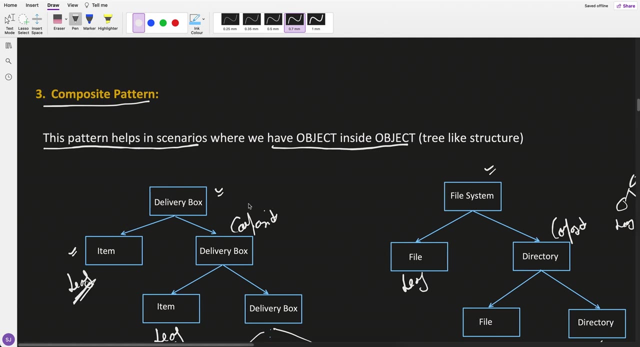 is a leaf, or you can have a directory which is a composite and this directory can again have either a file, which is a leaf, or can again have a directory. then this directory again can have a file or again have a directory. like this goes on. so this is just an example to identify the scenario where the composite pattern can be. 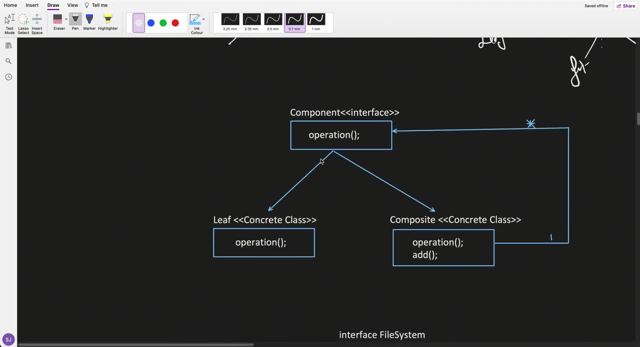 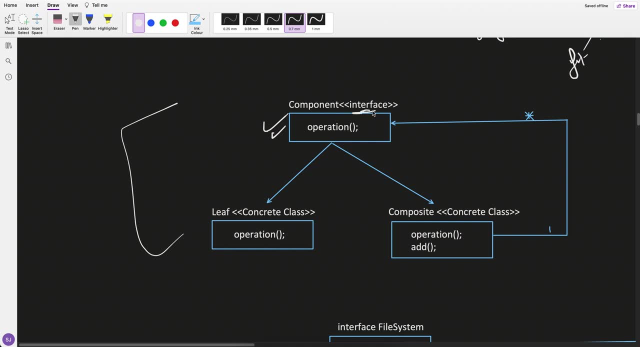 used like object inside objects. so this is the uml diagram, like your component, which is an interface and there is an operation. so either it can have a leaf, or it can have a leaf- Concrete class, Operation implementation, or either it can have a composite and if it is a composite it go. it's a recursion kind of thing. 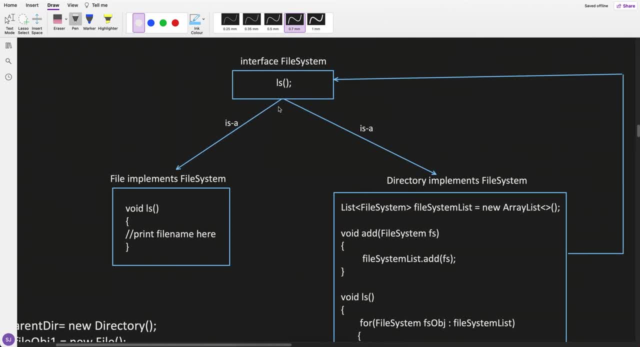 We'll see with an example. So now let's take this an example of a file system. So I have created an interface file system. Okay, so this LS, LS is used to print, right, Let's say it is used to print. So I am using this method, which is used to print the file. 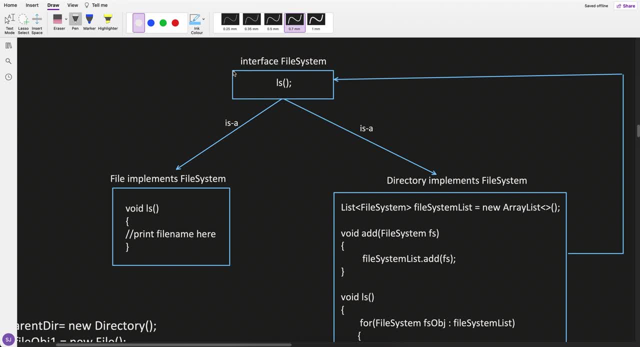 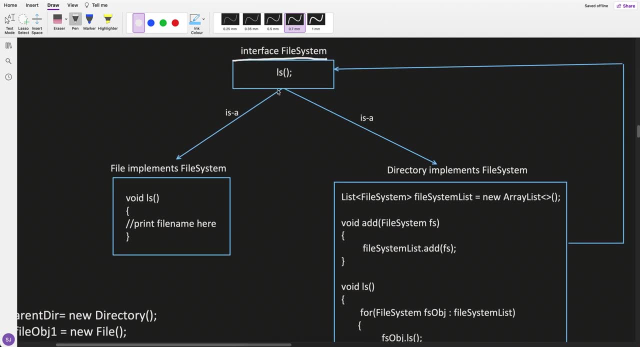 name. Let's say so. I have created an interface file system and one part is the leaf part where this file system directly have a file. So I have created one file which implements the file system and this implement this abstract method and print the file name here. 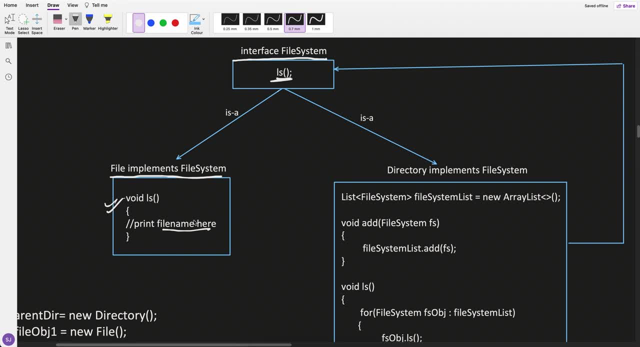 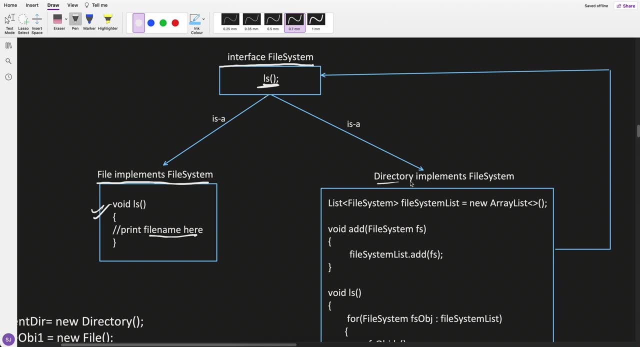 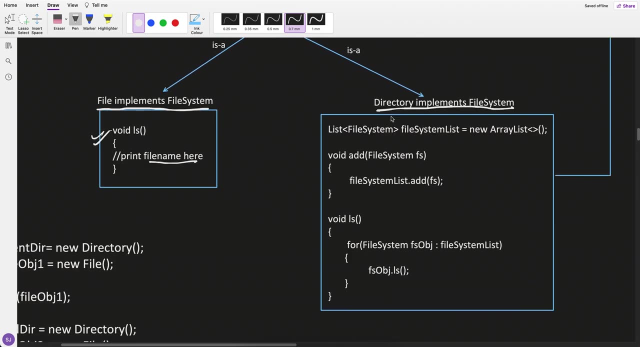 Let's say anything, whatever the file name would be. let's say it print Here. but another possible use case be: instead of file, It has a directory. So now it has a directory. So directory implements file system, right. So it is a. so inside a directory, what should be the implementation? 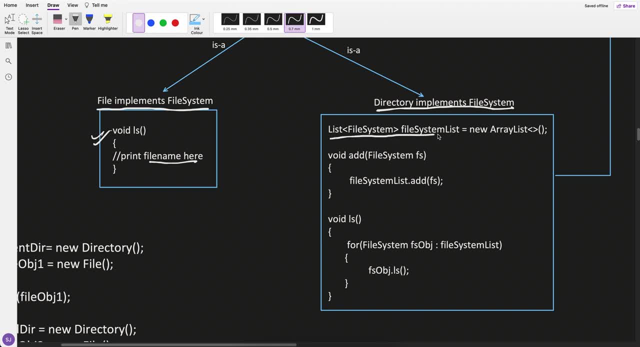 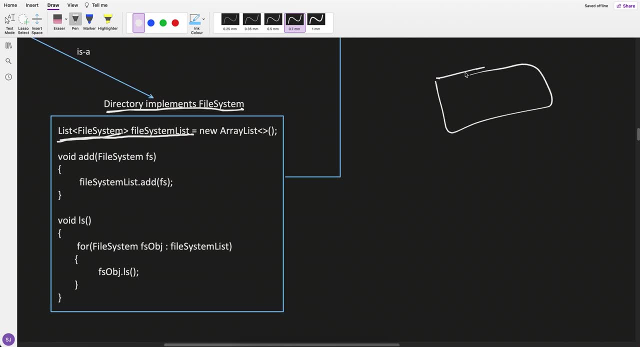 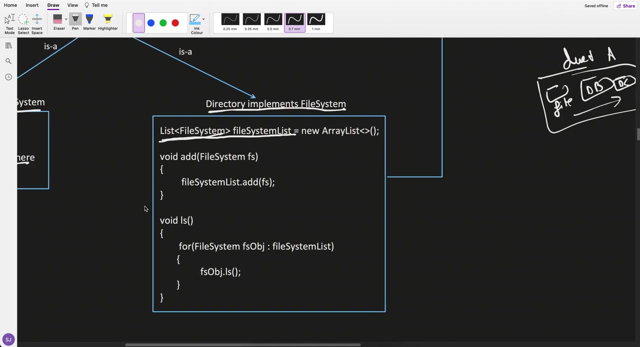 is directory, have a list of file system. It is a list of file system, Right? So let's say you have a directory A, so directory a can either have file either have can more directory, directory B, directory C, so it can have a list, right? 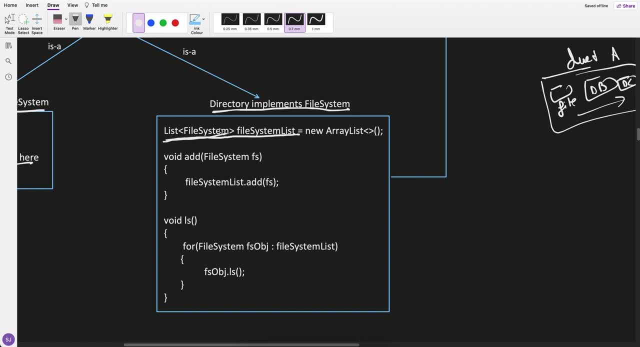 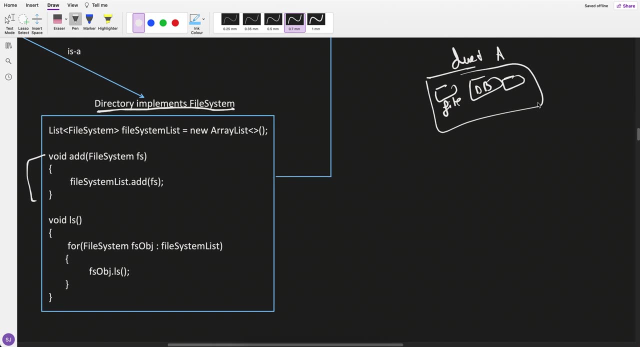 So list of file system. And list of file system is: it can be a file, It can be directory and there can be more than one. So I have added one method is add Right. So because in a directory you can add either file or directory. 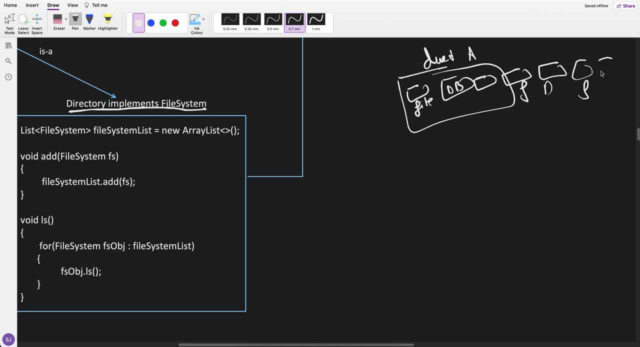 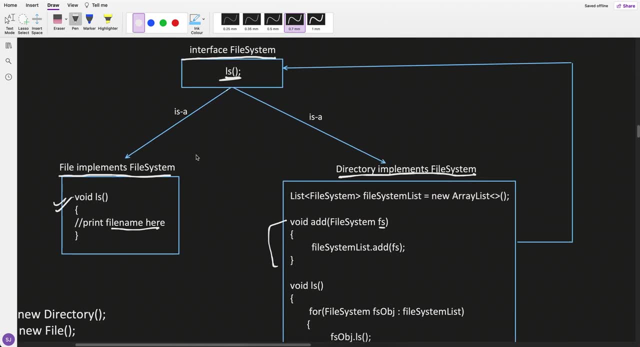 either file or directory. either file or directory. You can add more file or more directory, Right? So whatever the file system would be, because file system is an interface, It's apparent. So either you can have a file or either can have a directory. 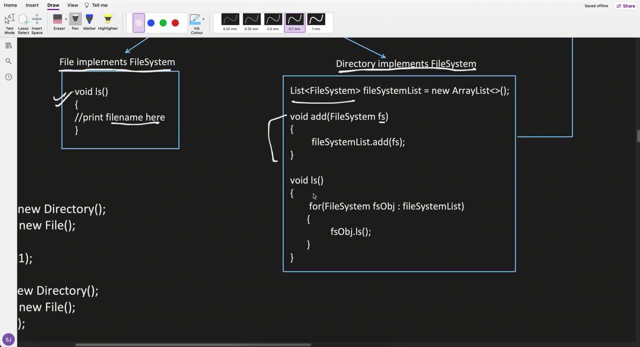 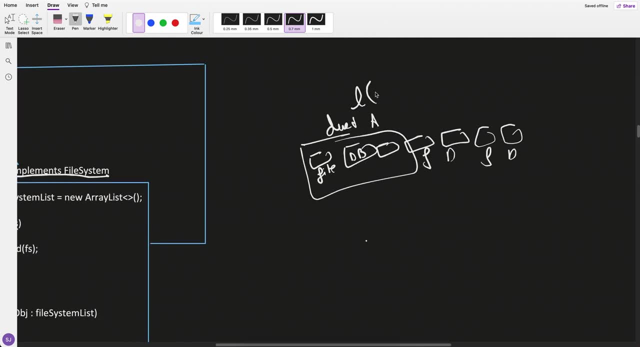 So you can add into the list And whenever the LS implementation, what I have to do. So whenever the LS in a directory is happen, LS, what it has to do if it is a file name. So I have to iterate over this list. 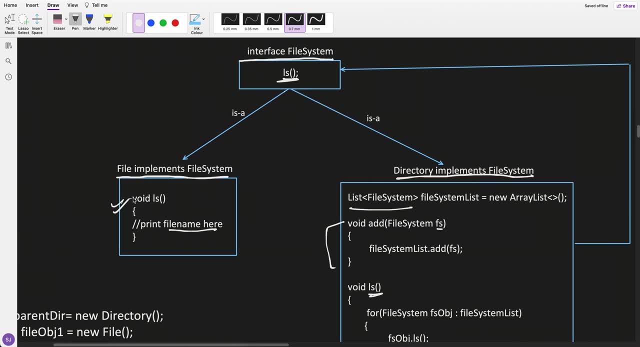 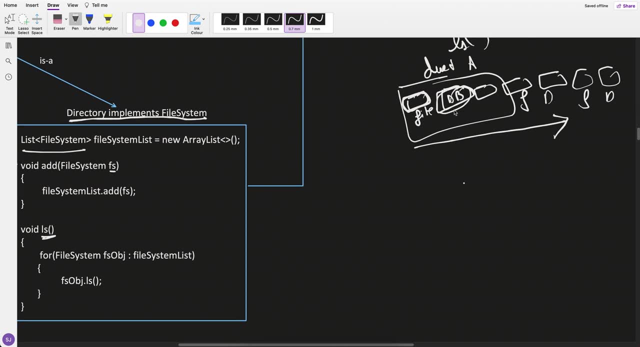 And if it is a file, I have to invoke the file one, this one, and if it is a directory, I have to do the same thing again, because this directory itself, internally, can have a file Directory, file directory like this, Right, So the same iteration has to be done for it. 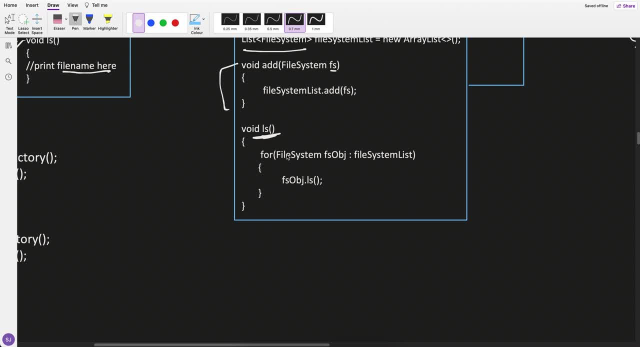 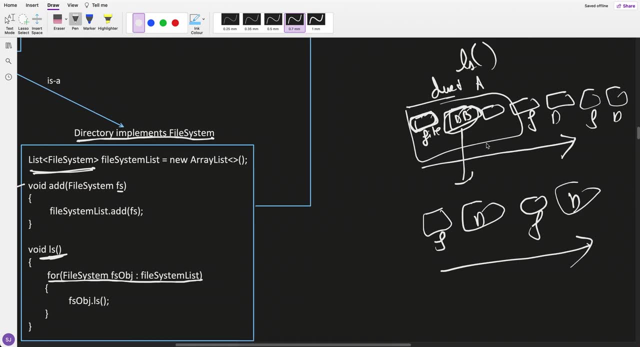 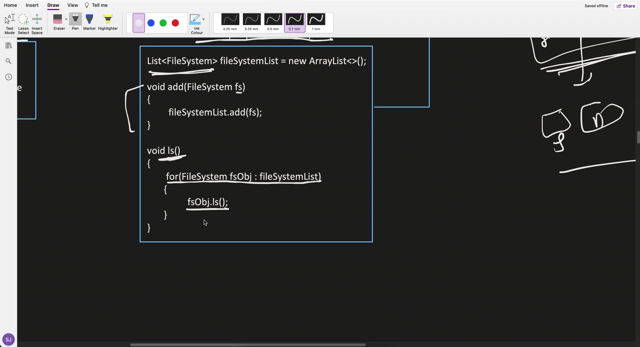 So the same thing I'm doing it. So in the LS part, what I am doing is I am iterating a for loop, I am iterating over the list, I am iterating over this list, Right, And I'm just calling this LS. 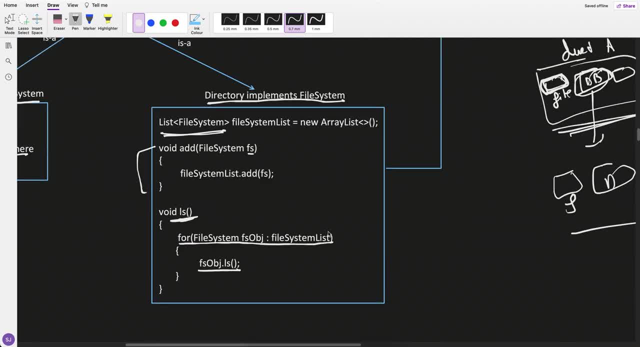 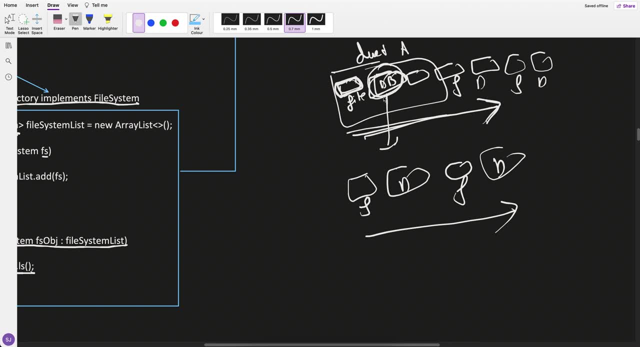 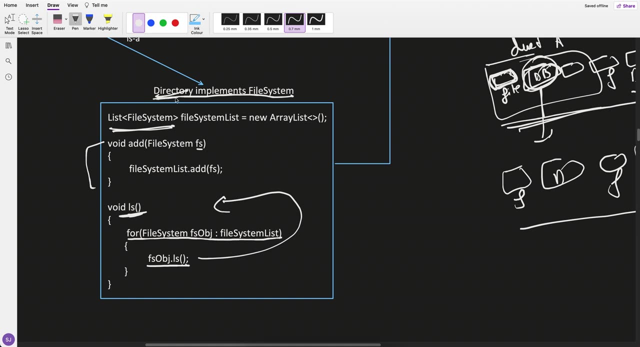 So now, let's say, if it is a file, It will invoke this LS and it will print the file name. And let's say, if it is a directory, Then it will call this, This method again, Because this is the directory class. 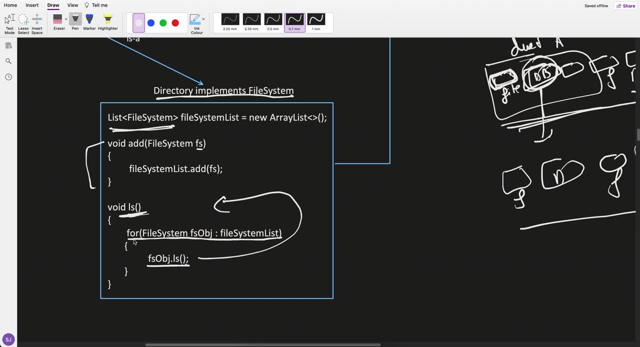 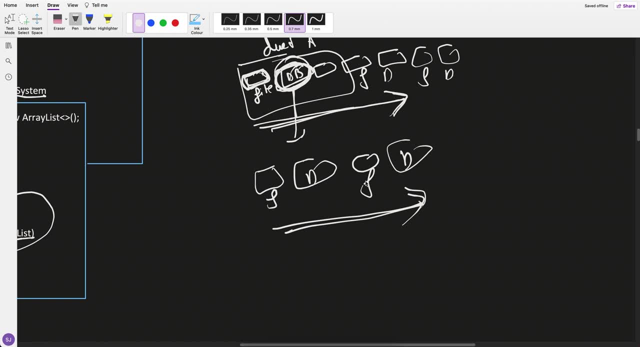 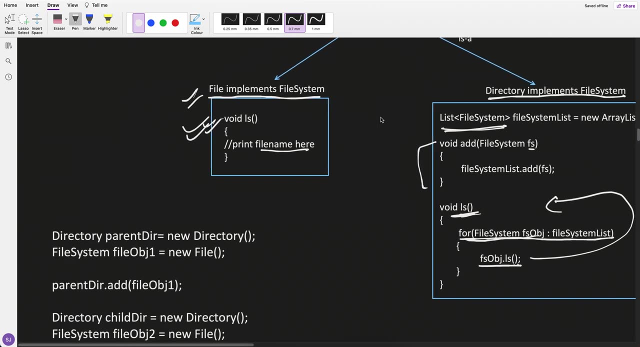 If it is a directory, this will call its LS again and it will go again for loop. So in this directory, whatever the list would be, it will first complete that, then it will. after completion it, it will move forward to here. Okay. 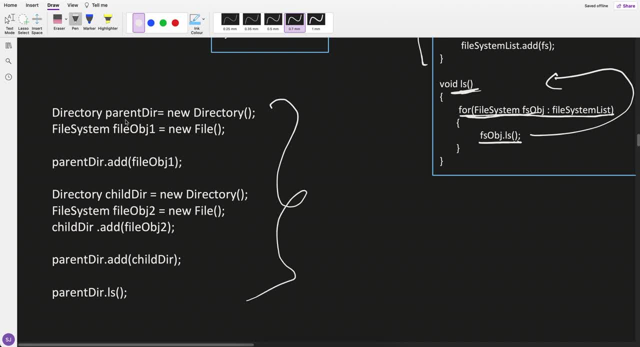 Got it. So this is just an example for it learn. I have created a directory, parent directory, Parent directory. Inside the parent directory, I have added one file, File one. then I have created child directory. Okay, then I have created a child directory. 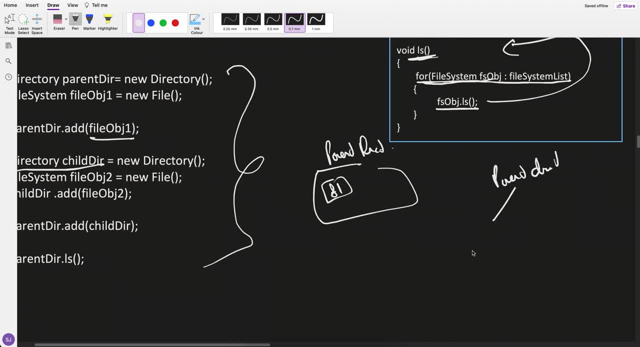 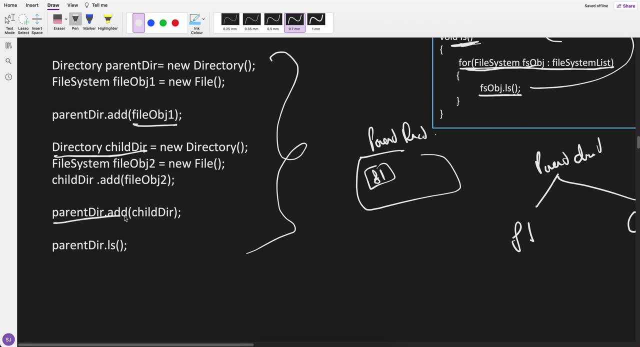 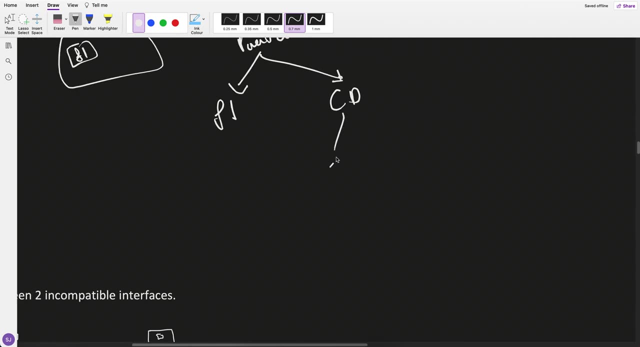 So this is your parent directory, So it has file one. then I have created child directory. In the parent directory I added the child directory And this child directory has file to this as file to. that's all. So now I am doing parent directory dot LS. 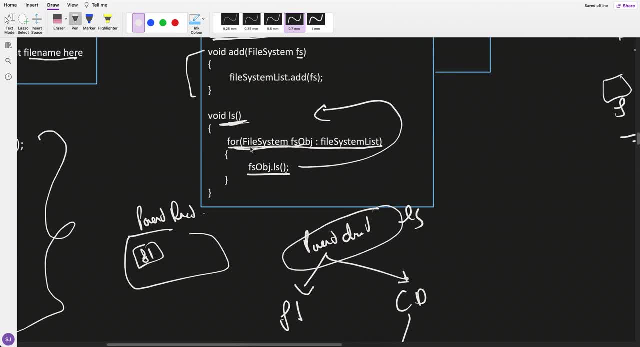 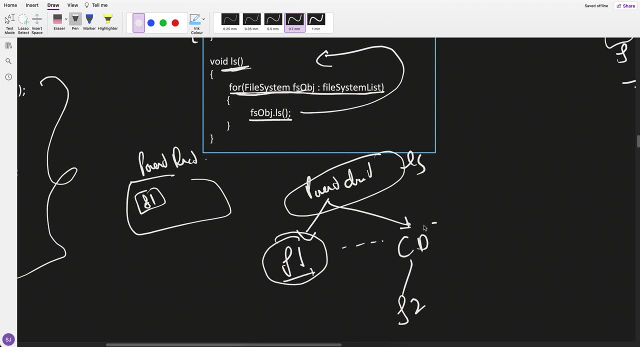 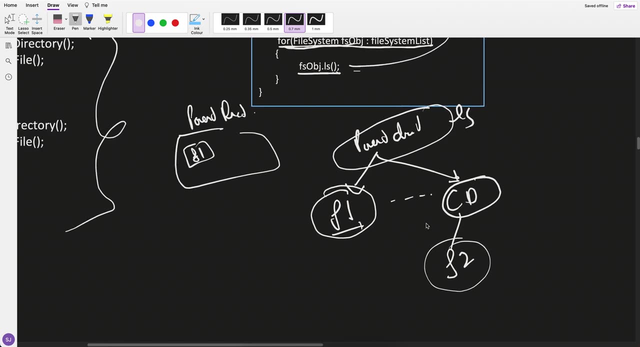 So I am doing LS here. Okay, so it will iterate over this. first It will go here, It will print this, then it will go here And it will call LS here. So it will now go to its child, So it will print F2 also. 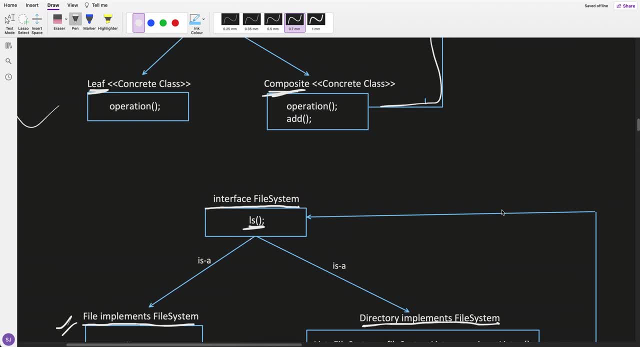 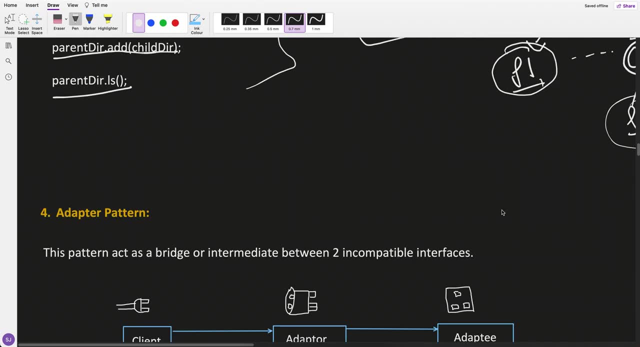 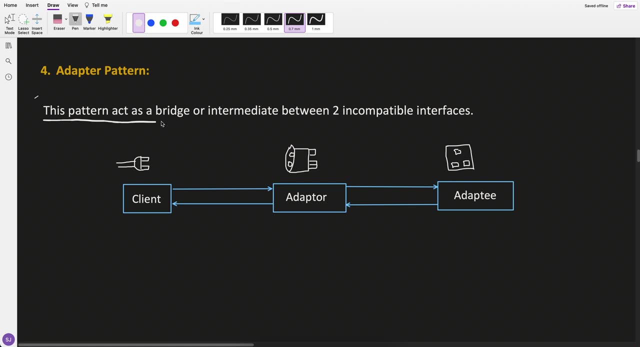 Okay, got it. So it's a kind of a recursion when very simple to identify where to apply the composite pattern. Okay. The fourth one is adapter pattern. So very, very simple understand this. this pattern act as a bridge or intermediate between two incompatible interfaces. 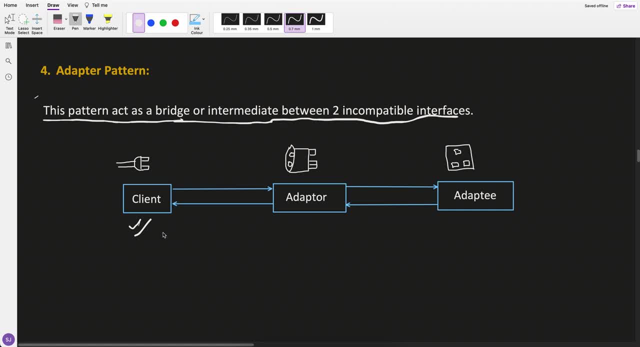 Okay, So this is an example. You have a client which wanted to access this adaptee. But see, client has this kind of a structure. adaptee is this kind of a structure. both are incompatible. So that's where adapter comes into the picture. 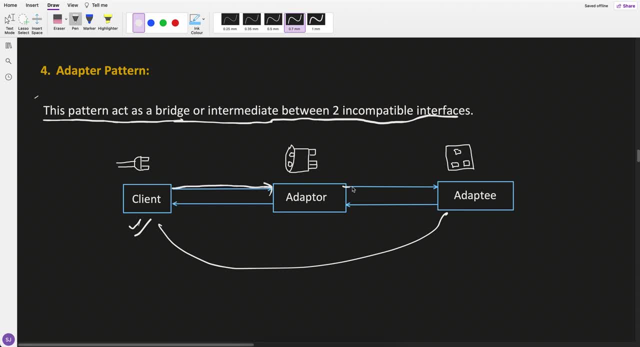 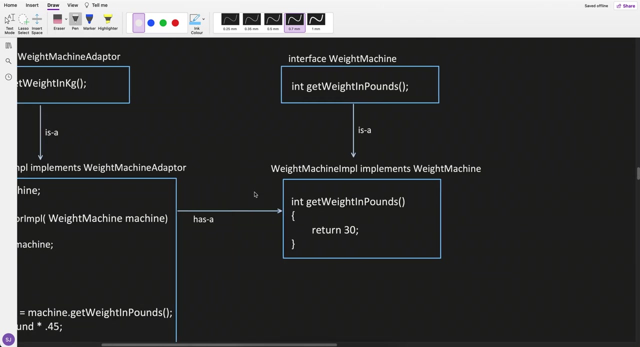 So client calls adapter, adapter calls adaptee, like whatever the adaptee understands in that manner, adaptee returns to the adapter adapter change the response, whichever the client understand, and return It okay, So it is a mediator now. So understand this with a very simple example. 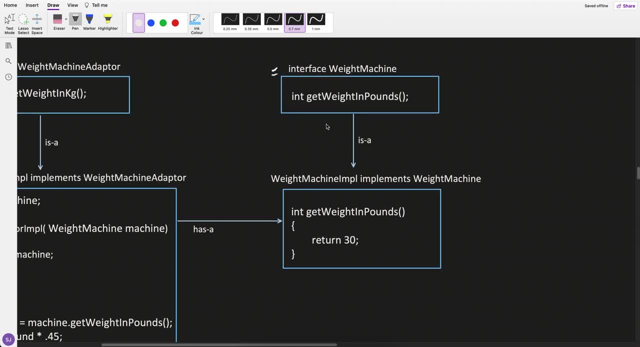 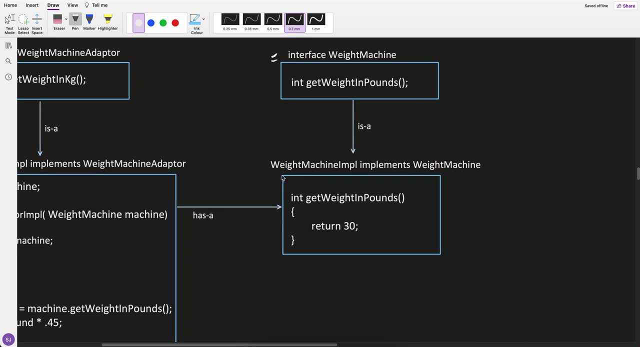 I have create a weight machine interface. Let's say so. this machine returns the weight in pounds, right, So I have. so this is just an interface. I have created, implemented it. this method get weight in pounds. Let's say it is simply returning 30.. 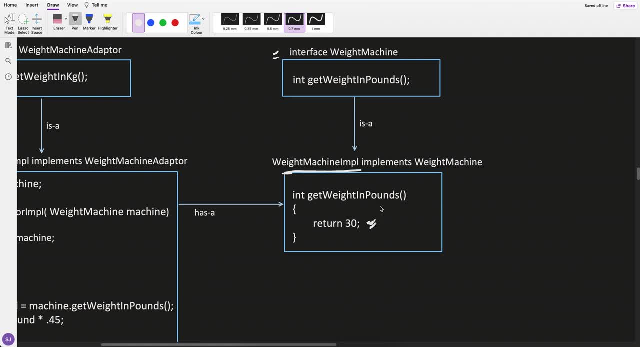 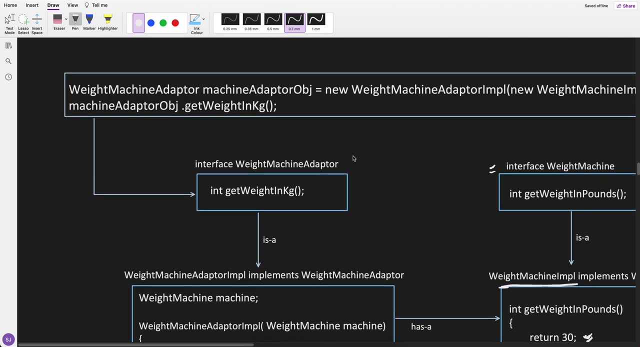 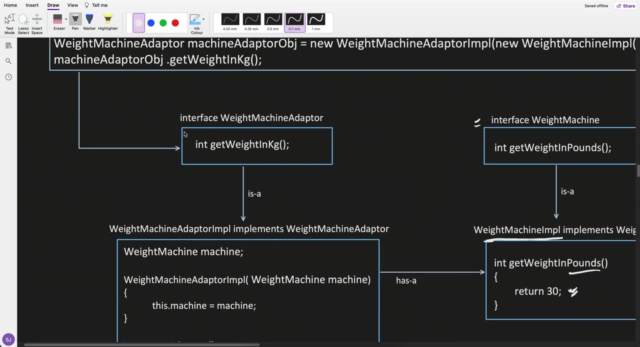 Right, I have a hard-coded it that's returned 30. So this is returning in pounds. Now I have a client which want in kg. Right, but client only understand kg. It doesn't understand the pound. So that's where I have created one adapter. 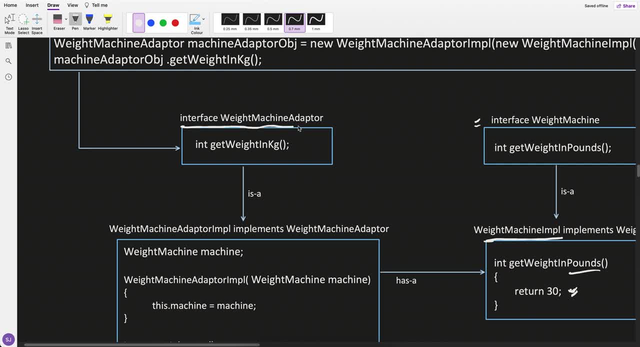 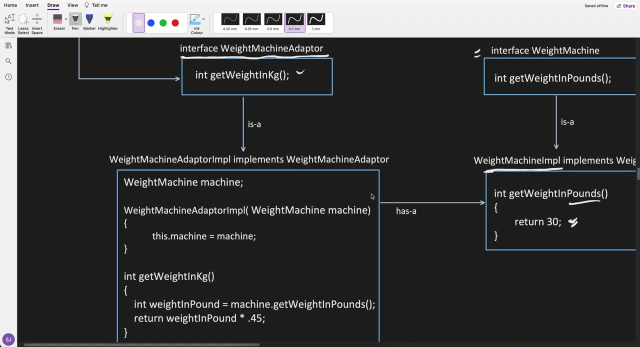 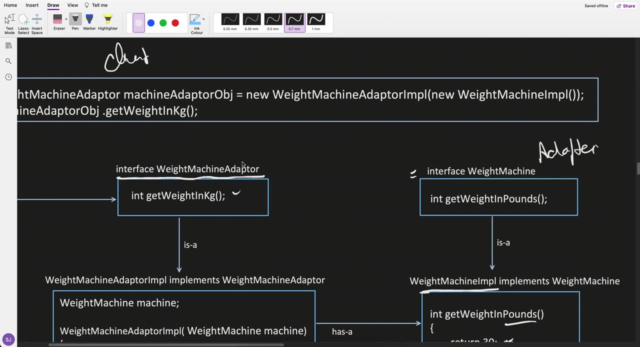 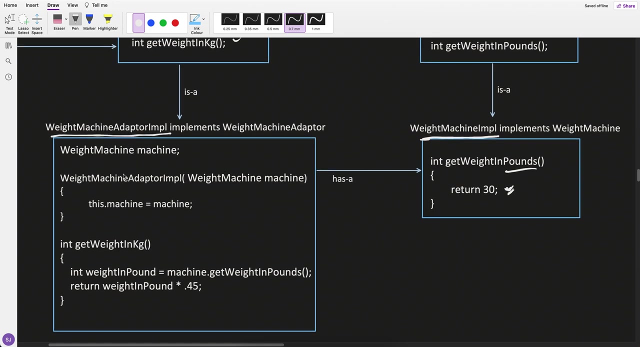 So I have created one interface and name it weight machine adapter. So it's method is get weight in kg. So now it is just a mediator between the client and adaptee And this is your adapter. So I have implemented this adapter. So now this adapter has your adaptee. 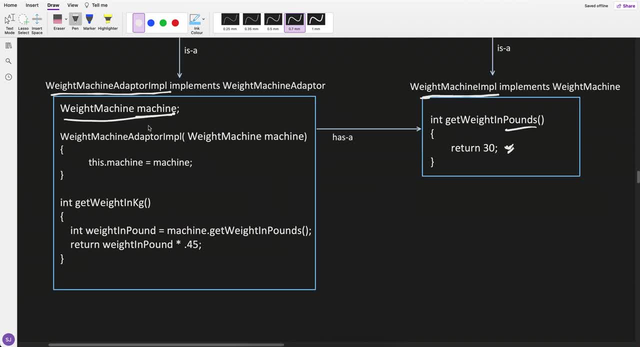 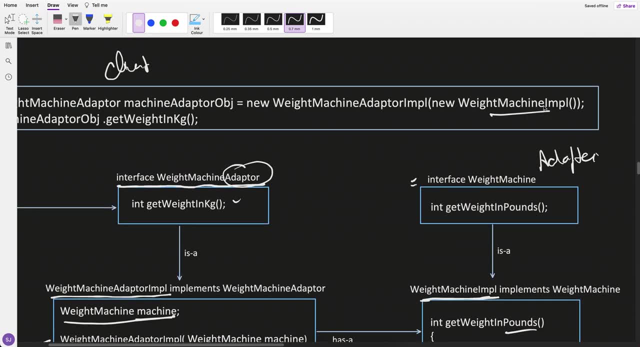 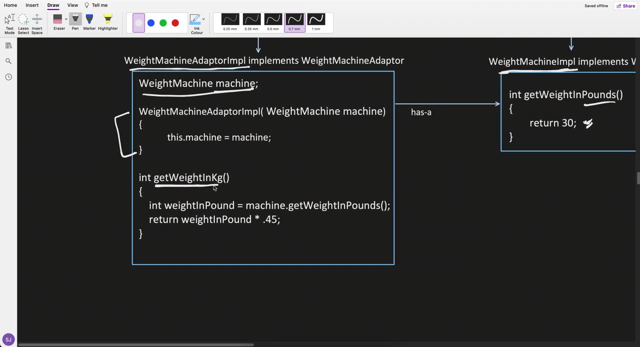 So it has an object of weight machine. Okay, so this is just a constructor to initialize this weight machine with the IMPL objects, right, with the IMPL object. Now, when the object is constructed, when this get weight in kg, so client will invoke this because client cannot interact with this directly, because 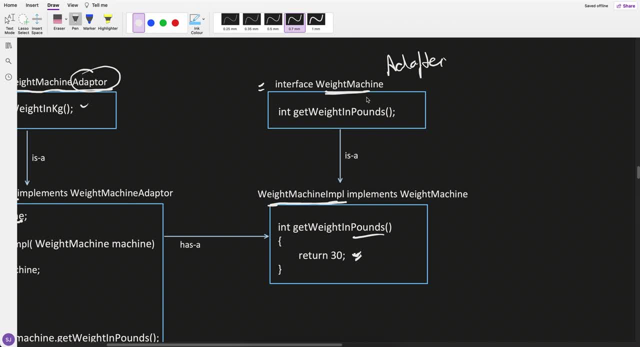 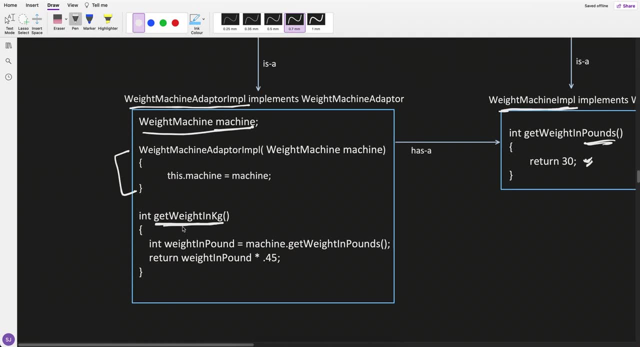 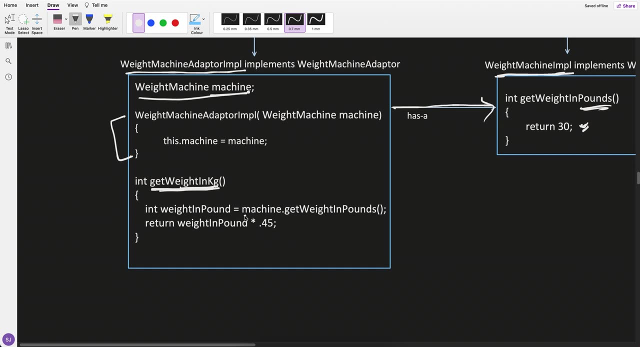 client understand only in weight. but this adaptee returns in pound. So client is invoking this adapter Get weight in kg. internally It invokes this get weight in pounds, So it has this. it has weight machine, So it calls get weight in pounds. 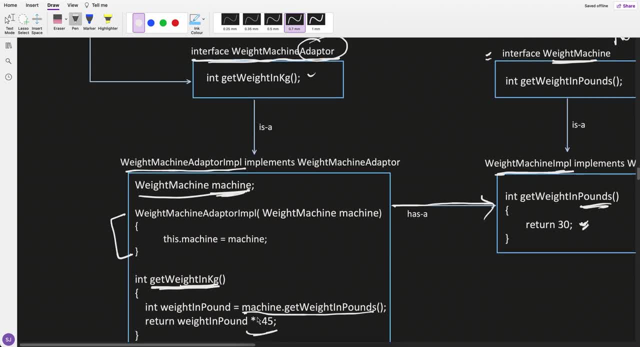 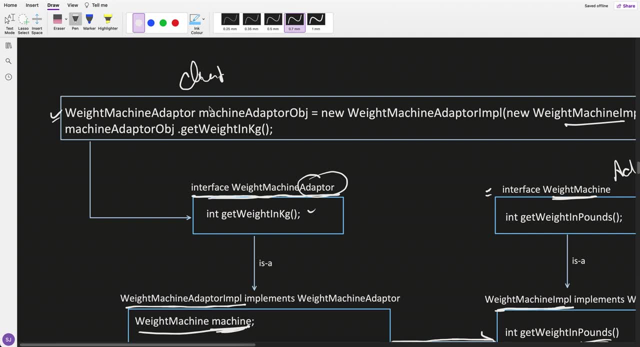 It converted to a weight machine, So wait and then return it, and then return it and the when client get received in the kg itself. So client is creating an adapter. So client is talking to an adapter, not with the adaptee. So client is talking to an adapter. 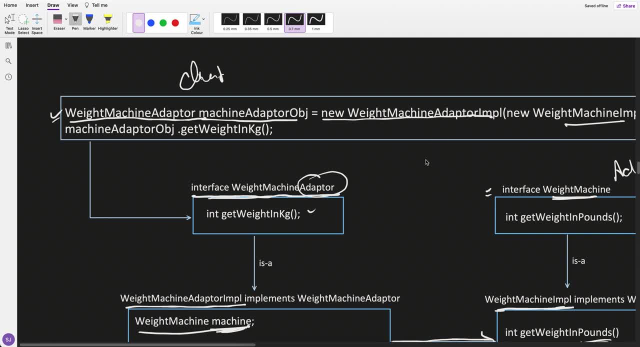 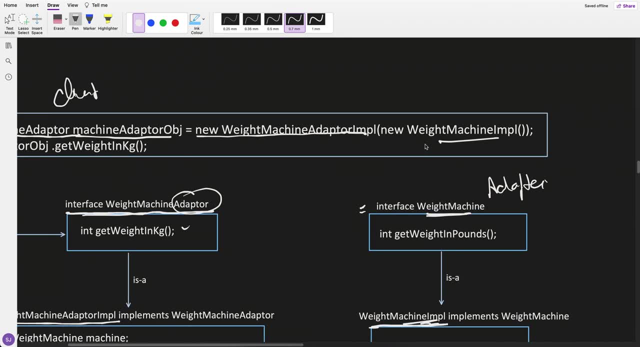 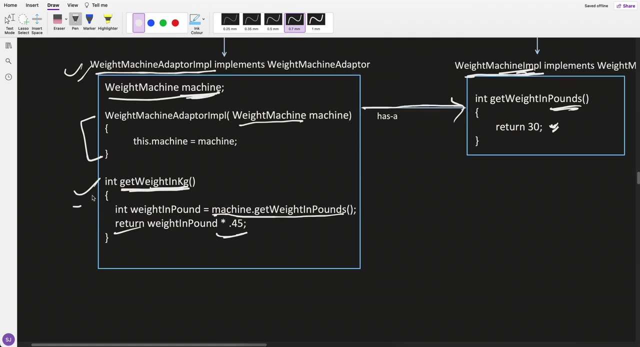 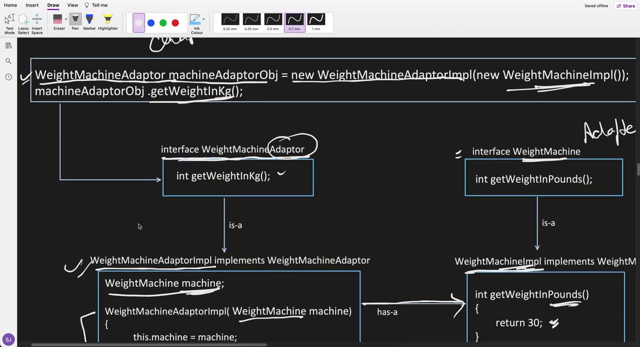 So it creating a new adapter object right. new adapter IMPL and weight machine. it pass an object of this IMPL Right. So now it calls get weight in kg adapter. So this method get invoked. It will first call the pound method, This one converted to kg and then return. 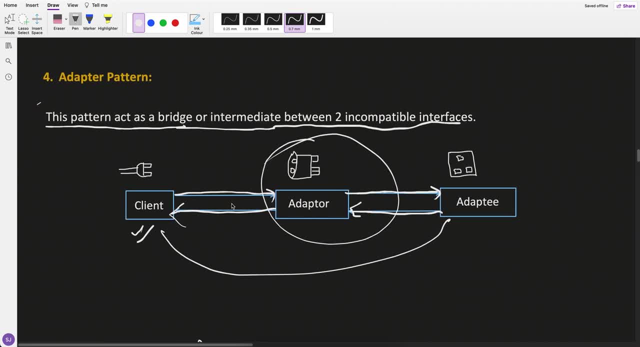 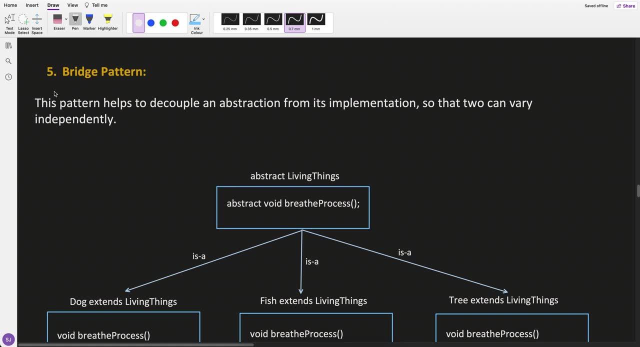 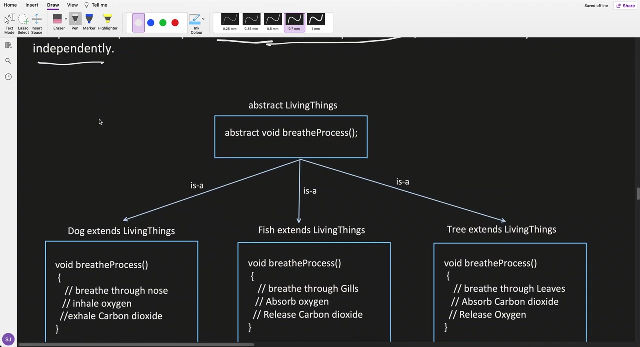 Okay, so it's become just a mediator, adapter pattern. Okay, Now another one we have is called bridge pattern. This patterns helps to decouple and abstract From its implementation so that two can vary independently. Let's understand this with an example. 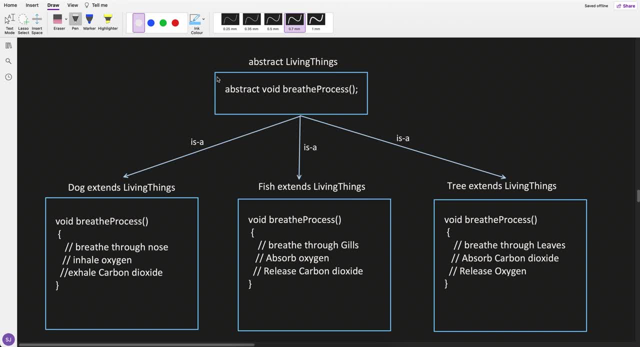 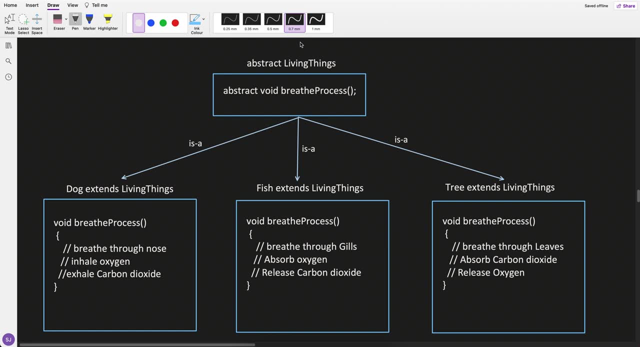 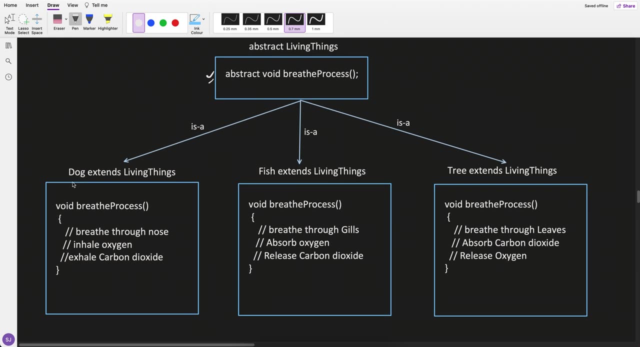 So I have taken an example of a living things. I have created one abstract class living thing and what one of the action which living thing do is breathing. So I have added one abstract method is breathe process And I have have three child classes of this living thing. 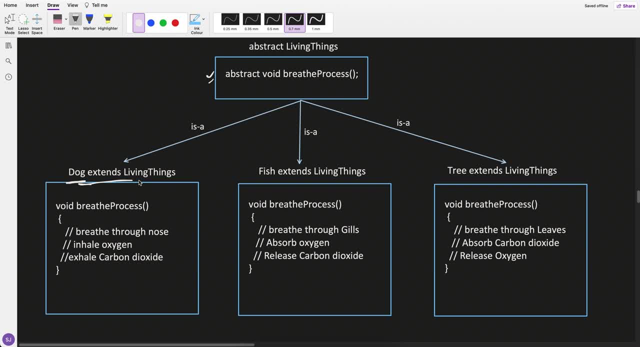 One is dog, Is a child of living thing, extends living thing. Another is fish, Another is tree. All three are living things and they are extending this living things abstract class. So all are implementing this breathe process And breathe processes: dog breathe through nose, inhale oxygen, exhale carbon dioxide. 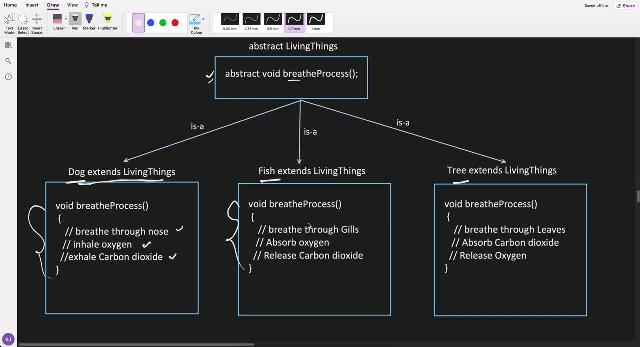 So this is a breathing process of a dog, Let's say. and the fish is: breathe through gills- absorb oxygen, release carbon dioxide. For tree, breathe through leaves- absorb carbon dioxide, release oxygen. So these are the different breathing process. But now let's say: 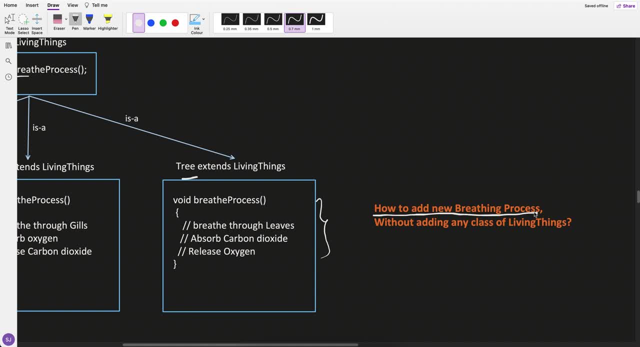 How you would add a new breathing process without adding any class of living thing. Now let's say I want to add another breathing process there. Let's say: breathe through. Let's say another way: like Nars are not cell right, So the the birds have nots right. 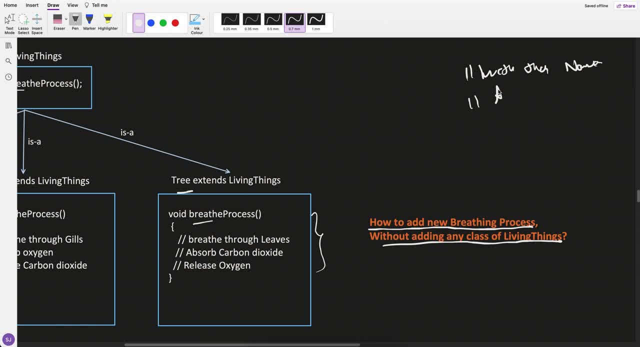 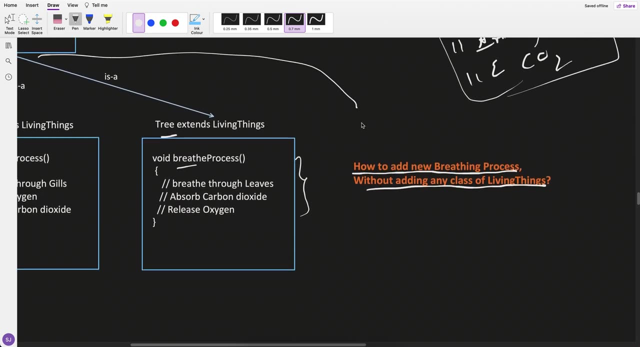 So be through nots And inhale Oxygen, exhale carbon dioxide. Okay, So this is another breathing process. Let's say how you would add it. So you have to first create Bird as this one and then add this Breathing process. 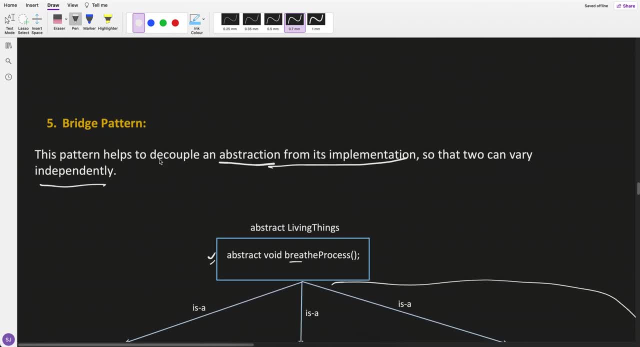 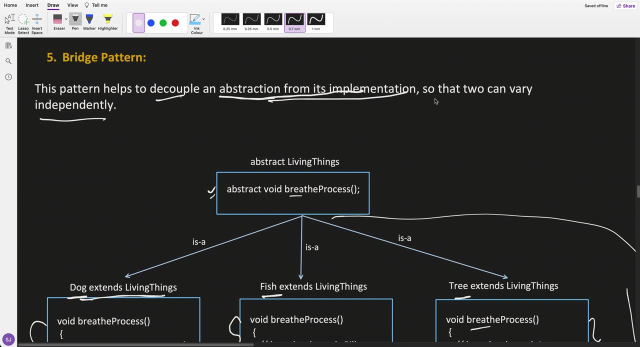 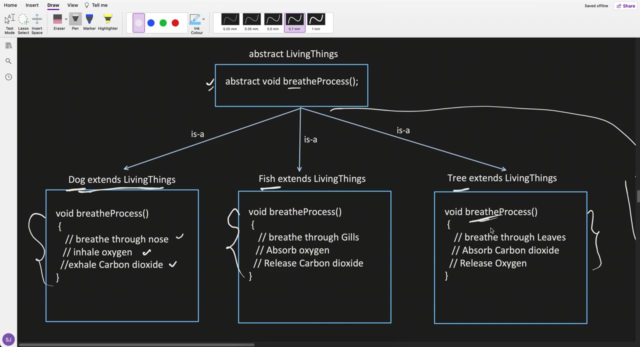 Breathing process here. So now here you see that it is very tightly coupled. So that's where bridge pattern, say that decouple and abstraction from its implementation, So that both can vary independently. Okay, So breathing process: Let's say this is an implementation. 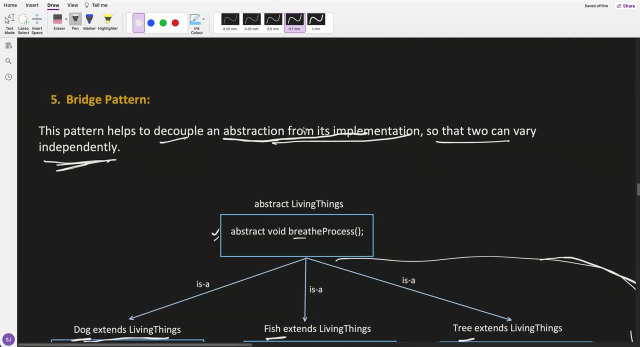 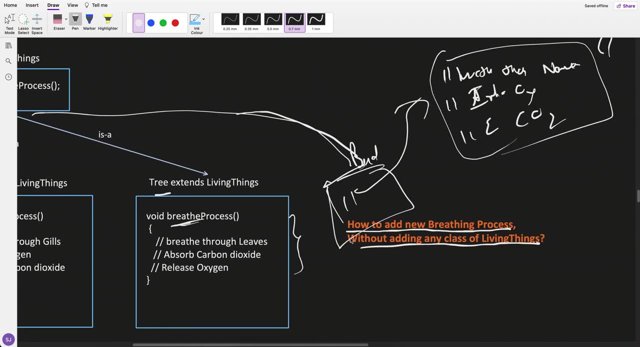 So currently it cannot, It cannot vary or it cannot increase Without Increasing that class. without adding that class, You can't add another new breathing process Until and unless there is no class which is using it. Okay, So that's where the bridge pattern say that decouple it and how to decouple it. 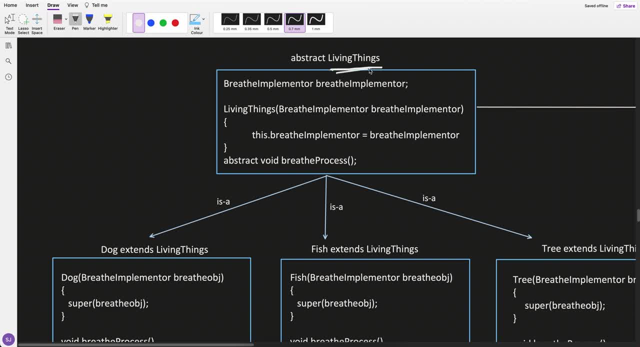 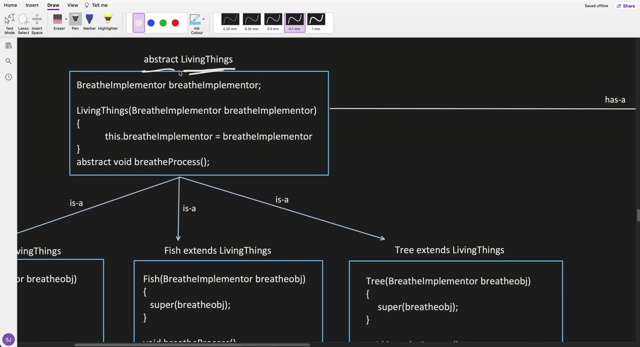 So here, if you see that Everything is same. But what I have done is I have added a breathe implementer. So again I have an abstract class living thing, Right? So just Just see that Living thing has one method called breathe process. 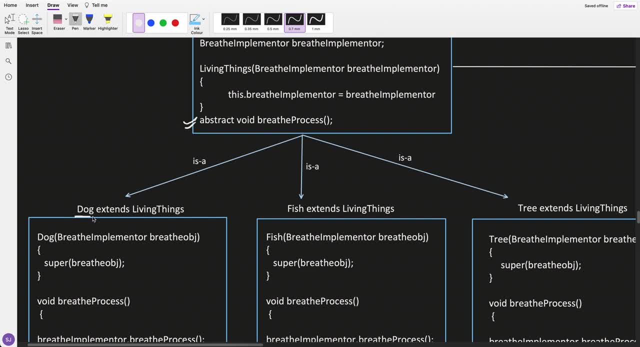 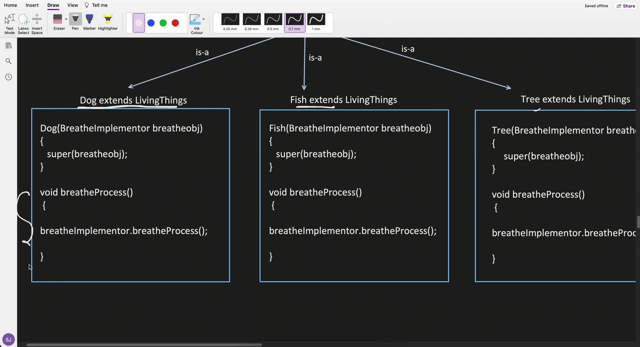 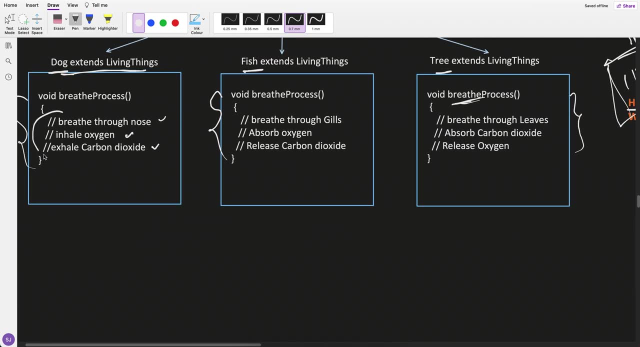 Same, Same dog is a child of this dog, Fish tree. Same three classes And the same methods breathe process they have implemented. But what is the difference now? So here, if you see that this logic Breathing process I have, 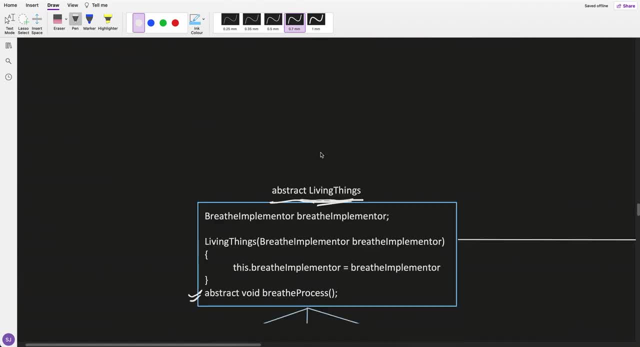 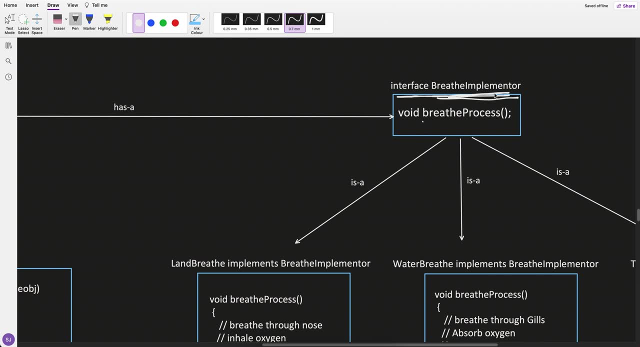 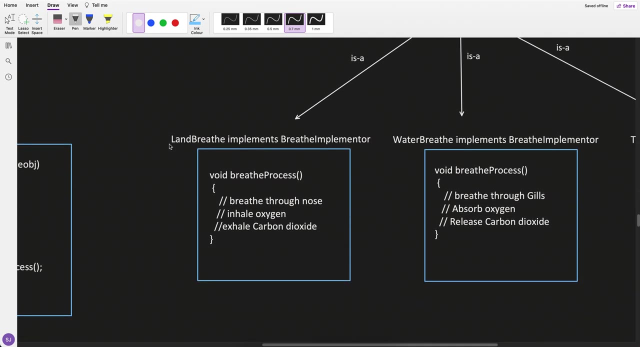 Taken out from this abstraction Right. So I have created one Breathe Implementer. I have created one breathing implementer interface breathe process. And what is that? one of the breathe processes, like land breathe, Which is a child of this one. 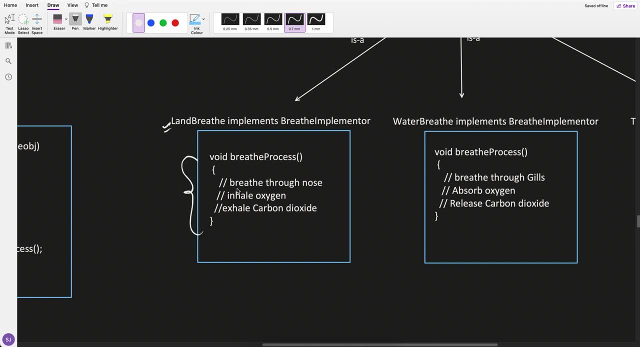 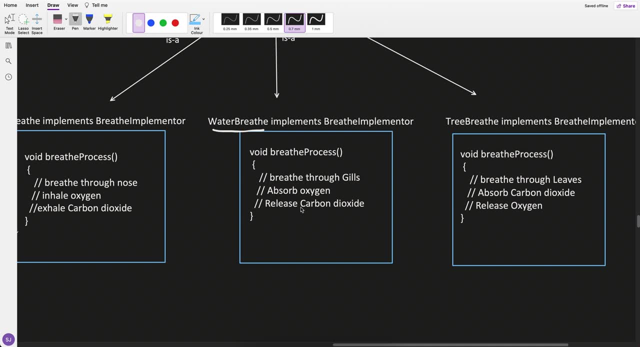 So here in the land, breathe. Breathe through nose, Inhale oxygen, Exhale carbon dioxide. Water breathe, class. Breathe through gills: Absorb oxygen, Release carbon dioxide. Tree breathe. Breathe through lips. 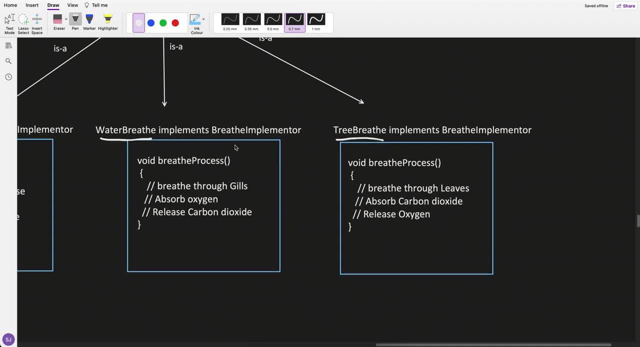 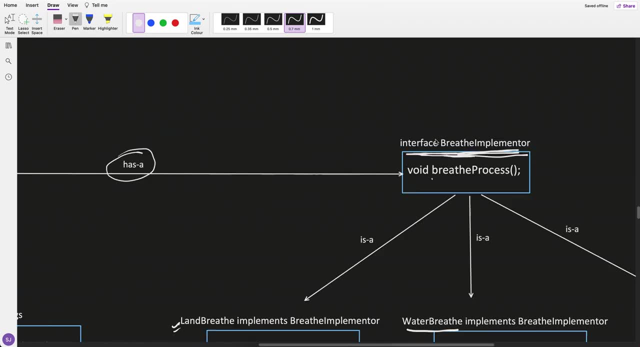 Absorb carbon dioxide, Release oxygen. So now Here, This living thing has Breathe implementer, So it has Breathe implementer. This is just a constructor To where child, Whichever they wanted, They can set this. 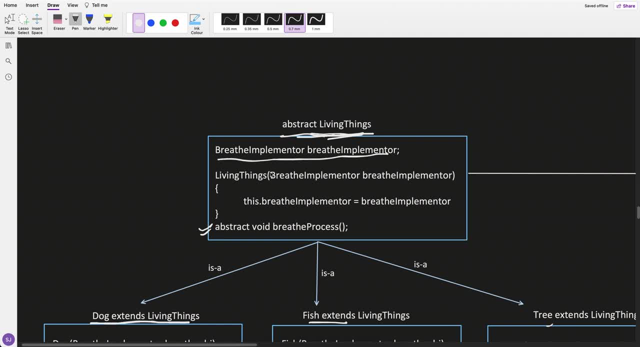 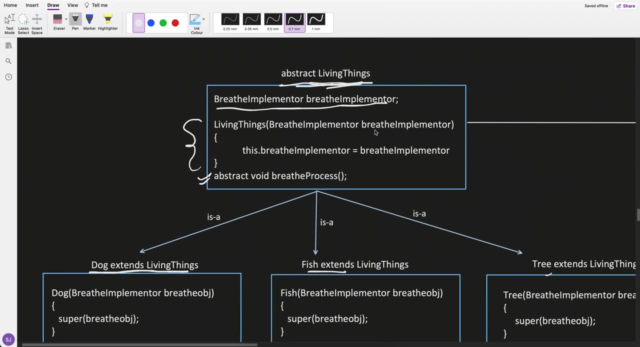 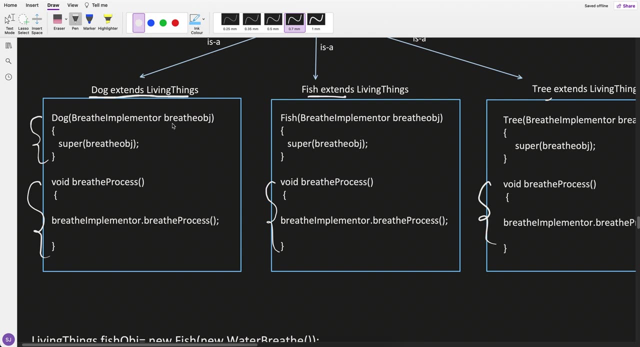 Breathe implementer. So the dog Here, This is the Constructor, And This is the Dog Here, This is the Dog Here, This is the Dog Here, This is the Constructor, And. 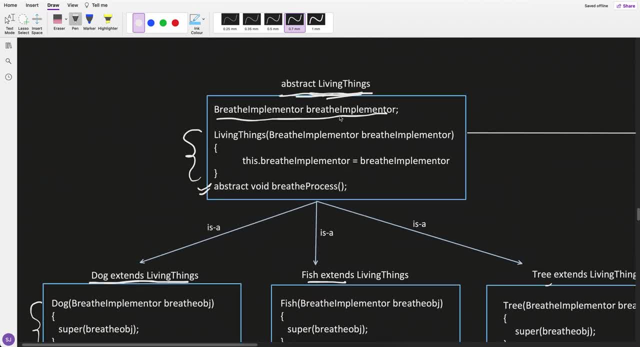 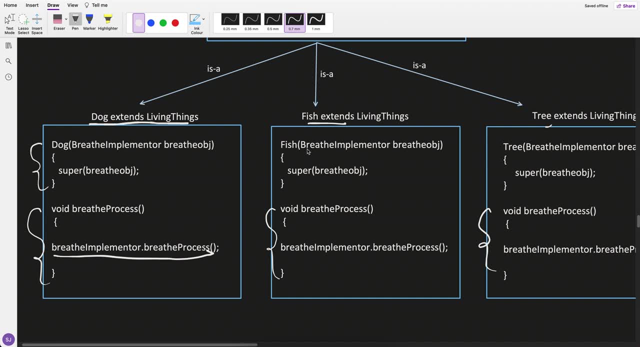 During the client. Whatever the Breathe implementer Would be passed, It will get set Here And It will call This Breathe process. Similarly, In the fish I am using This Breathe implementer. 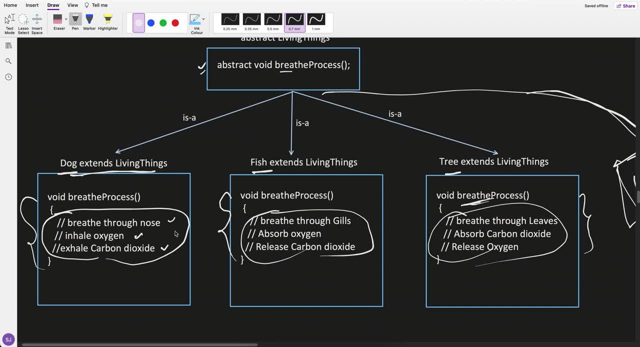 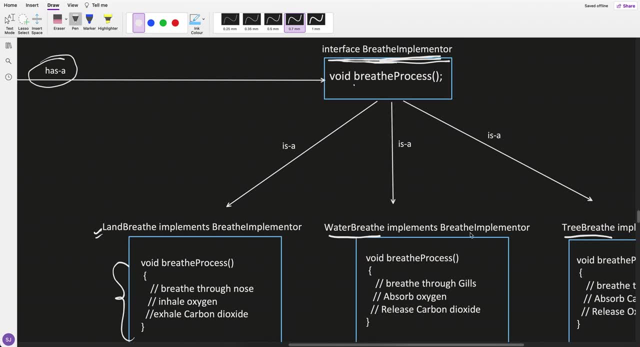 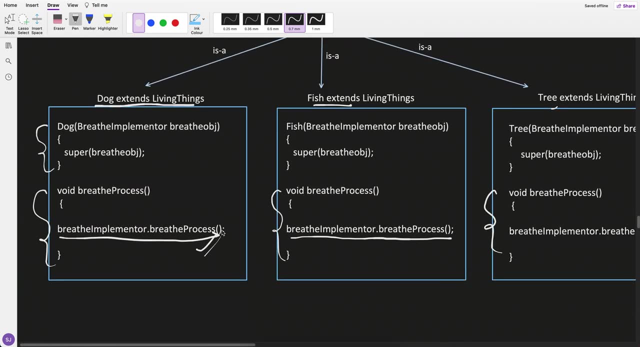 And call the Breathe process. So one thing You should notice: Now I have removed This logic Out of This class, Put into an Another Interface, And Now It Has This And 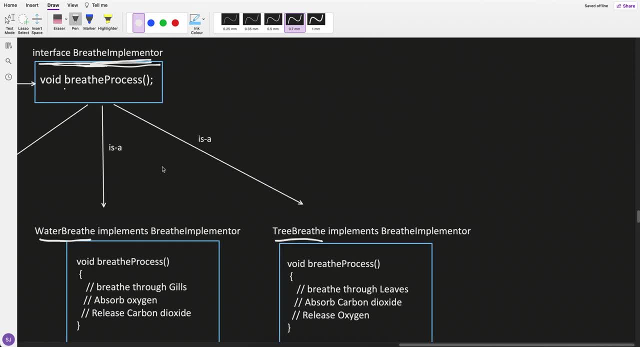 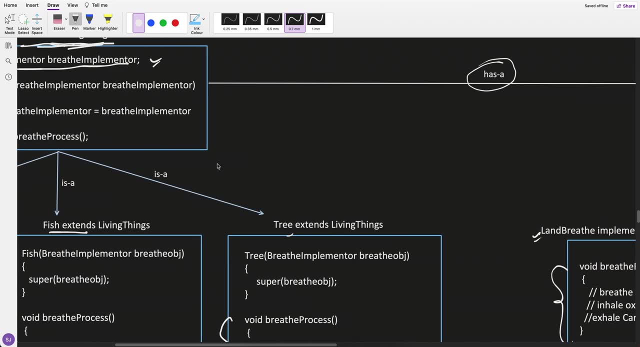 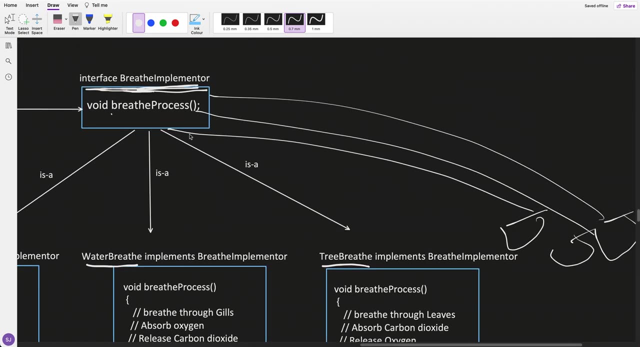 Calling That One. Now, What Will Happen Now? Let's Say, If I Want To Add More Breathe Process, I Can Add It Simply Independently. 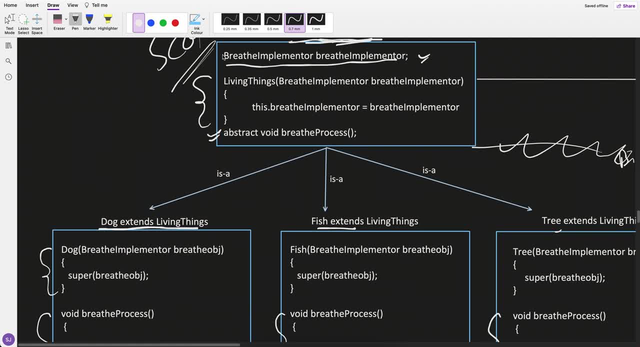 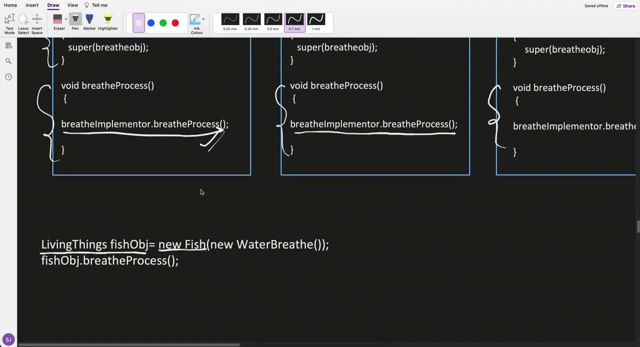 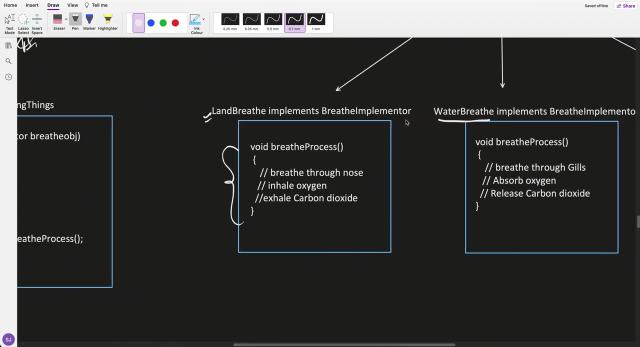 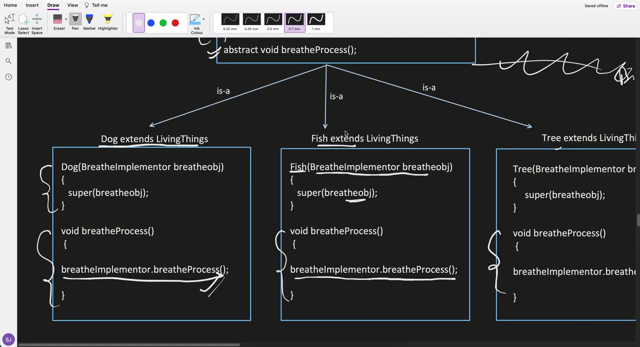 So I Have Decoupled It, Okay. So Just Take This Example. I Am Creating A Living Thing- Fish Object. So I Am Creating A New. 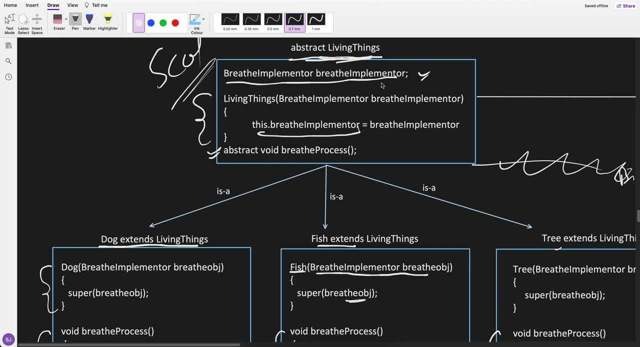 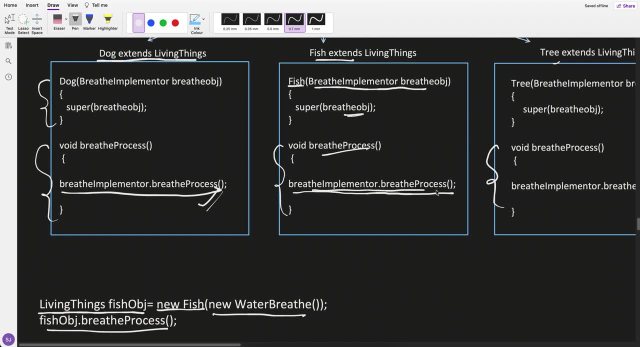 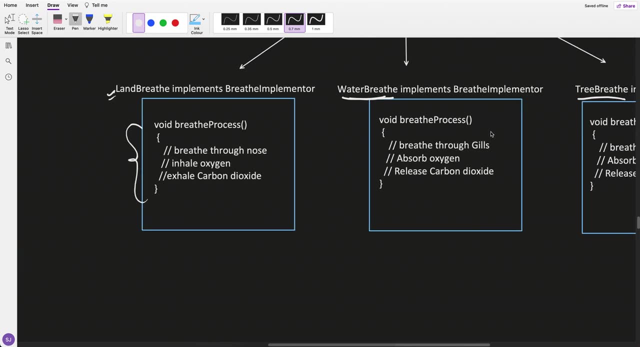 Fish, New Fish Object. Now I Am Calling Fish Object Breathe Process. So In The Breathe Process, Breathe Implementer Dot Breathe. 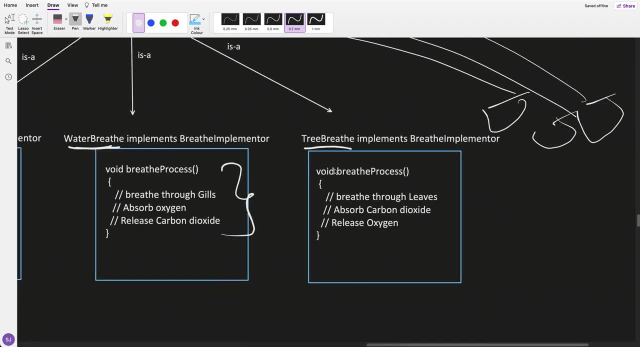 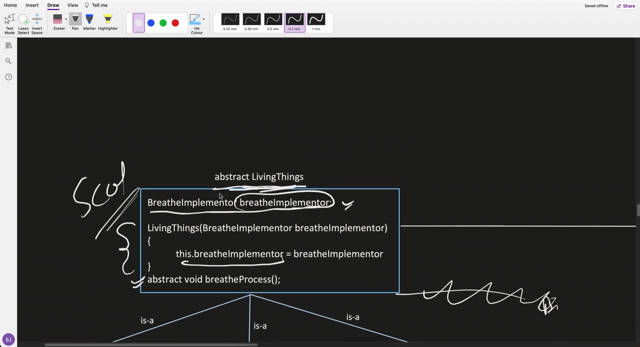 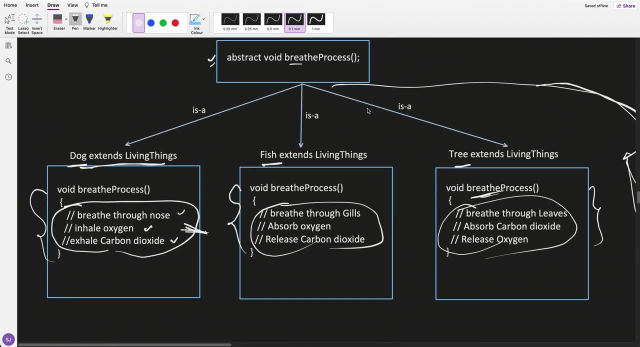 Process. So What Is The Implementer? We Said: Water Breathe One To Grow. It Can Grow Independently Without Even Worry About This Class. 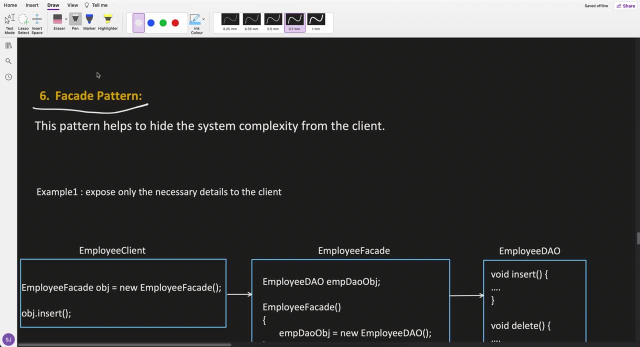 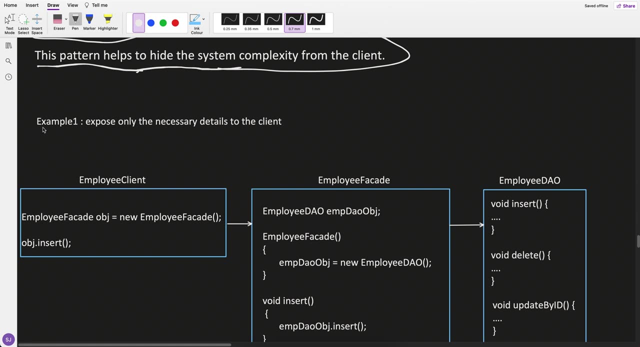 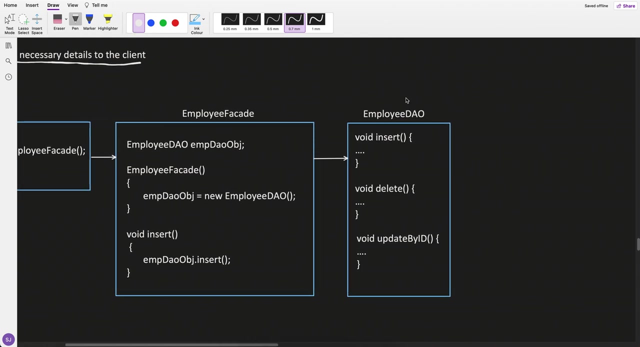 Okay, So That Is What Known As Bridge Pattern. So Another We Have Is Facade Pattern. So The Two Example, Let's Say This Example One: 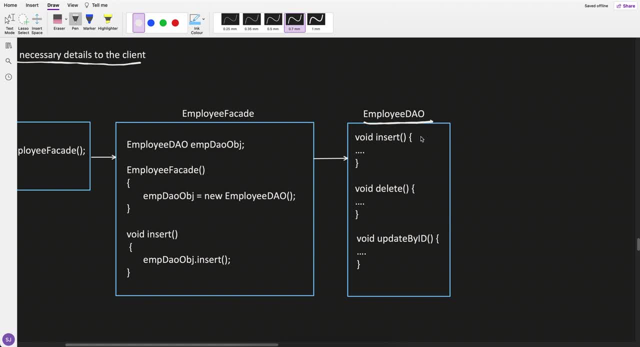 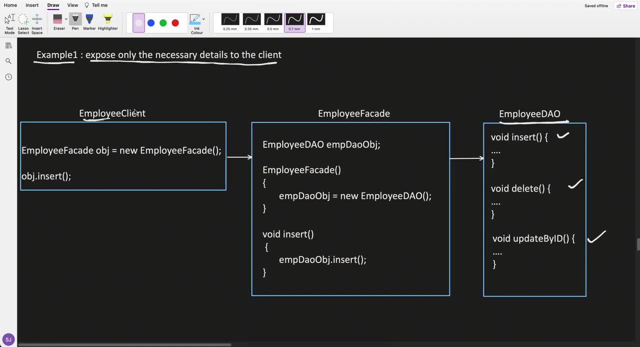 Expose Only The Necessary Details To The Client. So Assume This. I Have One Class Employee, Dow. I Have Three Methods. How Can I Do? 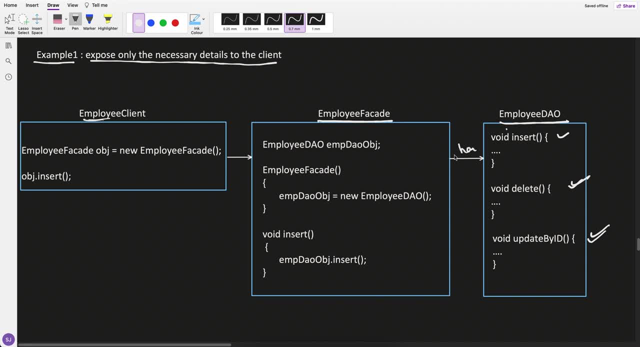 The. I Can Use Employee Facade In The Mid. So Employee Facade Has Your Dow And Use This Constructor To Initialize It, And It Only. 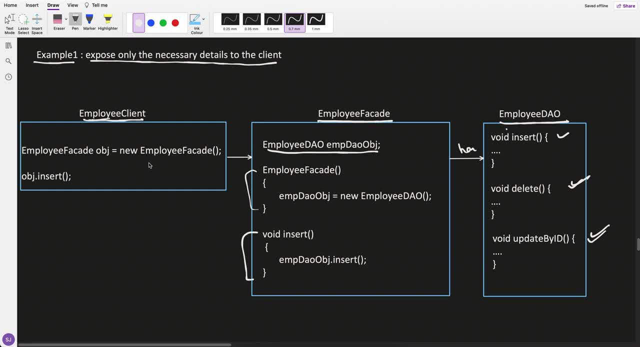 It Will Add Extra Overhead To The Client. So We Wanted To Make Client Very Like: Don't Have Only Exposed Things, Which Is Required. 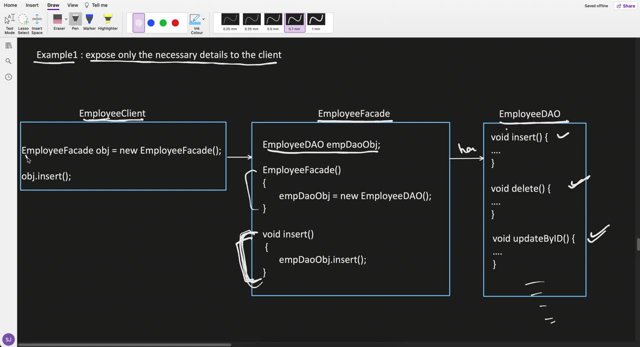 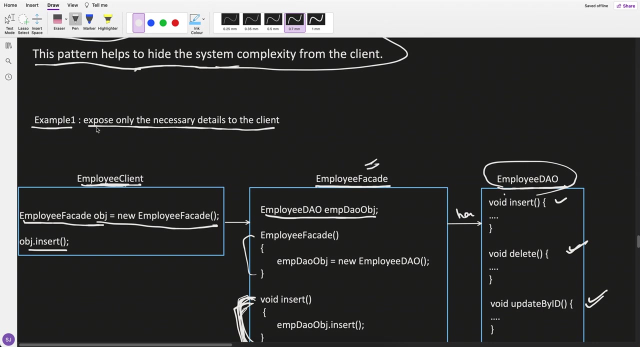 Right, So Here Facade Can And Call The Insert. Okay. So Here, If You See That This Employee Client For This Employee Client Only Insert, 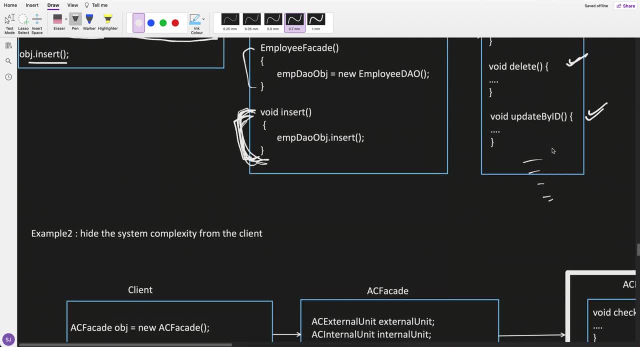 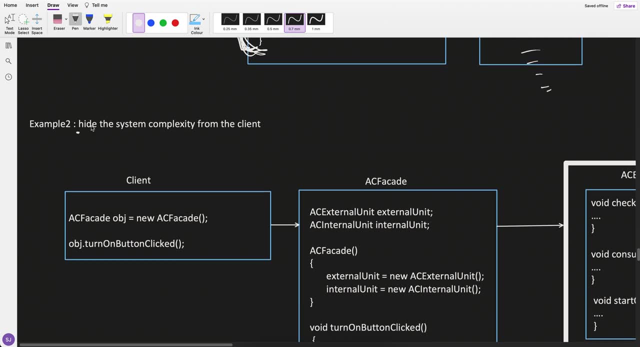 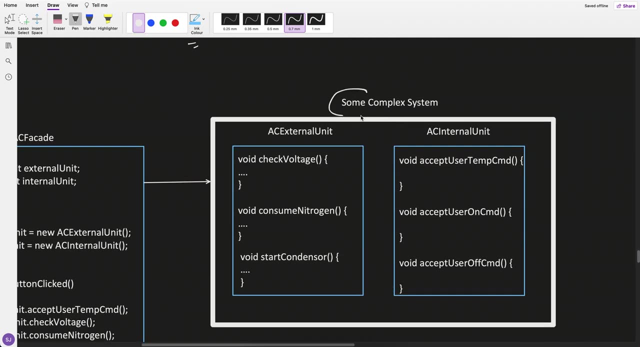 Is Insert Method Is Exist, It Don't Have To Use The Facade. So, For Example, What Is The Facade Can Be Used. Hide The 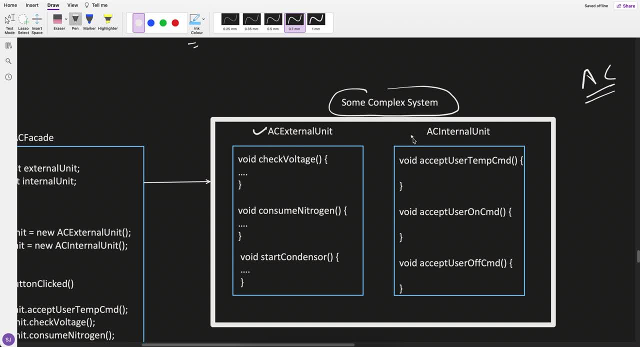 System Complexity From The Client. How For Example: This Is A Very, Very Complex System, So If Client Has To Perform A Particular Operation There, 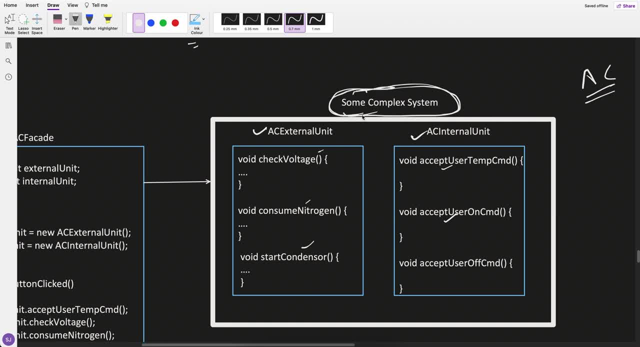 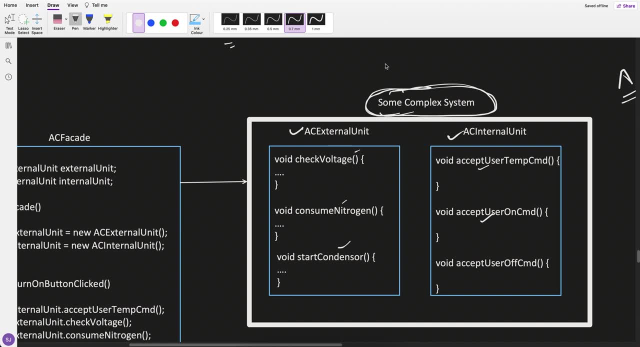 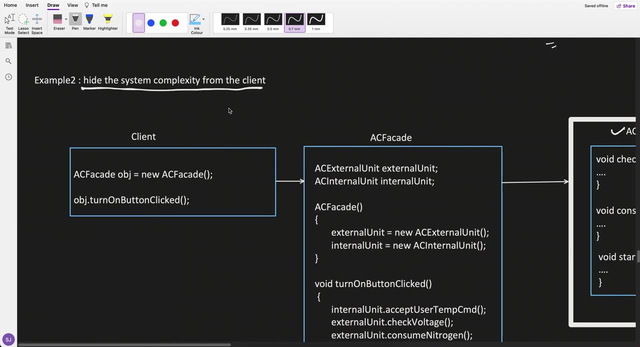 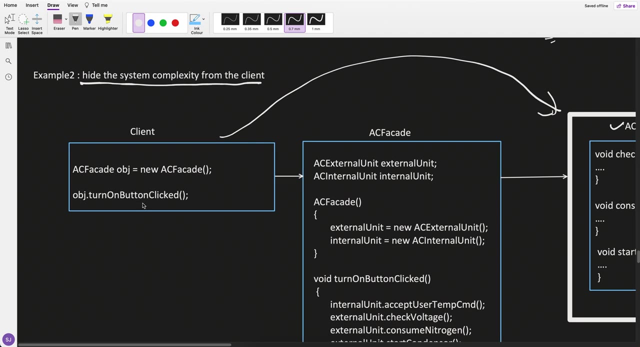 Could Be A Sequence Of Steps You Have To Perform In A Multiple Classes, So If Client Has To Directly Contact With This Complex System, 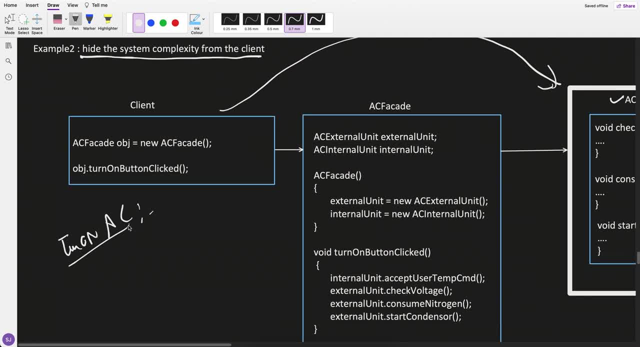 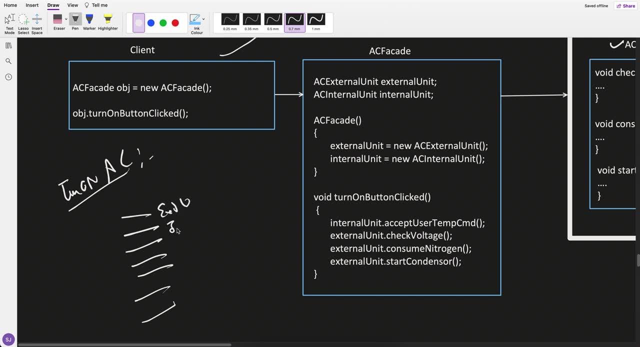 And Let's Say It Has To Turn On The A C, Then There Might Be. It Has To Perform Several Steps Of Any Update, Any 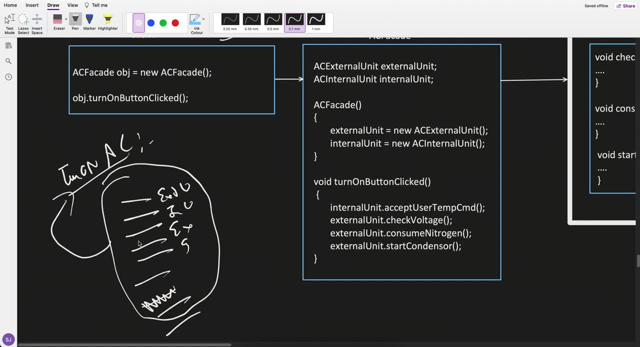 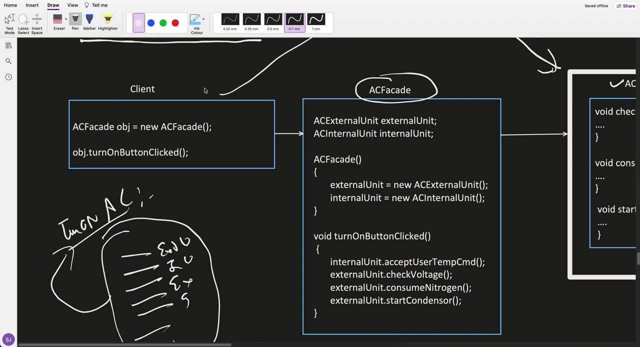 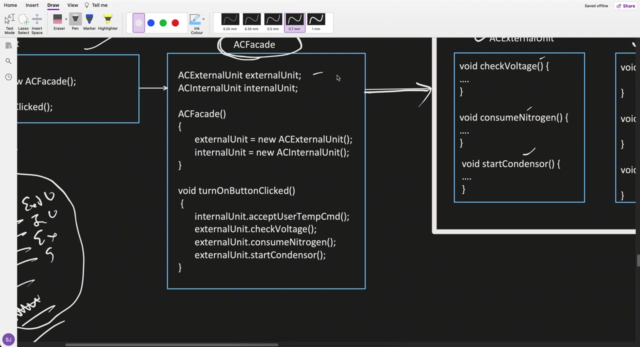 Of This Step Got Removed Or Any Of This Step Got Added New, The Client Will Break. Client Has To Change It. So What Facade? 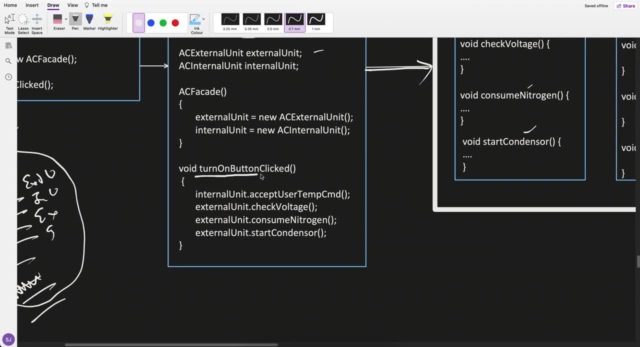 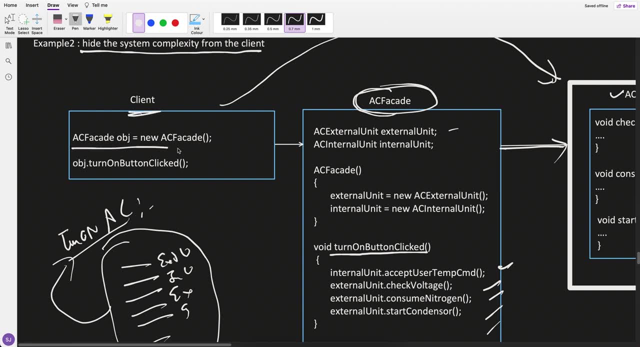 With Whenever Turn On Button Has Been Clicked, It Will Do All The Steps Which Is Required To Turn On The A, C For The 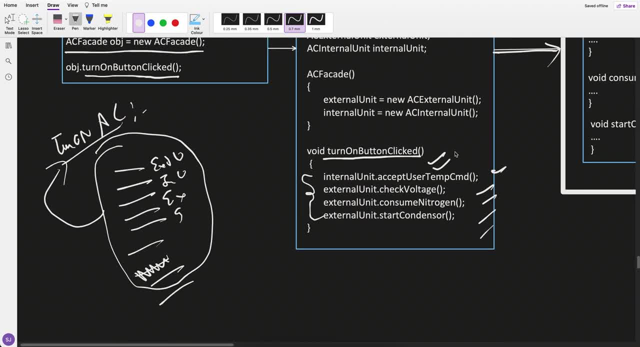 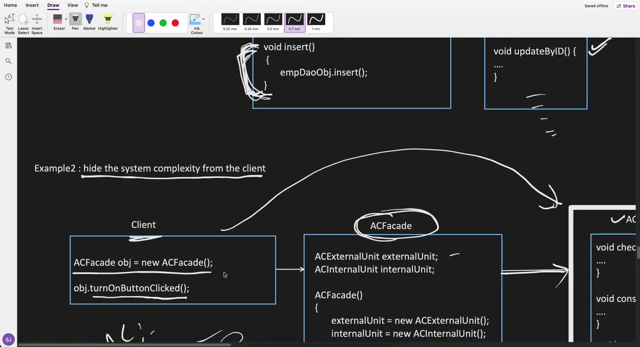 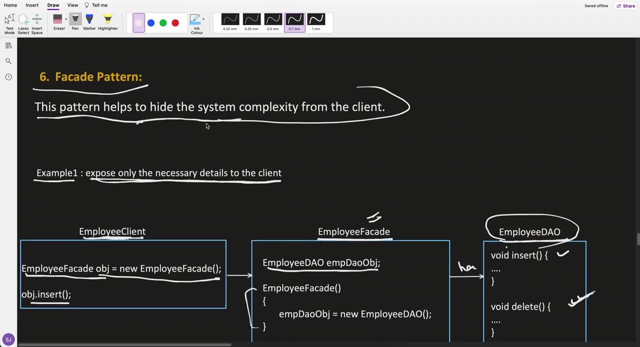 Client Interact With The Facade. If There Are Too Many Clients, No Client Will Get Impacted. Okay, So You Got It Right. What Is? 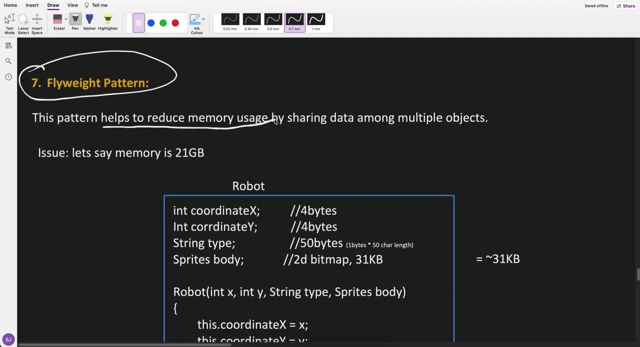 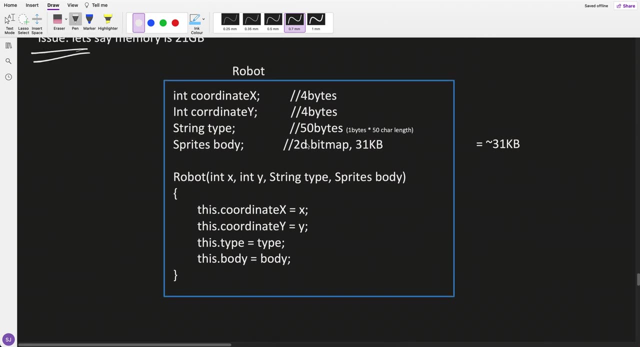 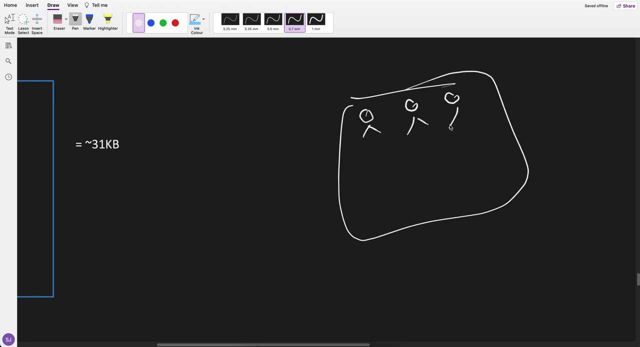 The Use Of The Facade It Used To Help Hide, To Reduce The Memory Usage. Let's Understand With An Example. What Is The Issue? Which? 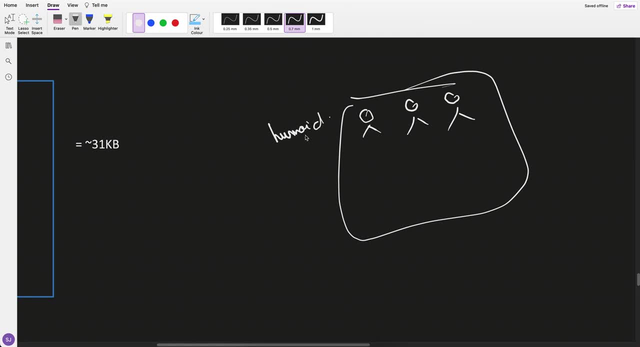 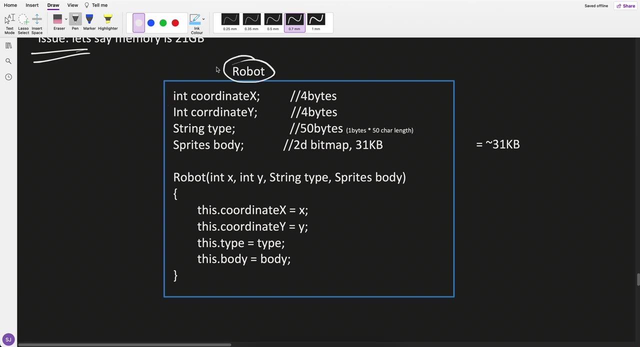 Is Flyweight, Is Trying To Start. Let's Say, I'm Building A Game And In That I Have Created One Robot Class And I Have 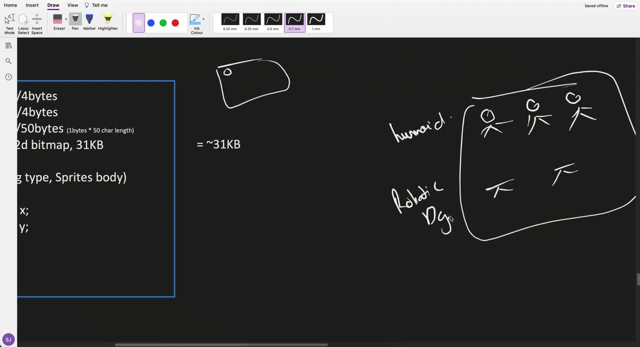 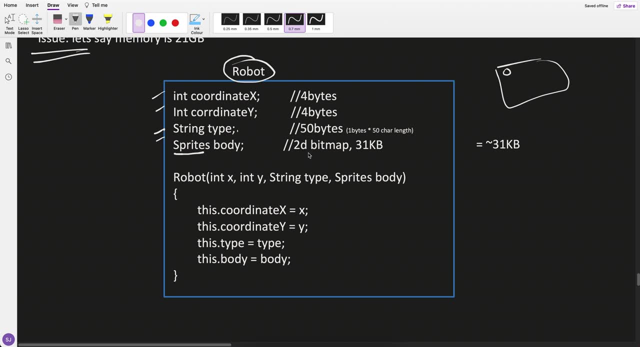 Like X, X's, Y, X's In The Screen Where To Display That Robot Type Of A Robot, Maybe Two D. You Can Say That It's. 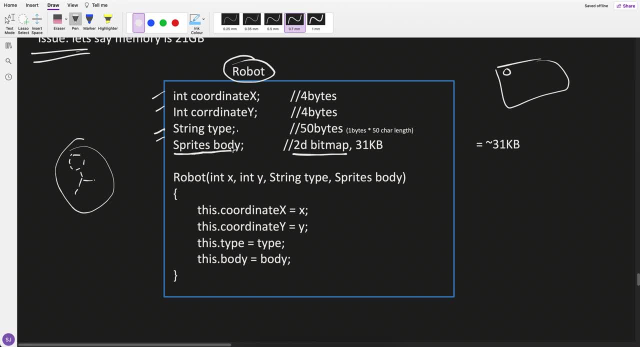 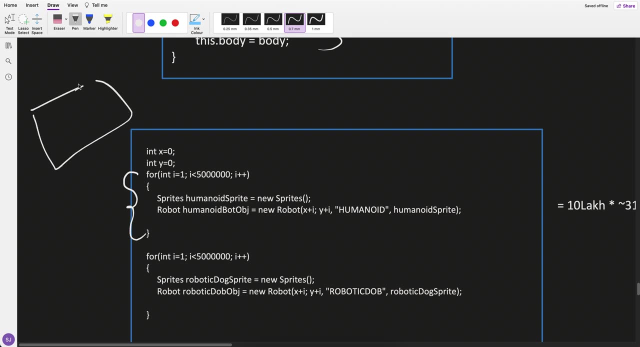 A Bitmap Which Is Used To Render The Image. Okay, So I Have One Sprite For This Type. So Now In The Screen I Have 5.. 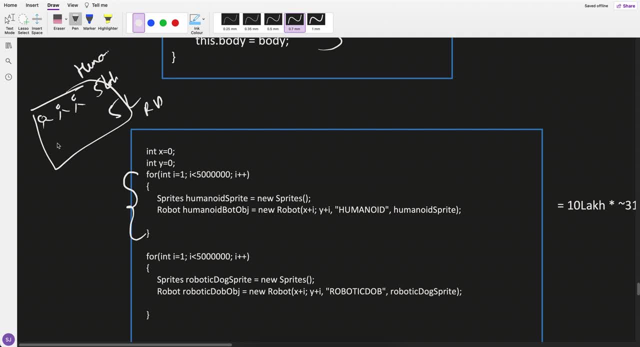 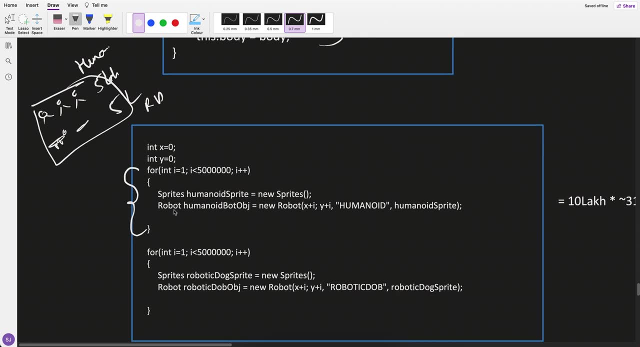 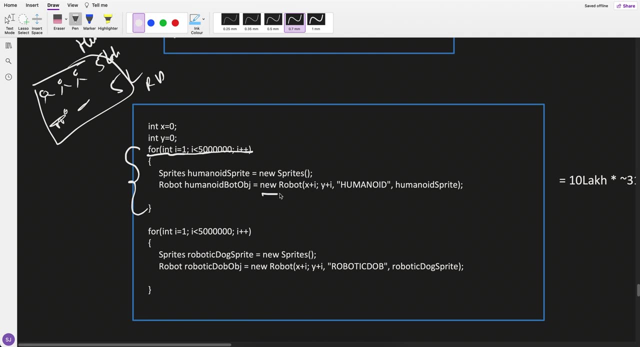 Lakh Humanites And 5. Lakh Robotic Dogs. Robotic Dogs, Right? So Maybe Robotic Dogs. I Have To Create So Many, So Here. 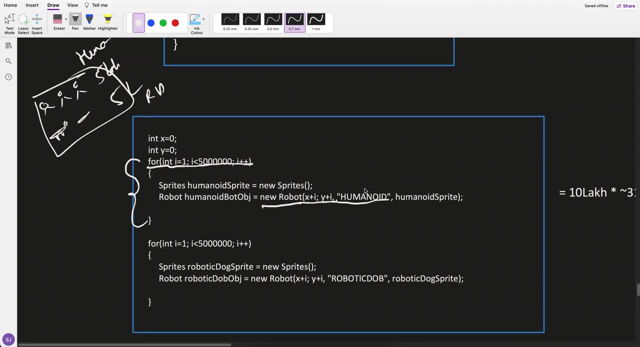 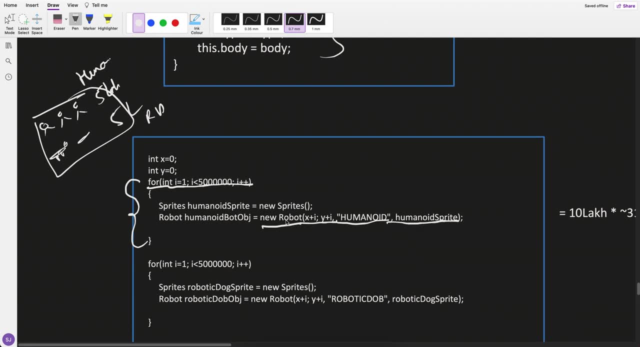 What I'm Creating: A Humanite. I Wanted To Create A Humanite Type And I Pass The Humanite Sprite, So Let's Assume That This 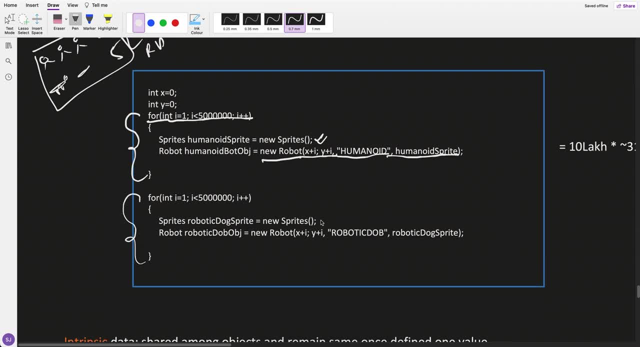 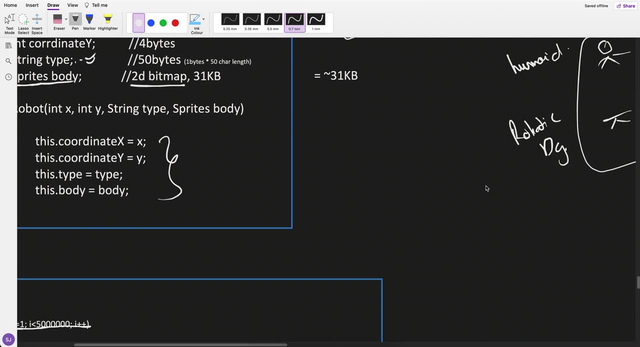 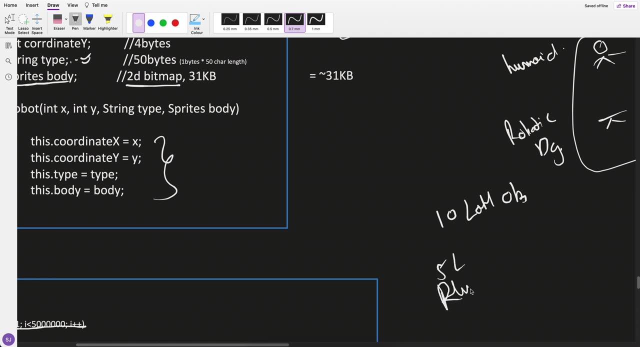 Is A Object Which Has The Graphic Rendering Information. A Now I Am Total. I Am Creating 10. Lakh Objects, 5. Lakh Robotic. 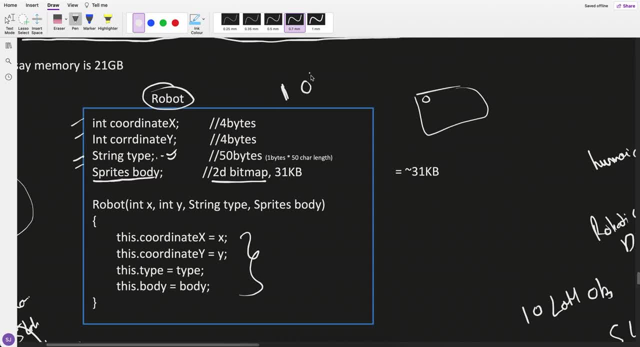 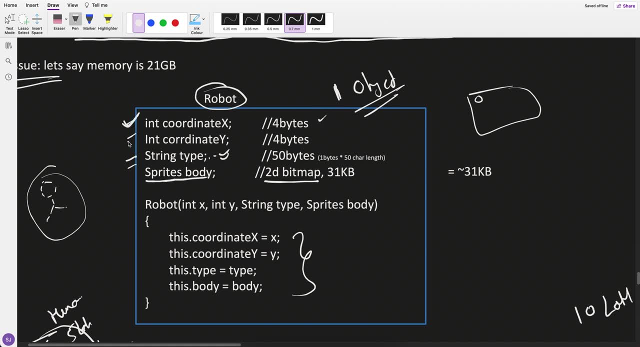 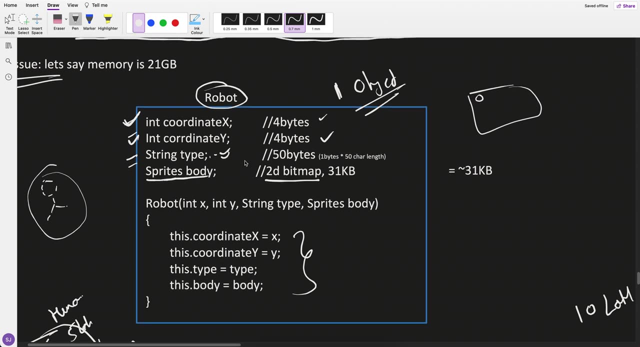 Humanites, Human Robots And 5. Lakh Robotic Dogs, Right Total 10. Lakh Now, But One Character. One Character Is One Byte, So Let's. 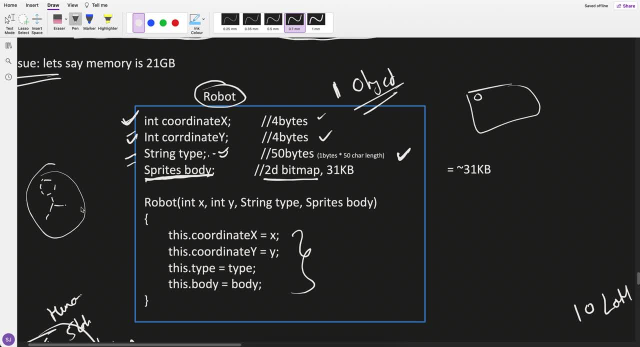 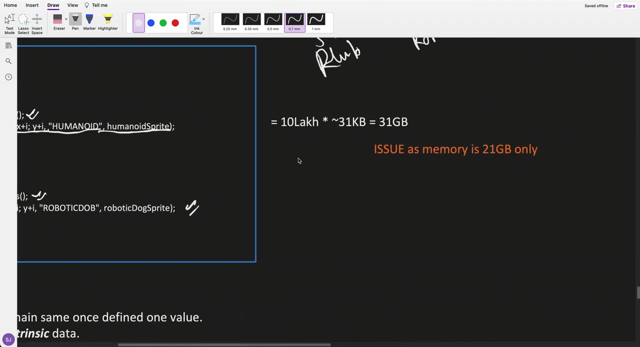 Say It Is 50. Bytes And Sprites Body. So This Is One, Let's Say, Heavy Object Where We Are Rendering 2. G, B, Let's. 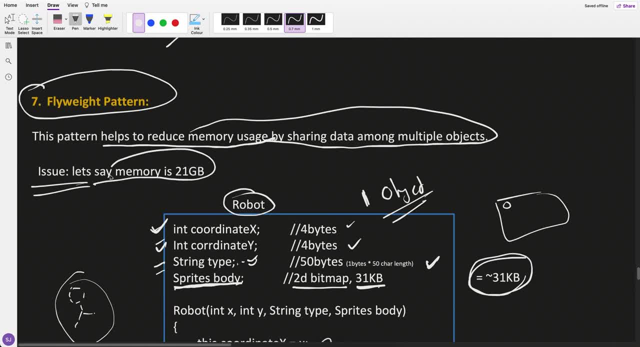 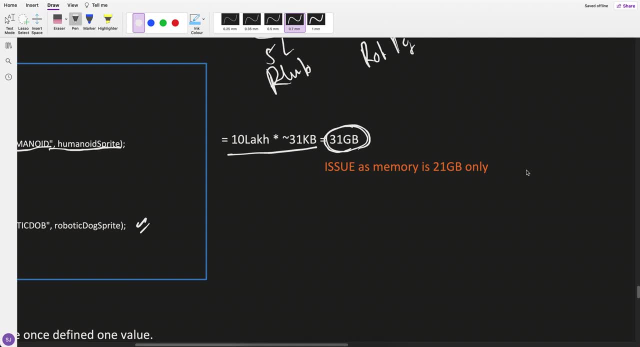 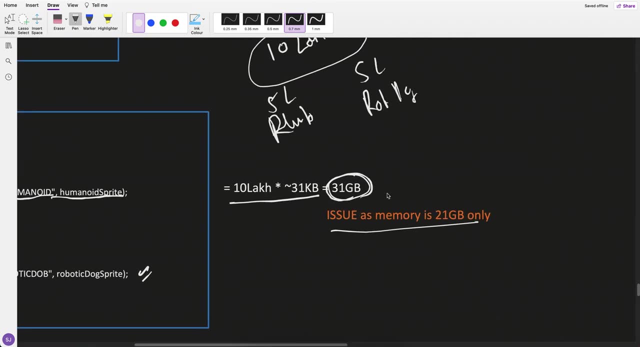 Say: But We, Let's Say We Have Only 21.. G B Memory And We Are Creating So Many Objects, Which Is Almost Consuming 31.. 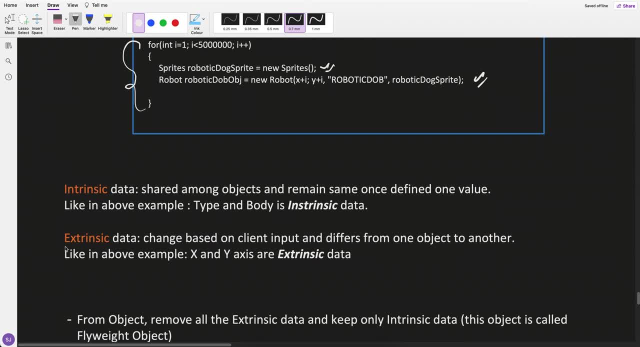 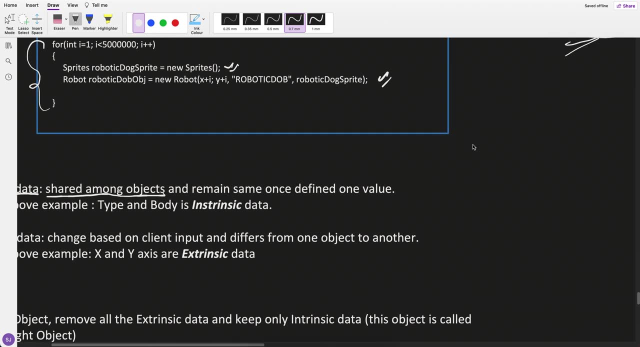 G B, How It Has 2. Parts. One Thing You Have To Look At Is Instinct Data. What Is Instinct Data? Instinct Data Is: 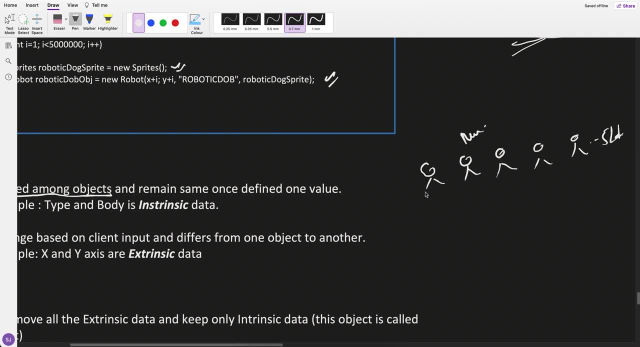 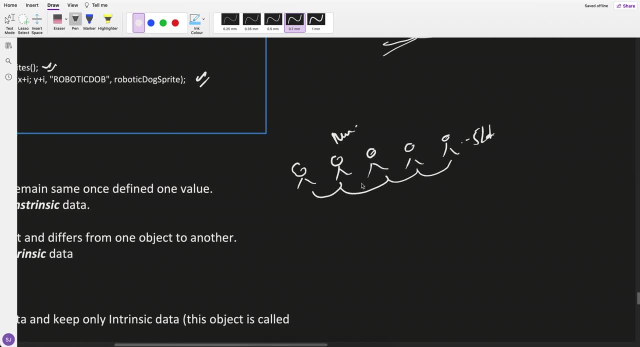 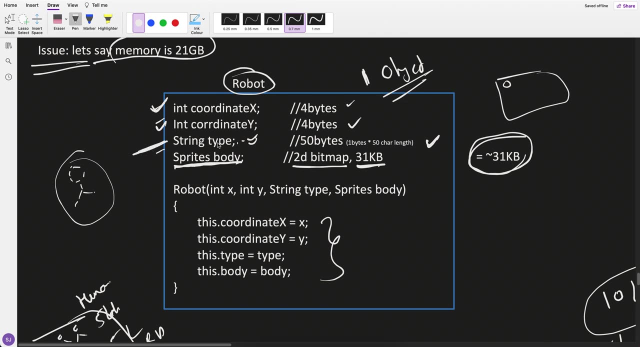 Shared Among Objects, So Look For Any Shared Among All Of This. Is There Any Shared Data? Yes, There Is Shared Data, So All Are Human. 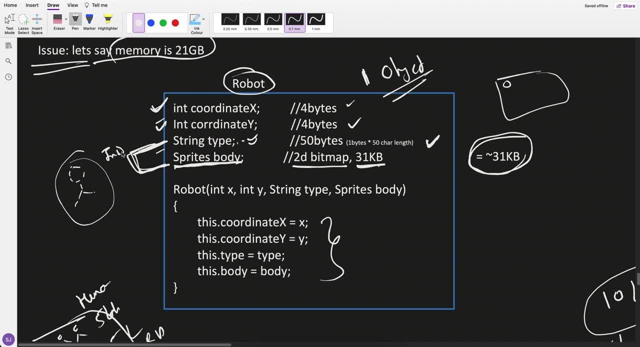 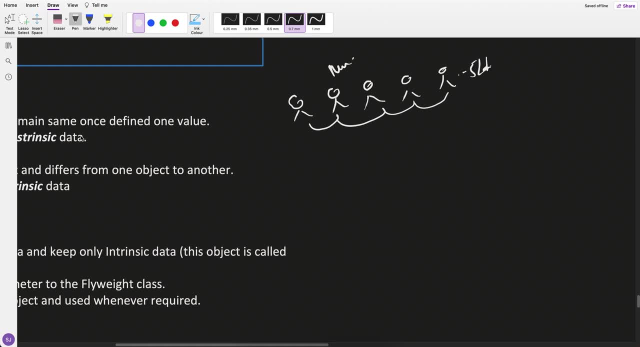 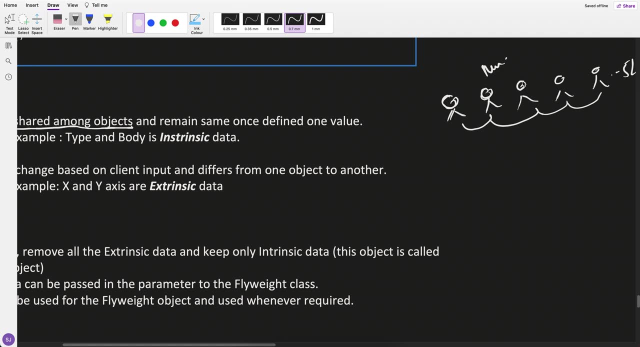 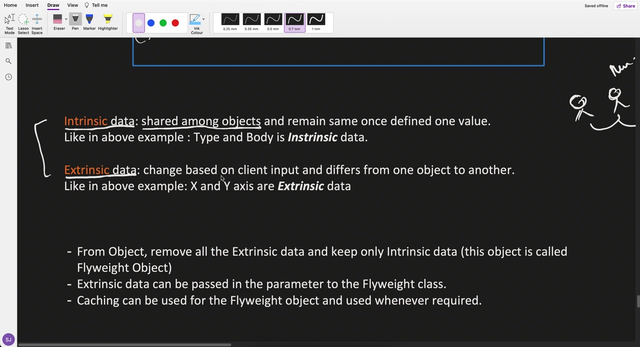 So Their Type Is Same And Their 2D Rendering Is, And Once They Are Defined They Will Remain The Same Once They Are, Whatever The 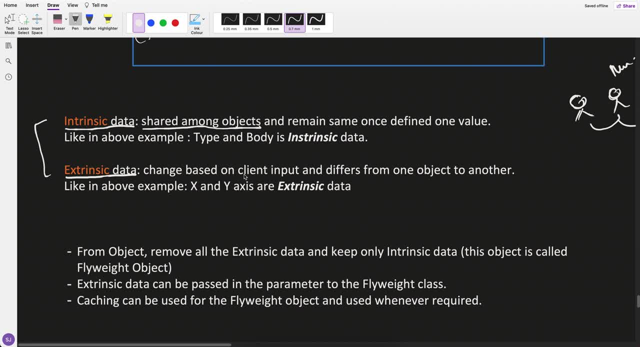 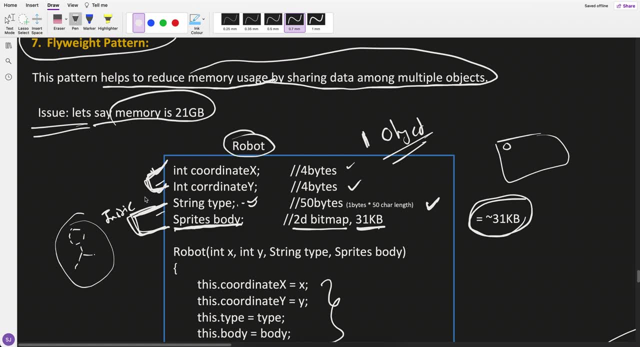 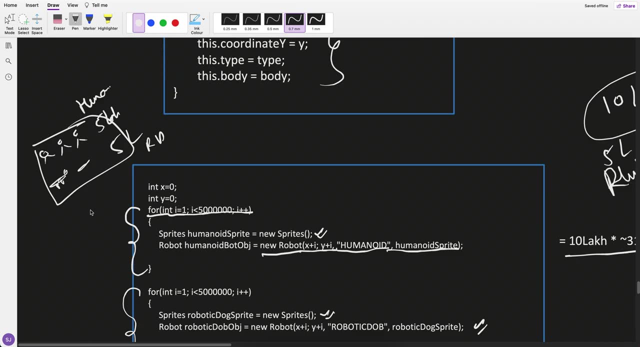 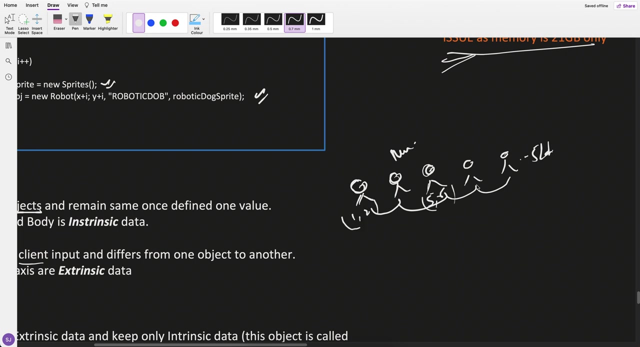 Value Is Defined At Once, Their Value Doesn't Change. Actually, They Always Look Same. So This Is A Strict Data Right. So This Will Change. 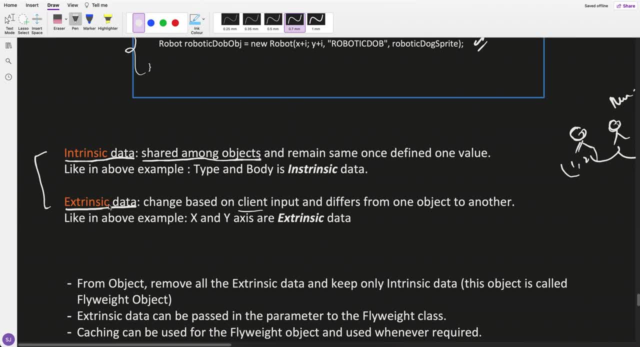 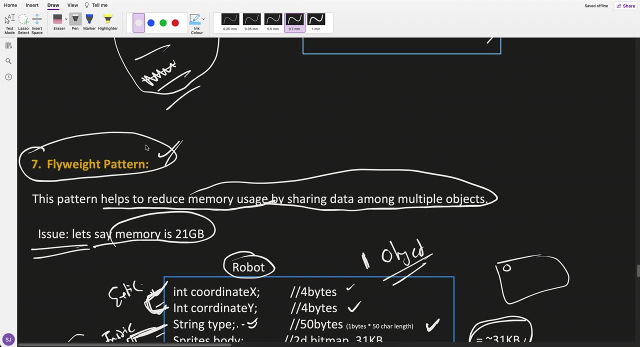 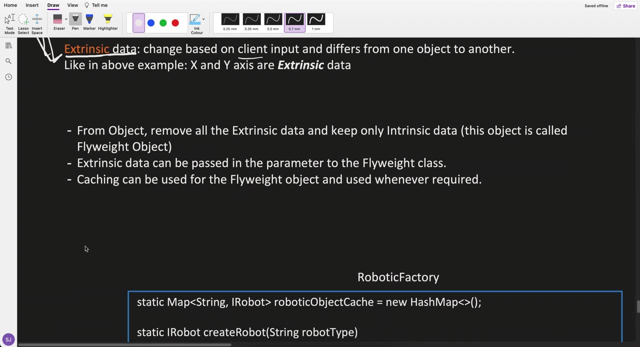 For Every Object. So Maybe This Object Is Placed At One Comma, Two Xs, This Can Be Placed To That. So Let's See. 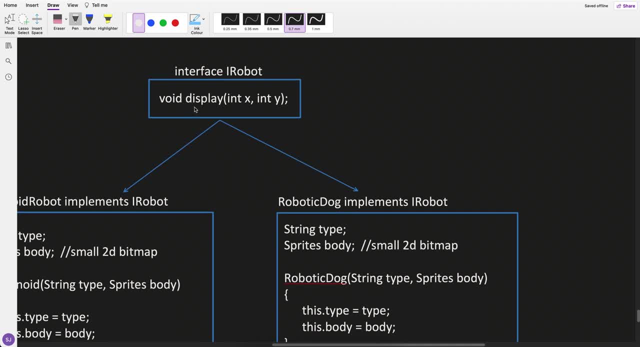 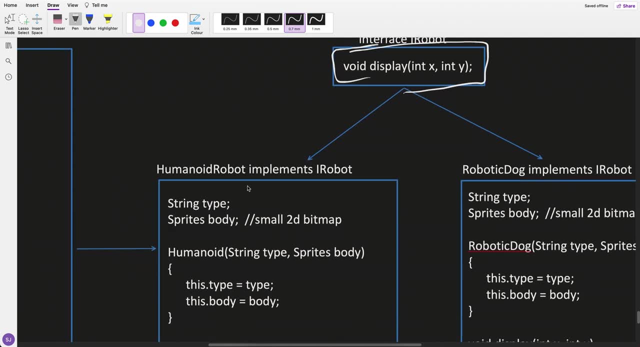 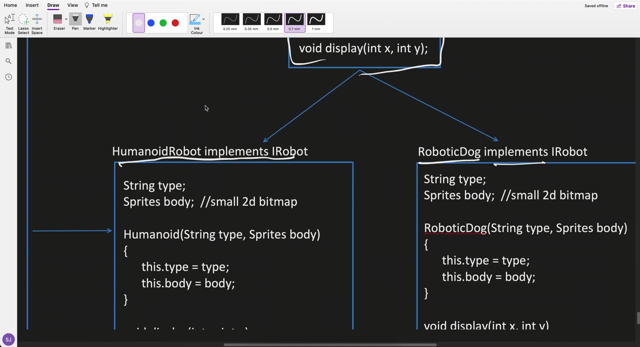 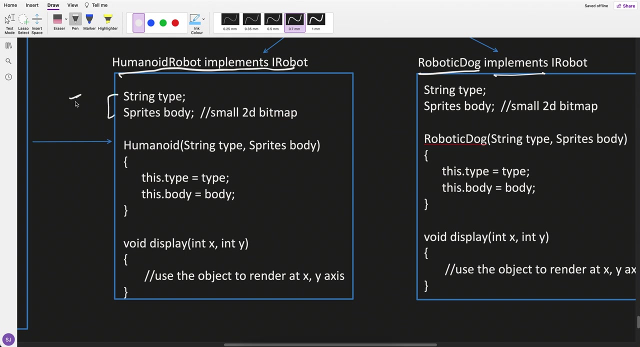 This An Example, So I Have Modified The Previous Class. Like I Have Created An Interface Robot, I Wanted To Create A Two Type And Instinct. 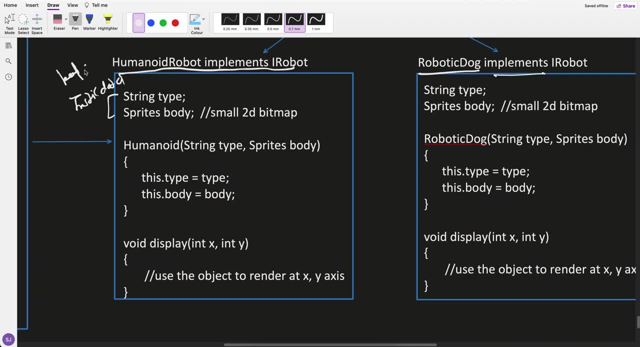 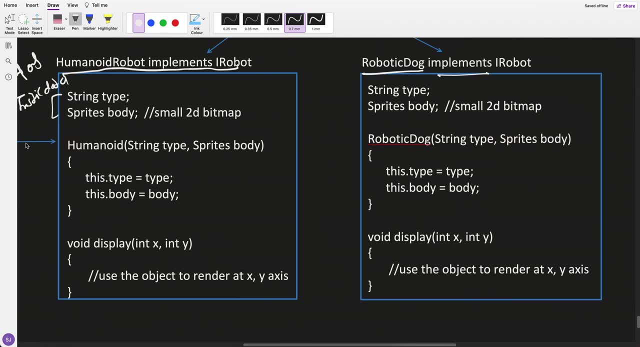 Data. Keep Only Instinct Data. What Is Instinct Data? Properties Which Are Shared Among Different Objects. Okay, So Type And Body Is Something Which Was. 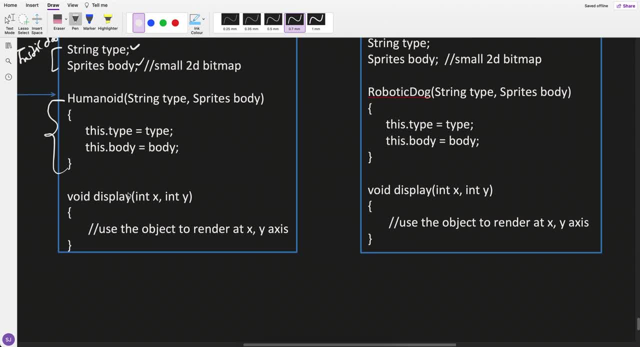 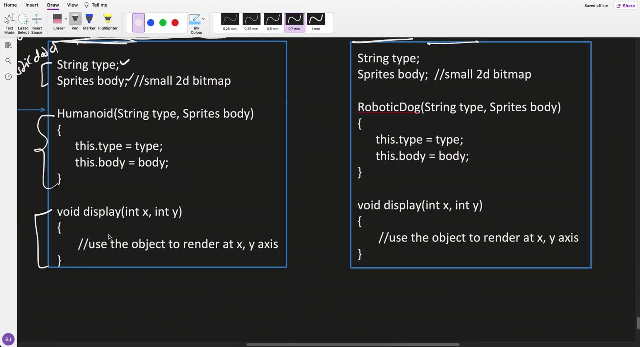 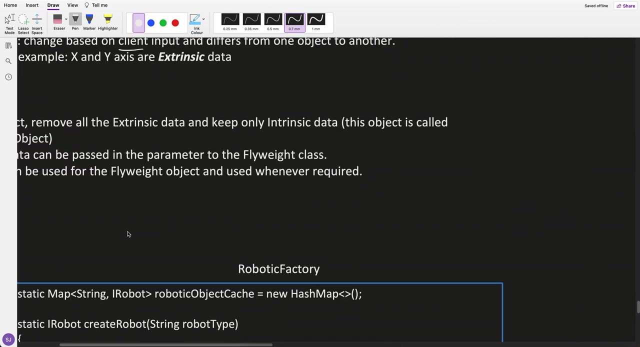 Same For Those. And The Display Method Right And Now Display Method. And Where To Display X Xs And Y Xs Right. So Now Two. 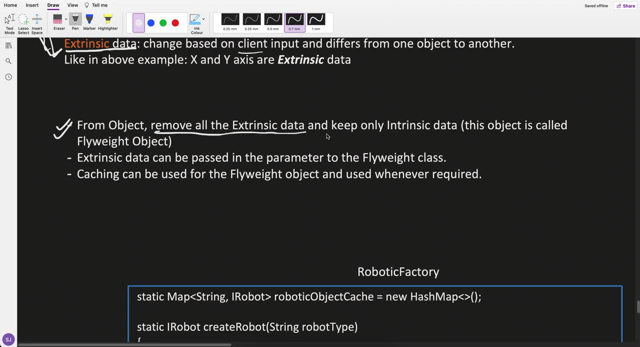 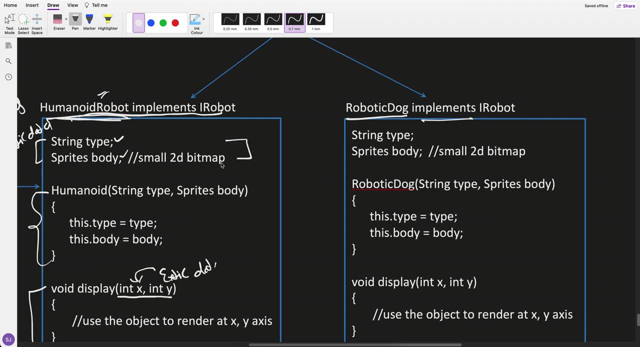 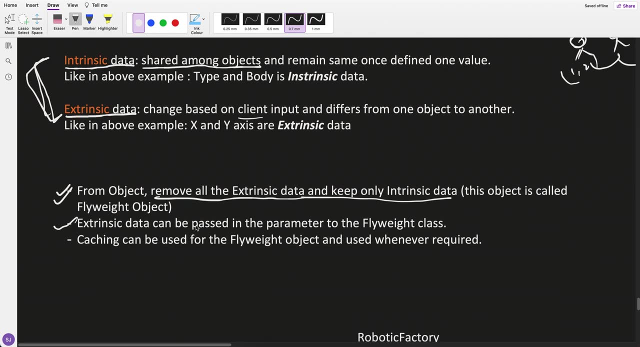 Things Which We Have Been Instinct Data. So From The Robotic Object I Have Only Kept The Instinct Data. I Have Removed All The. 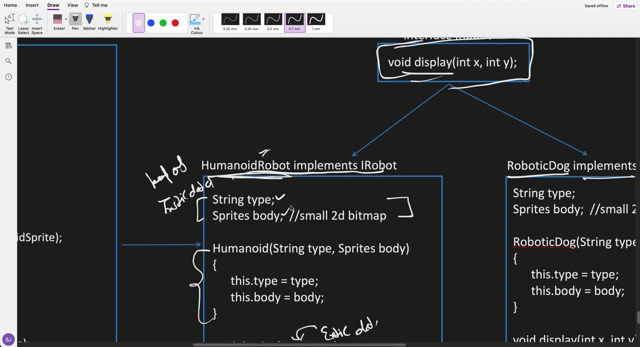 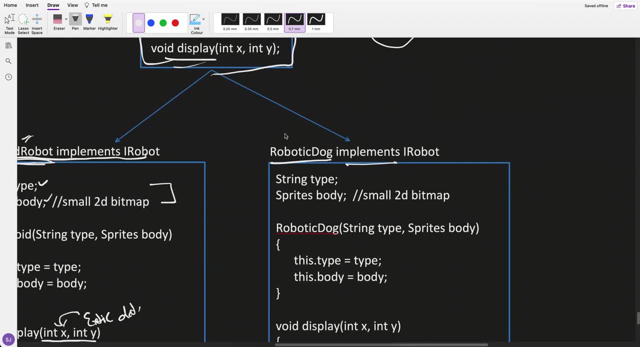 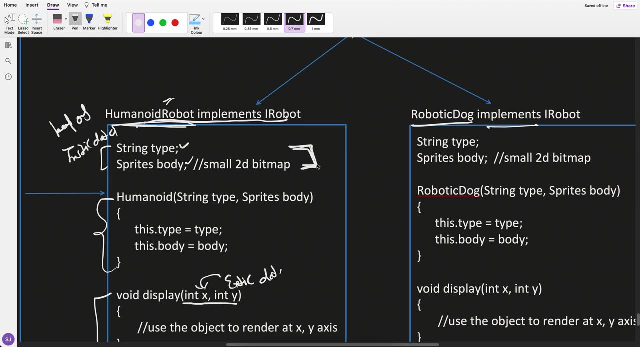 Extinct Data And Whatever The Extinct Data Is, You Have That. Create Your Class As A Flyweight Class In The Flyweight Class You Have. 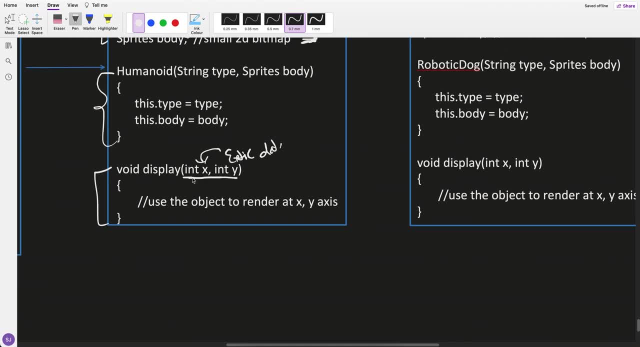 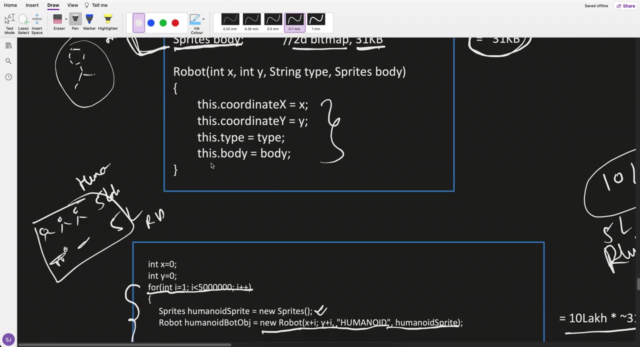 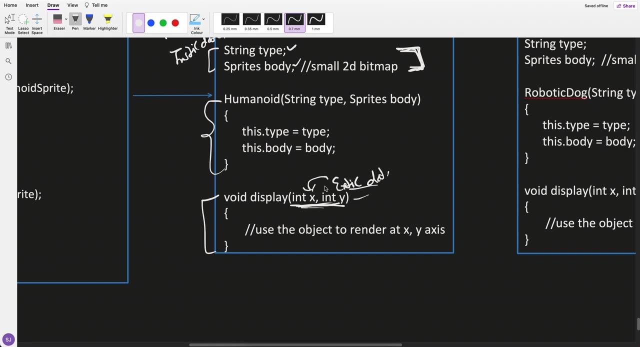 Only Instinct Objects, Instinct Properties And Wherever You Want A String Properties Or The Properties Which Was Required. I Have Put The Pass The. 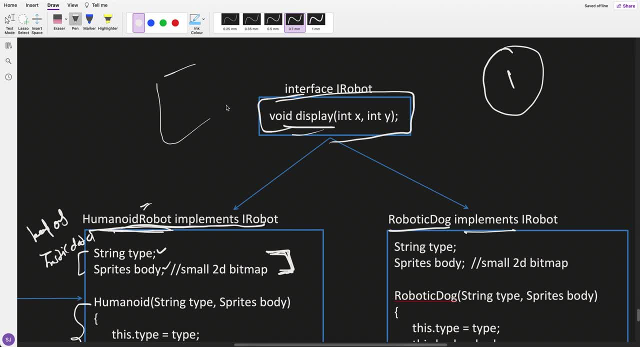 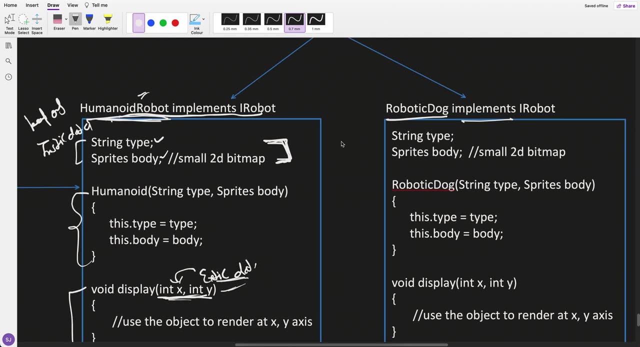 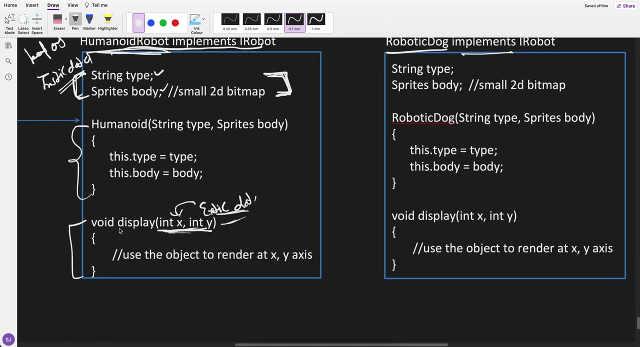 Parameter As All The Extinct Data. Similarly I Have Done For Robotic Dog Also. Okay, So I Have. So Just In The Class: Robot Class. 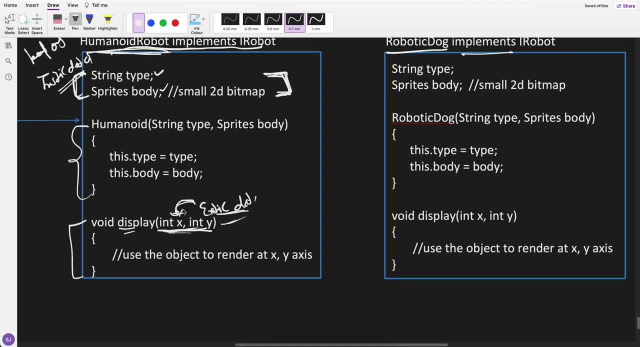 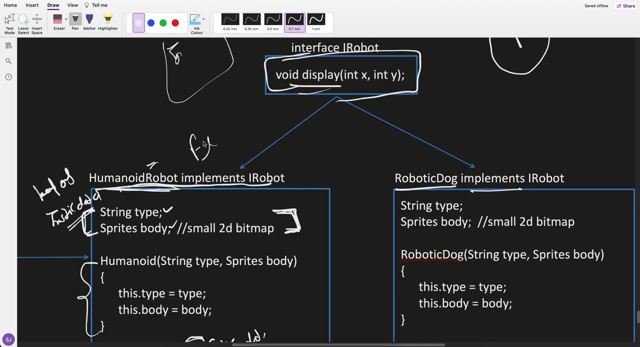 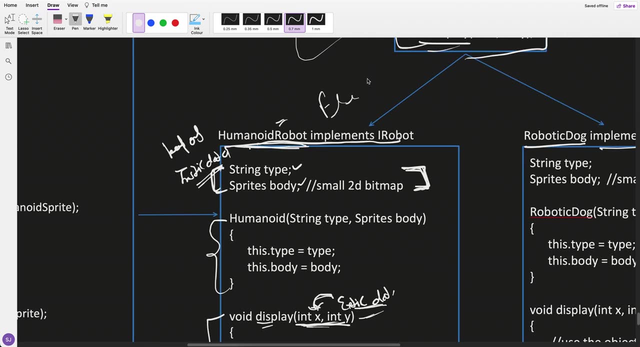 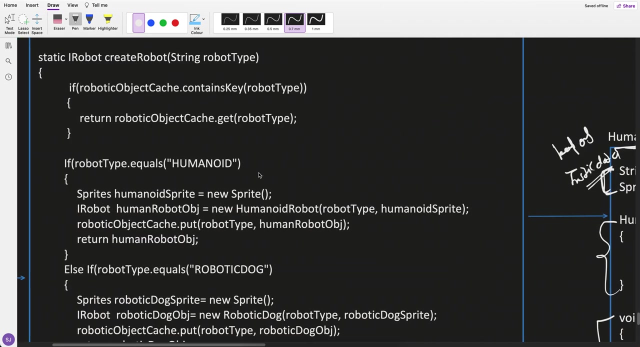 Now We Have Only Instinct Data And The Method Which Have To Work On The Extinct Data. We Have To Pass It Through Parameter. So 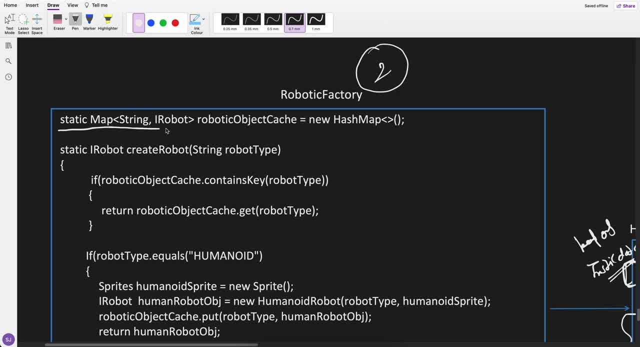 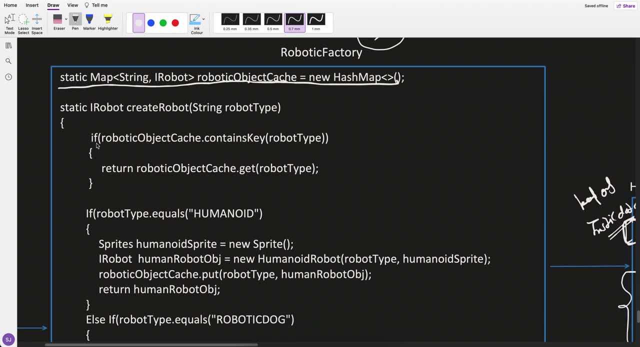 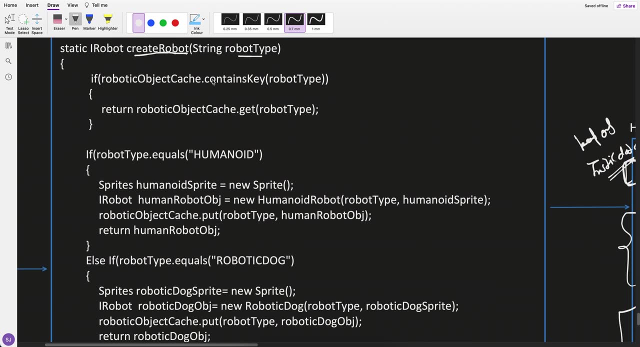 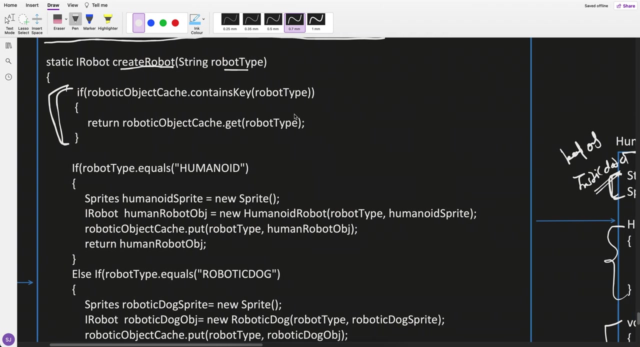 Now, What I Have Done Is I Have Created One, Let's Say, Hash Map, Kind Of A Cache, So I Will Store It, Okay, So? 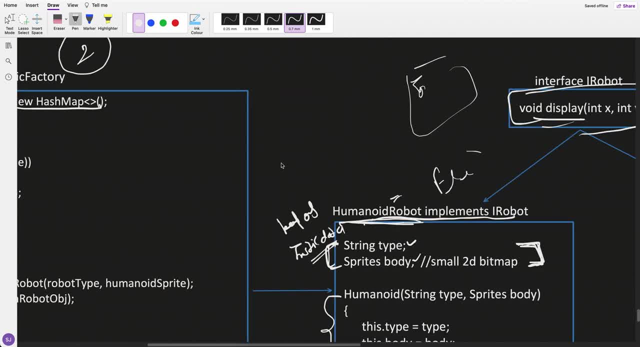 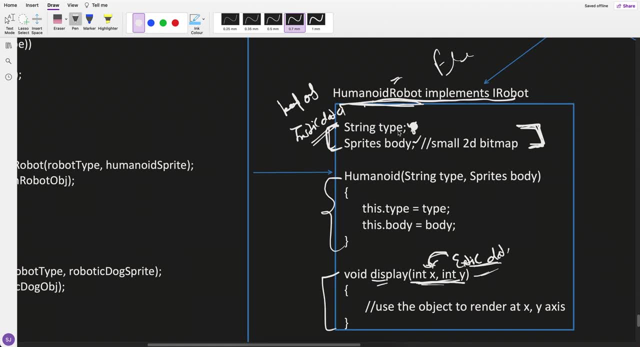 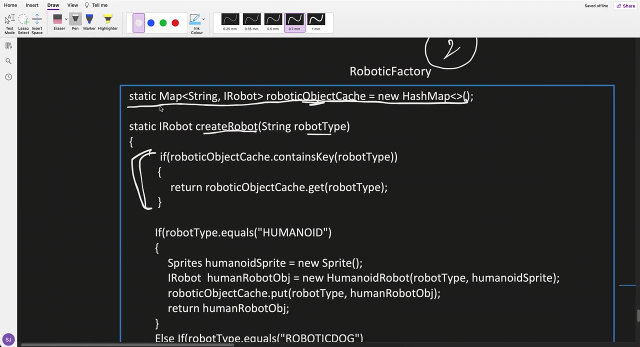 Here I Have A Robot Type, So I Am Distinguishing This Cache On The Basis Of Type. Okay, Humanite Or Robotic Dog, Two Types. 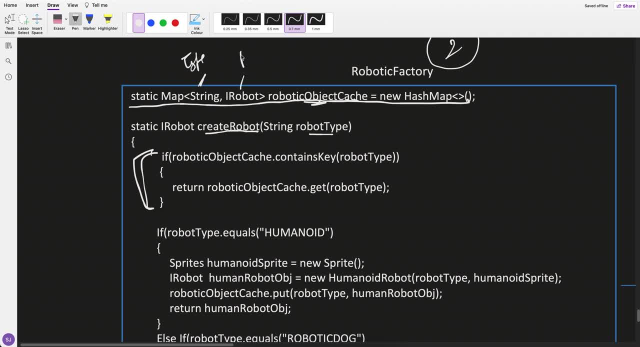 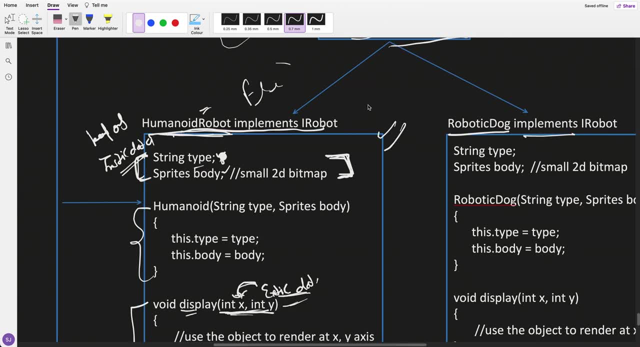 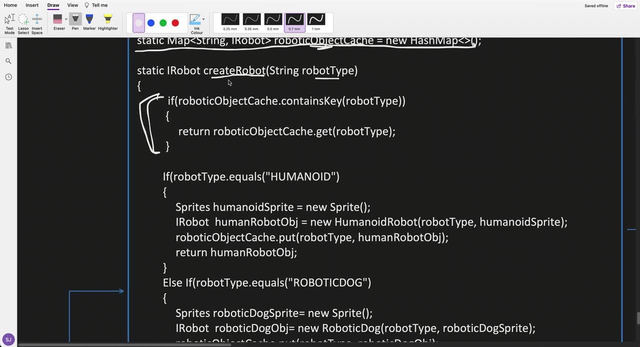 Of Robots Are Exist Right, Humanite Or Robotic. This Is Something Which Is Very, Very Expensive To Construct- Sprite, Okay. So First, Whenever The 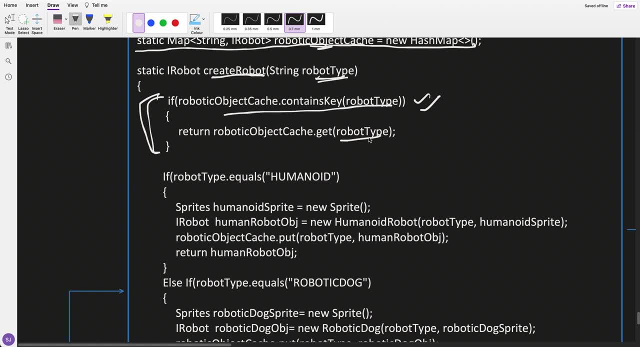 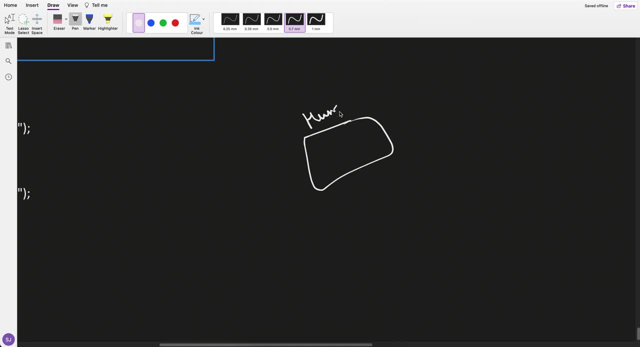 Create Object. Request Comes In Based On The Robot Type, I Will First Have Put Into The Cache, Right. So This Is An Object Of Humanite. 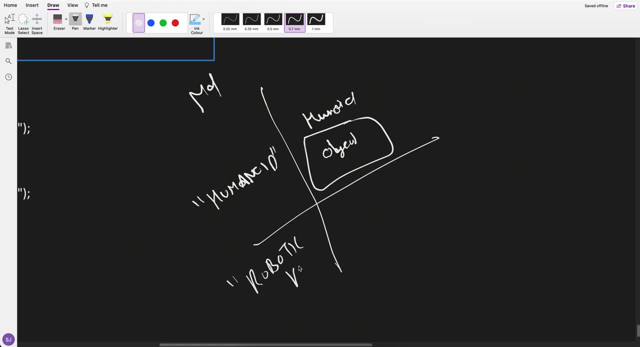 And Map Then. So This Keyword Is, Let's Say, Type, Is Humanite, And Let's Say This, Already Exists? If Yes, Return The Same Object. 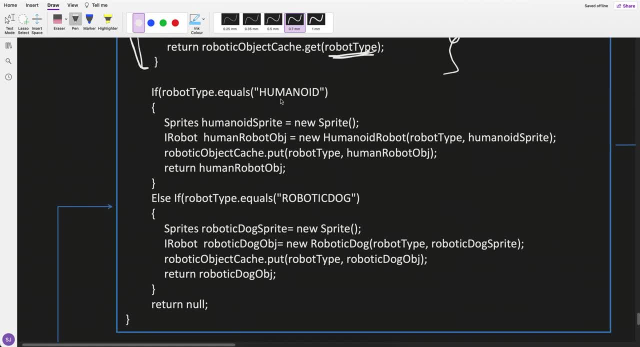 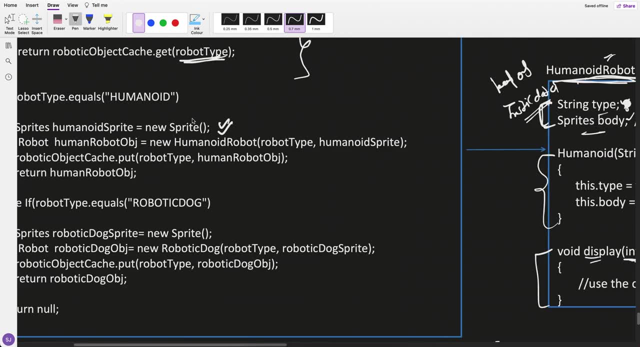 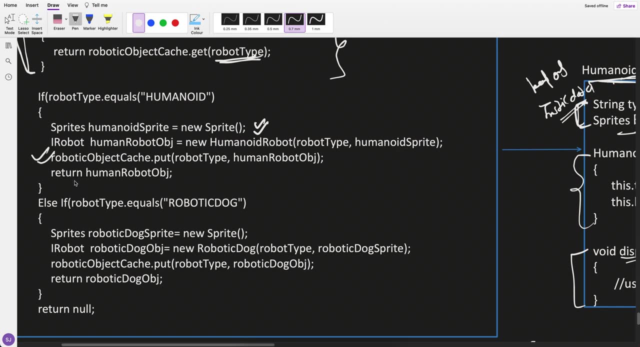 So Now We Are Reusing The Object, Okay, But Let's Say, If The Cache Is Empty, Right, So We What? We Are Caching It. 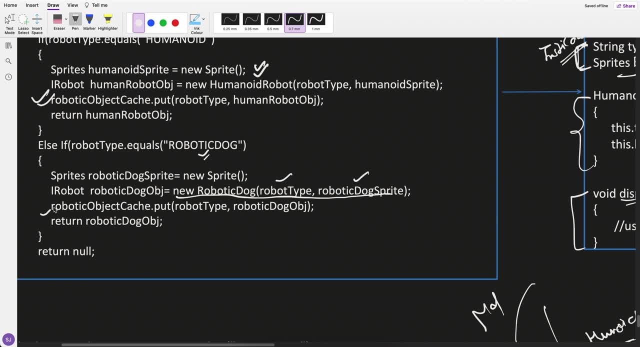 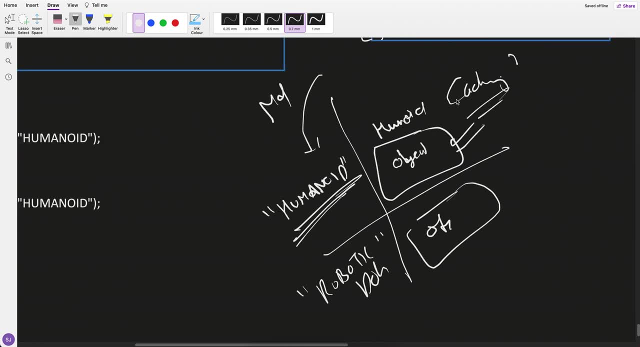 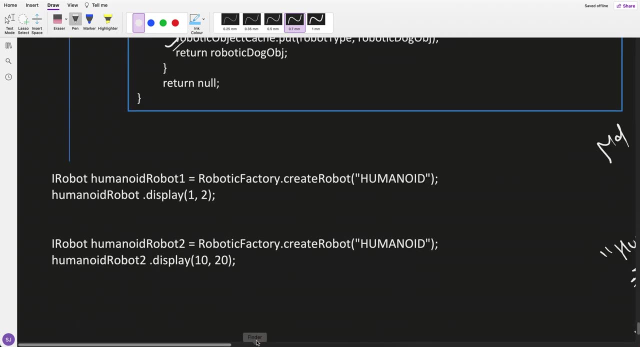 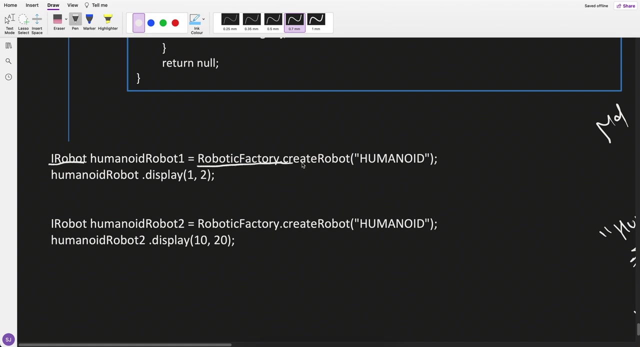 Okay, So Only One Time We Should Be Having It And We Should Reuse It Whenever It Is Required. Now- See In The Client Side. 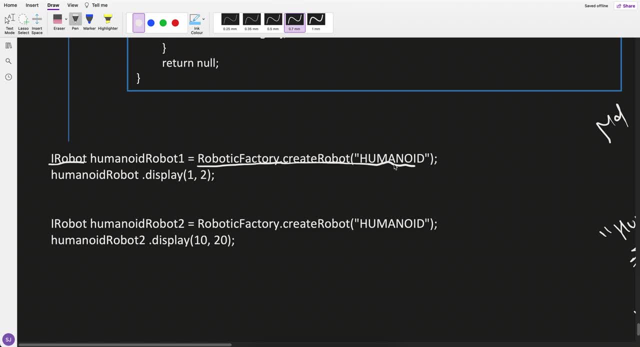 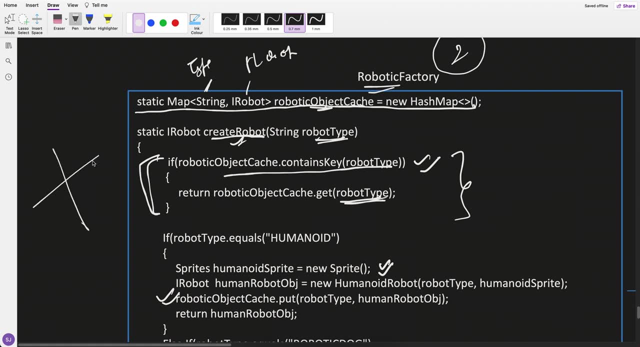 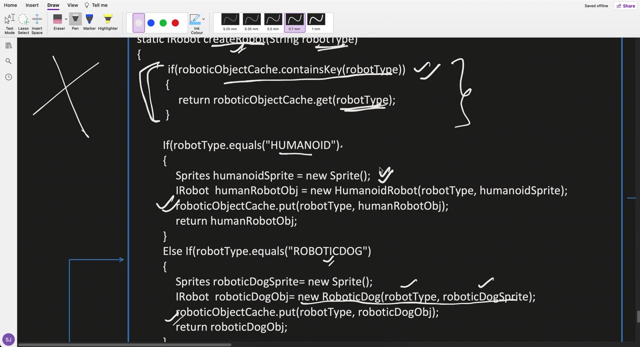 How We Are Giving A Command: Say Robot Factory, Create A Robot Human I. Robot Factory. It Will Create, Create Robot Human I. So Initially It